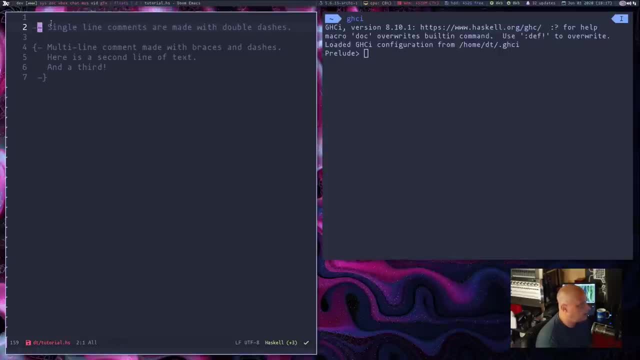 comments are made with Double dashes, So two dashes comment out a line. If you'd want to do a multi-line comment, how you do that is you start it with a brace dash and then, when you're done, end it with a dash brace. 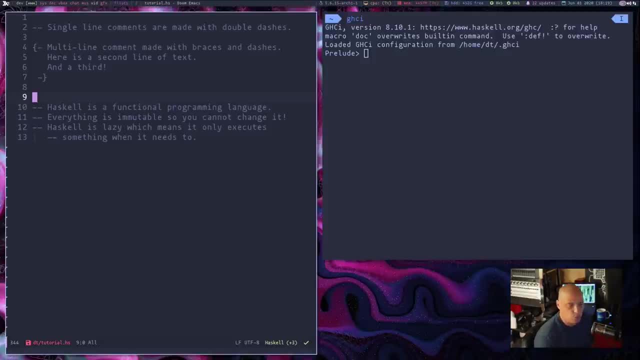 Now let's discuss a little more about Haskell, some things you need to know about before you get started. Haskell is a functional programming language. You're creating all these functions and these functions can be passed as parameters to other functions- Functions inside of functions, right? 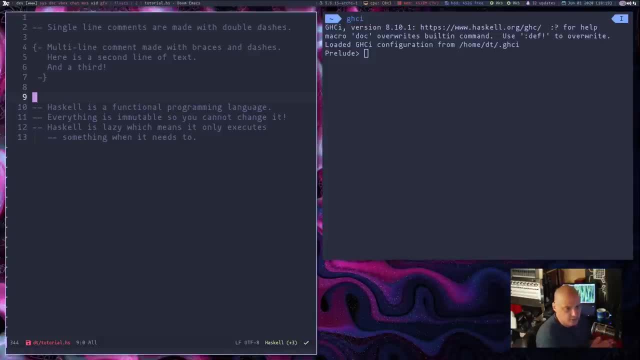 Everything is Mutable in Haskell, meaning you set a value, you can't change it. You set a value, it's that value forever. there's no going back. And lastly, you need to know that Haskell is a lazy language, meaning it's only going to execute something when it absolutely needs it. 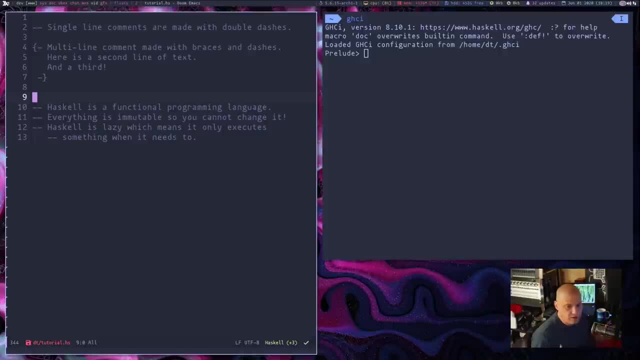 So you don't have to worry about writing this massive program with all these functions and worried about your program being bogged down or slow or anything like that, because it only evaluates something if it really needs it. And for those of you who don't know Haskell, it's a lazy language. 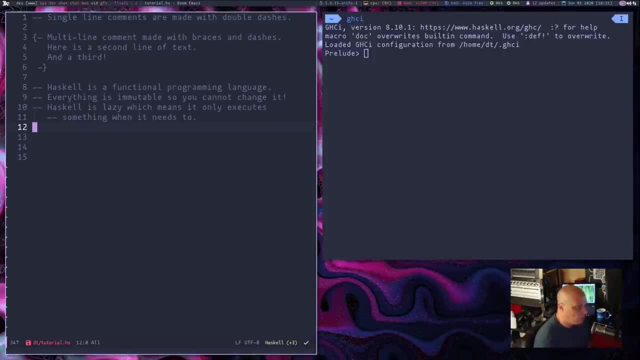 And for those of you that are going to want to dive a little deeper into Haskell, more so than what I'm going to do on today's video, I will leave you some links to some documentation. Some of the best documentation around actually is this book here. Learn You a Haskell for Great Good. 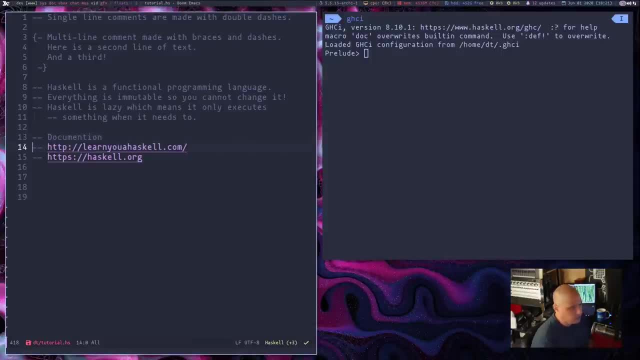 It has a website. you can download the PDF and it's a fantastic read. It's a very good introduction into Haskell. Of course, you can also go to the official Haskell documentation over at Haskellorg. So let's write a little. 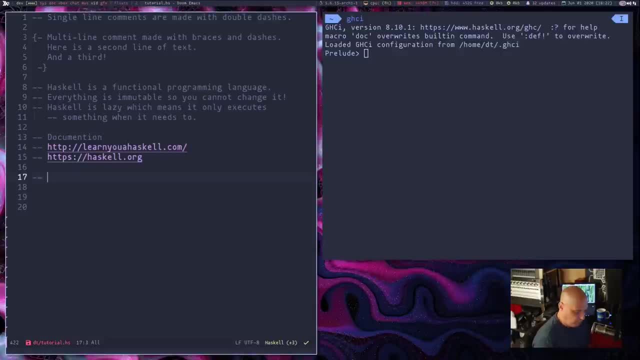 So the very first thing you want to do in Haskell is you probably need to import some libraries. So you're going to create all these functions later and these functions are going to have these commands in them, But those commands are not going to work until you import the specific modules needed for those commands to work. 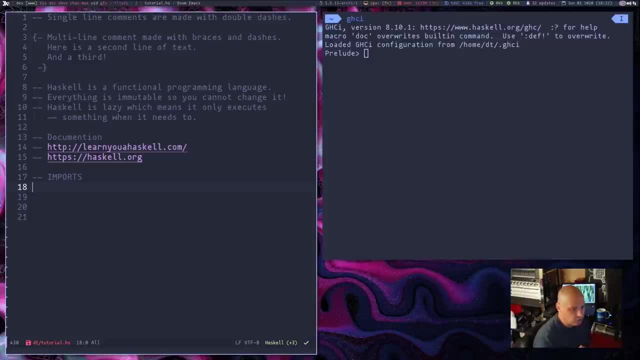 So today, most of what I'm going to do on video is going to involve lists. So, because we're going to really work with lists today, I'm going to import datalist and that will cover most of the stuff that I'm going to put in this document today. 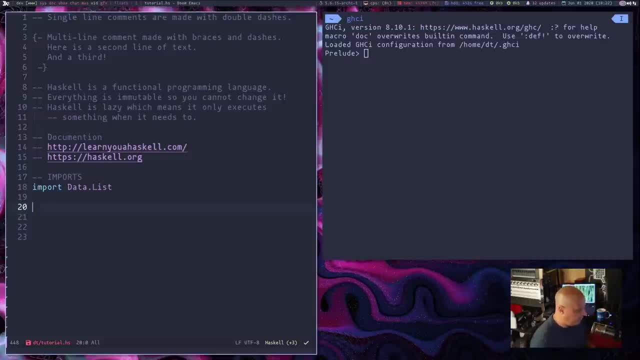 I may have to come back and import other stuff We'll see. Now let's talk about types. Everything has a type in Haskell. And what are these types? Well, they can be a variety of things. Some common types that we're going to play with are bool, which is basically a true or false. 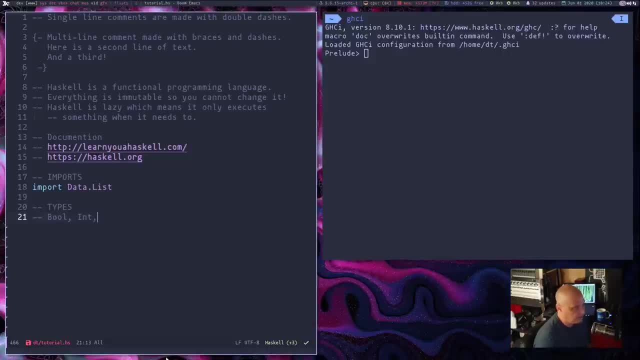 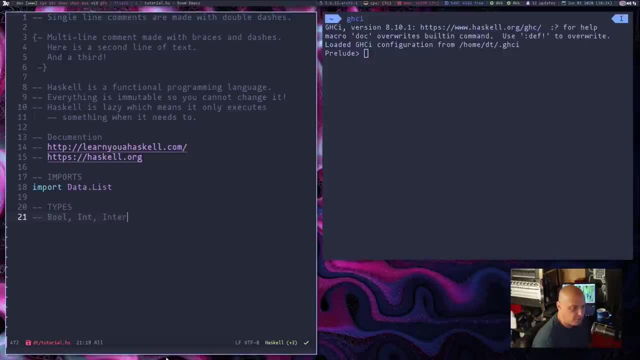 It's a very big number, but it does have a limit. Another type is integer, which is a unbounded whole number. It can be as big as anything. right, That number can be as big as your computer can handle. Another type is float, which is a floating point number. 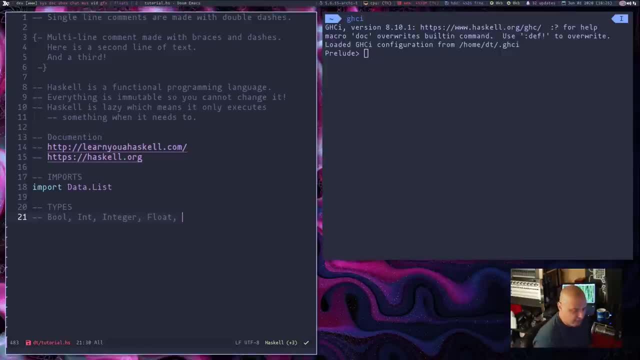 That is a single precision floating point number. If you want more accuracy, you want to use double, which is a double precision floating point number. Also, you have characters, Characters are a type C-H-A-R and basically when we start talking about strings, so you 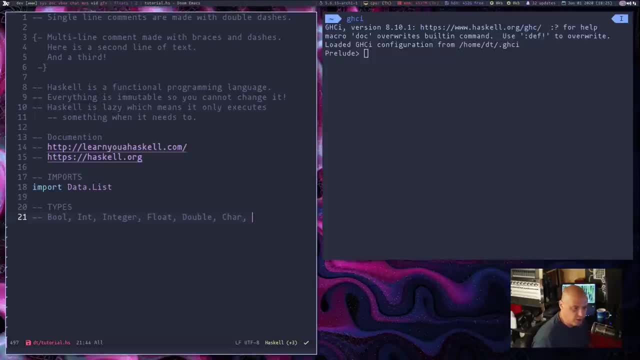 type a sentence, it's really a string. but a string in Haskell is really a list which is designated by the square brackets and then the character type within the square brackets. so a string is basically a list of characters. I hope that makes sense. 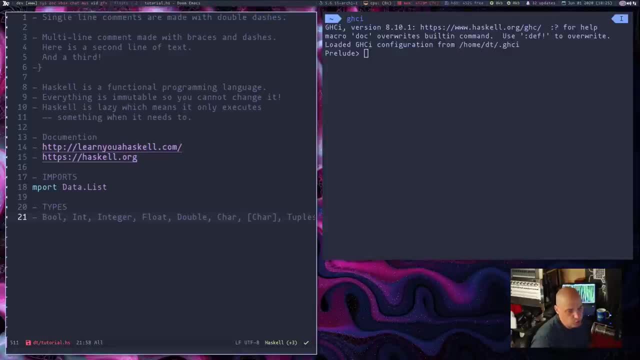 And we're also going to very briefly talk about tuples later. A tuple is basically a list, but unlike A typical list, which is the square bracket list, your normal list in Haskell can only contain like items. So you can have a list of integers, but you can't have a list of integers and characters. 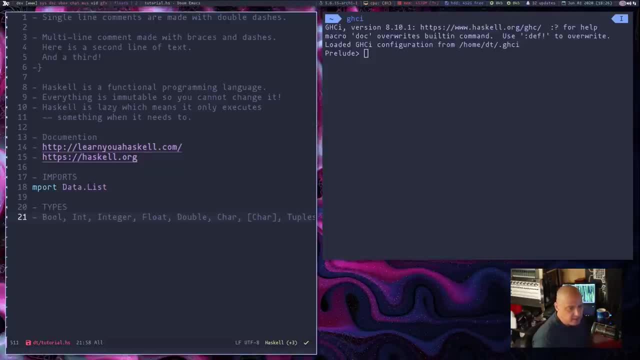 Hope that makes sense. Where a tuple can have a list is basically a list of items that don't necessarily have to be of the same type. Where lists are designated by the square brackets surrounding the items. a tuple uses parentheses, So a tuple. 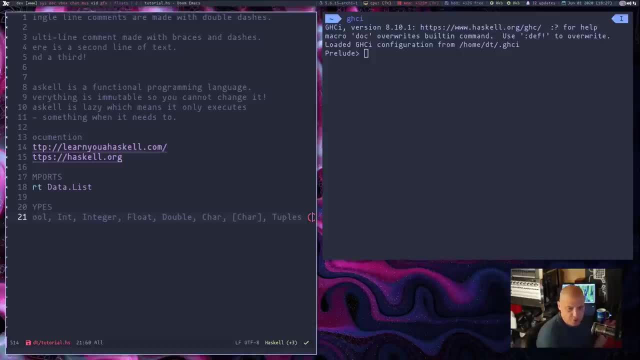 A tuple would basically be a list of stuff, but it will have a parentheses around it. That's how you know the difference between the list and the tuple. So let's talk about the Boolean type. So Boolean is basically asking: is something true or false? 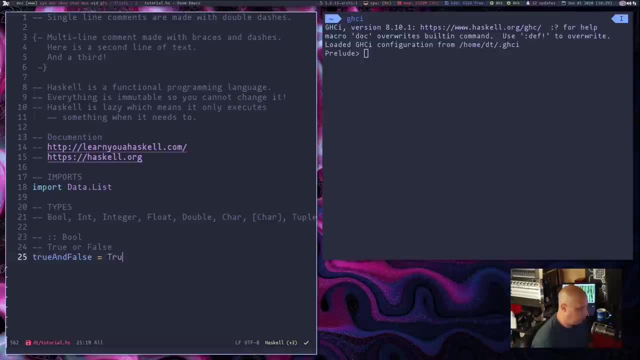 So if I did true and false equals true and and false, and let me write that I'm going to go over to the terminal window here in GHCI and I'm going to do colon L, because we haven't Loaded this tutorialhs file into GHCI. 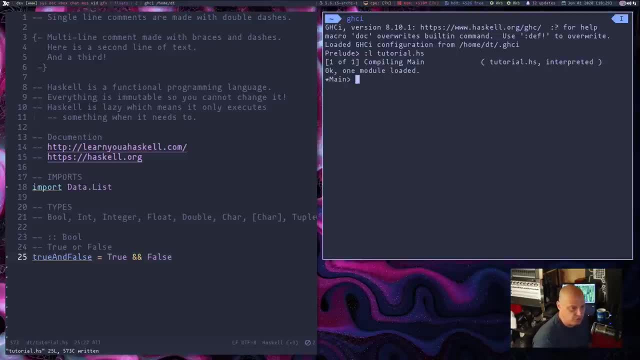 So colon L and then the name of the file. It compiles just fine, meaning there's no errors. And now I should be able to run true and false, And it returns false, as you would expect. And I said a couple of more things here. 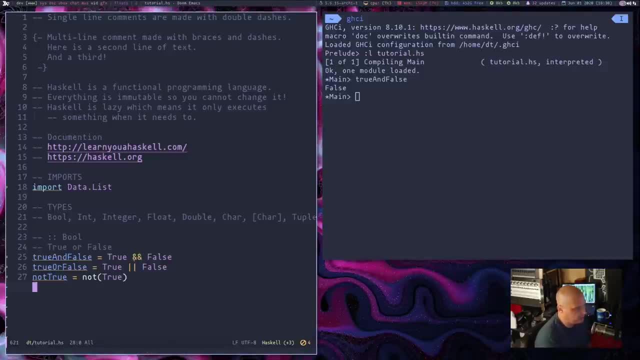 I did a true or false. You can see it's exactly the same as true and false itself. So the two ampersands, it's the two pipe symbols. And if I reload this here into GHCI, Which is colon R for reload, and then did a true this time or false, you see, this time I get true. 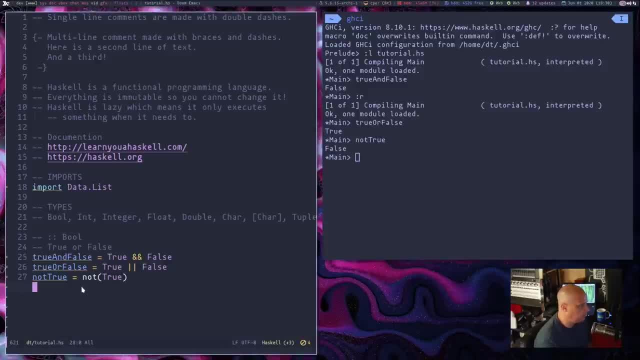 And if I do a not true, I get false, because not true equals the command not, And then in parentheses I put the word true. So if it's not true then obviously it has to be false. Hope all that makes sense. 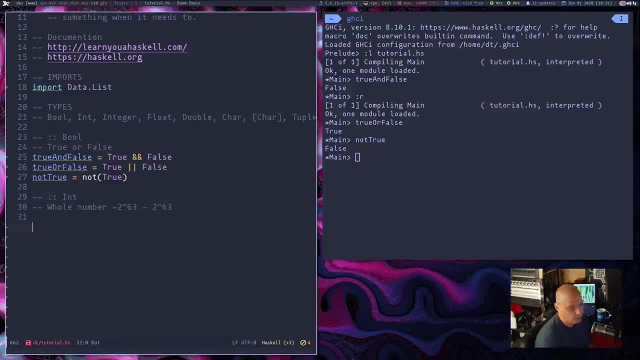 The next type we should talk about is int- I-N-T, So those are whole numbers. They do have a limit And if you want to see what the maximum size number is, we could do a max int. that's going to be the name of this variable here. 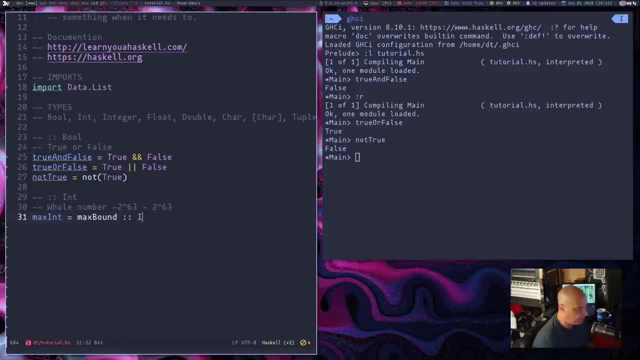 And it's going to equal this command, max bound, two colons I-N-T for int, And let's write that, And then I'm going to go over to the terminal and let's reload, And then I'm going to run max int. 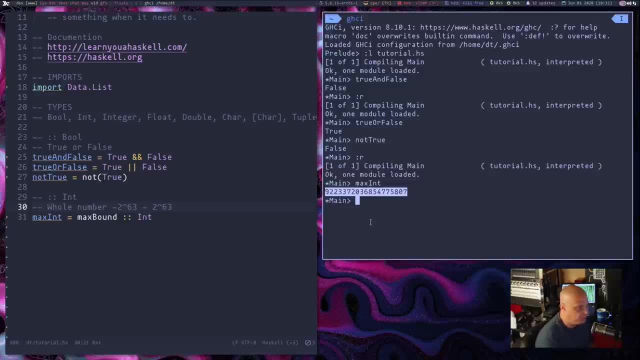 And you can see that is the biggest int that you can use. If you wanted to see the smallest int you could use, you could do min bound colon, colon I-N-T and that is the smallest int you could use. And remember that the main type that you want to use is probably integer rather than int. 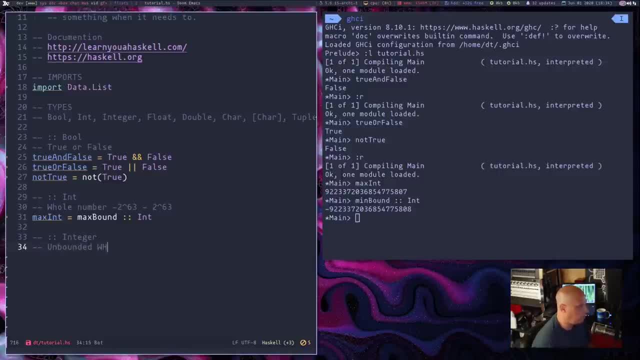 Integer, of course, is an unmounted whole number, So let's play with this a minute. So if you wanted to go ahead and create something here, so let's do. num five equals five. Now the Haskell compiler is smart enough to know that is an integer. 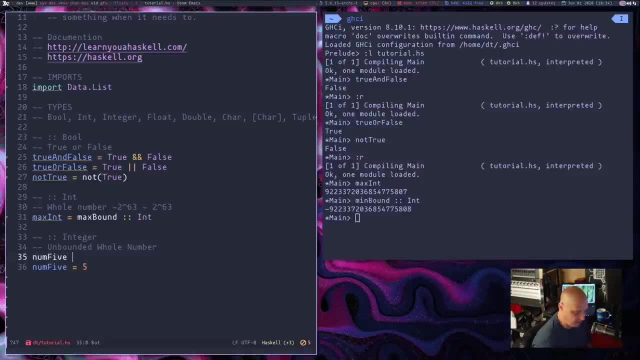 But typically in Haskell, good practice is to always type this: you know, set a type for it, So I should go up above it and do num five, two colons integer. Now I don't actually have to do that, because if I comment this line out, let me write and save. 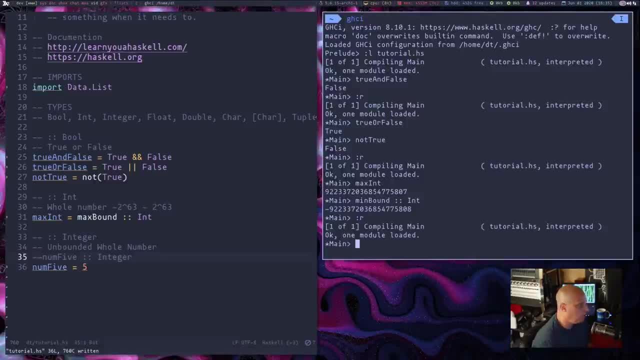 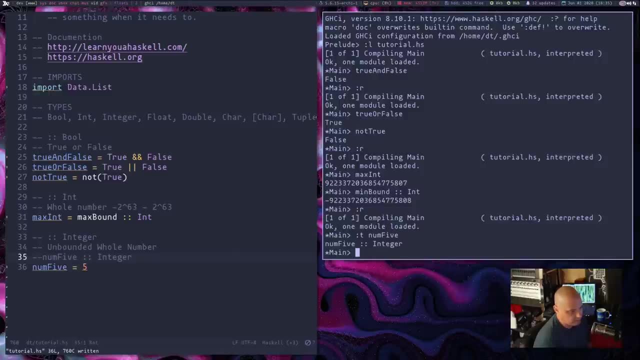 And then let me go and reload over in the terminal here And I do a colon T to get the type of num five. You see it says num five, colon colon integer. It already, It already knows, just because five was the value I set. 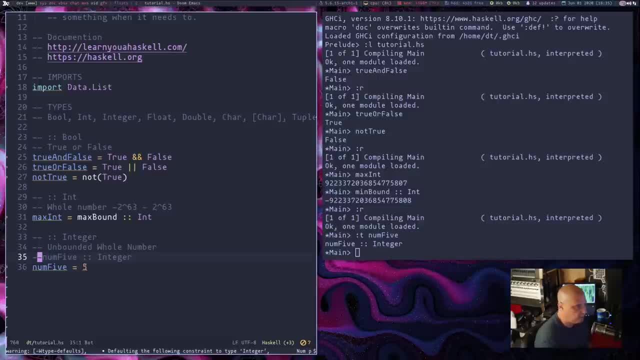 Five is an integer. It doesn't need me to tell it it's an integer. You know, Haskell is pretty smart. It can infer what the type of something is, usually by whatever you stored. you know as far as the value of that expression. 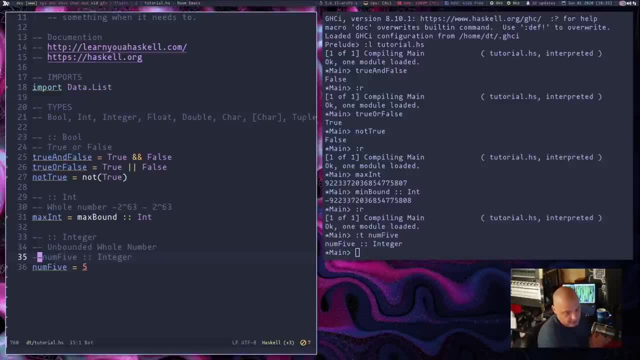 But although it can do that most of the time, sometimes you really do need to specify a type And for purposes of just you know this video, I will go ahead and leave that. It does no harm to go ahead and set the type. 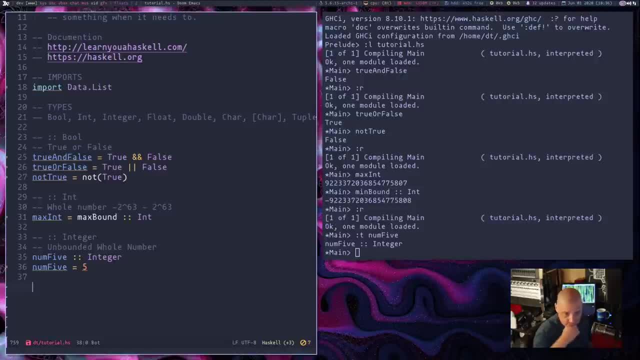 Now what if I, Instead of integer, I wanted to use the floating point number? Well, I could do another variable here. I could do num five, and then I'm going to do a single quote at the end. Basically, that is often used when people do Haskell programming is they create two very similar variables. 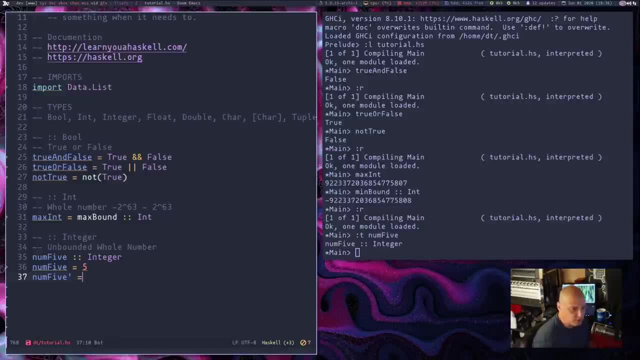 They'll do name of variable and then they'll do name of variable and then one single quote at the end, to let you know, is basically the same variable, Just a minor difference. this time I'm going to set this to five dot zero, And then I need to. 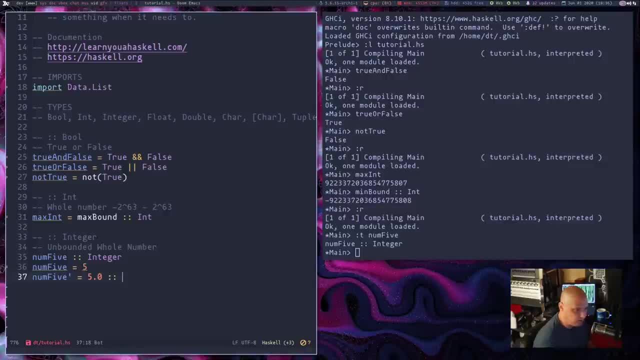 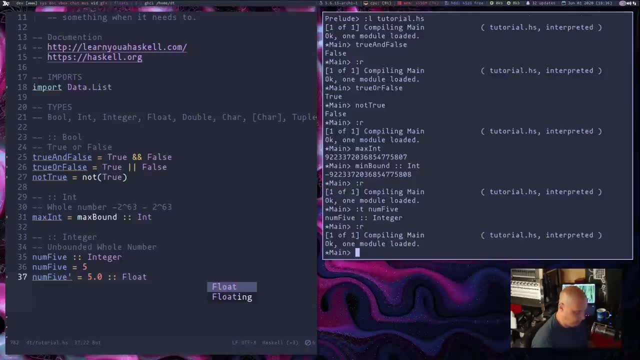 Specify that this is a floating type. I could just do the two colons at the end of the line here and do float right there and then get over into the terminal. Let's reload and then run num five. Actually, did I already run it before? 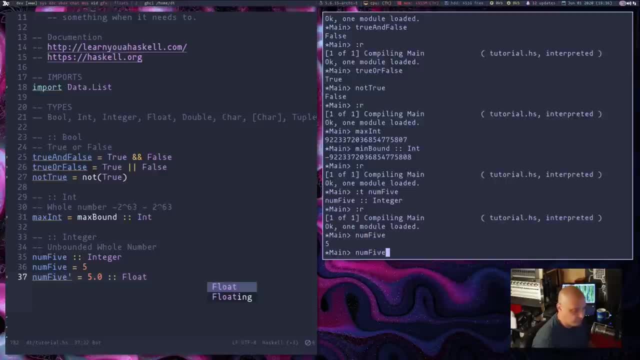 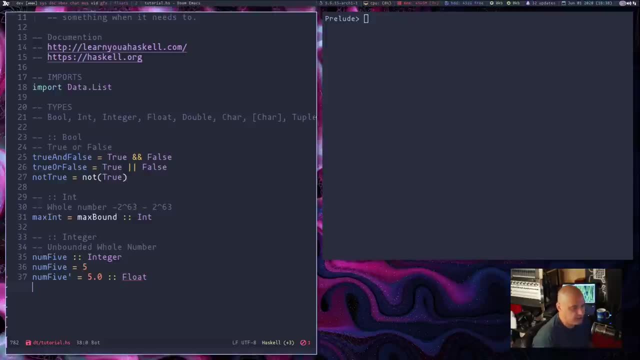 No, I didn't. Let's run the first num five, which is just five, and then num five with the single quote behind it returns five dot zero. And if you want to see how good Haskell is at inferring the type you already saw, it can pretty much figure out whether something's an integer or 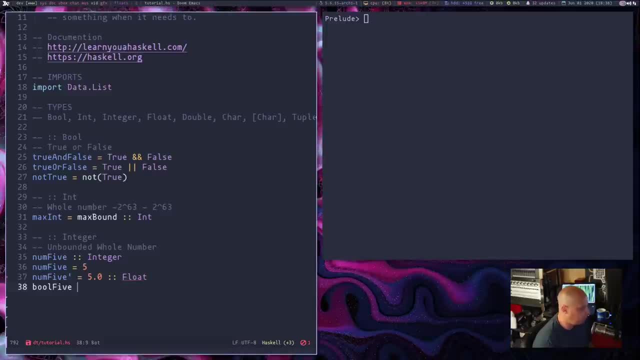 Float. How does it handle boolean? Well, let's put it to the test. If I do bool five here, I'm going to call it boolean five. and equals five is greater than four. Let's write that. Get back to the terminal. 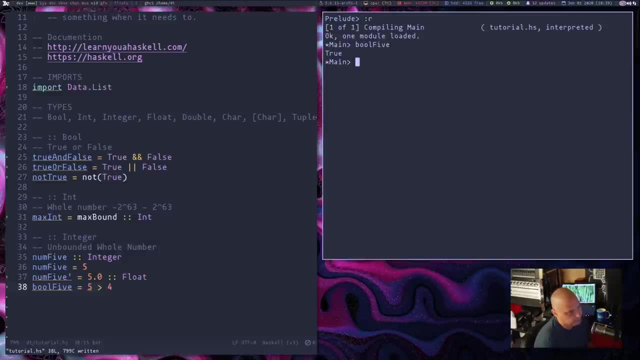 I'm going to do a colon R and then if I do bool five, it returns true because of course five is greater than four. But if instead I did a five is less than four, save that and reload over here in the terminal again and bool five. 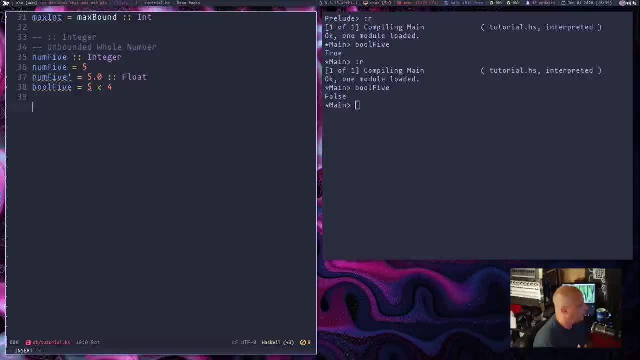 Now is false. Let's talk about floating point numbers and doubles. Typically, you're going to use doubles for everything. You're usually not going to bother with float, which is the single precision floating point number. but you could, but you probably need to specify that it's a float. 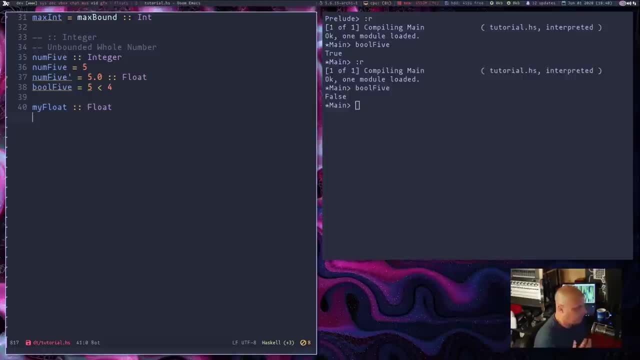 Otherwise, you know, Haskell may decide it's a double. This is kind of tends to default to doubles anyway if it has to infer, you know, whether it's a single precision or a double precision floating point number. So we're going to set the type and I'll just do my float. 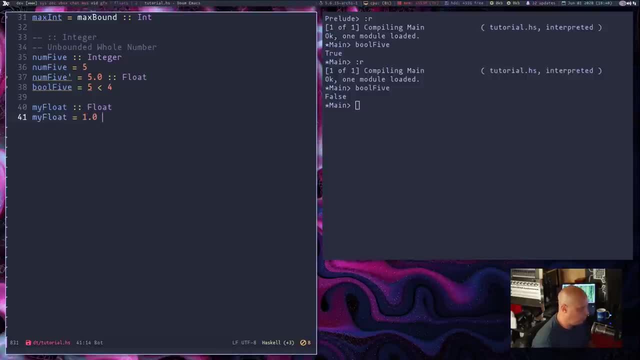 Equals and then it needs to be, of course, point numbers. I'll do one point zero plus two point five. Let me write that and get back into the terminal, Let's go ahead and reload that and let's run my float and then you see it returns three point five. 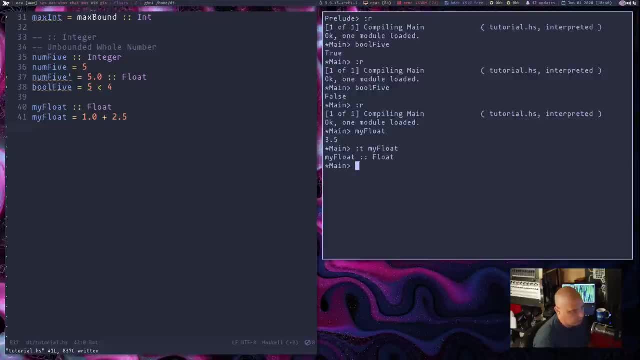 If I ran a type on it. we specified it in the document that it was a float. But what happens if I comment this line out and then get back into the terminal Reload, And this time when I type my float, you can see that the compiler would rather that be a double. 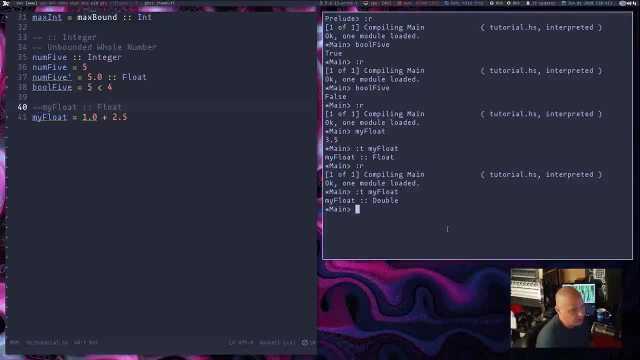 You know it defaults to calling pretty much every floating point number a double rather than just a float. And let's talk about the double floating point numbers and how precise there are. They're precise up to 11 points, so it has 11 point precision. 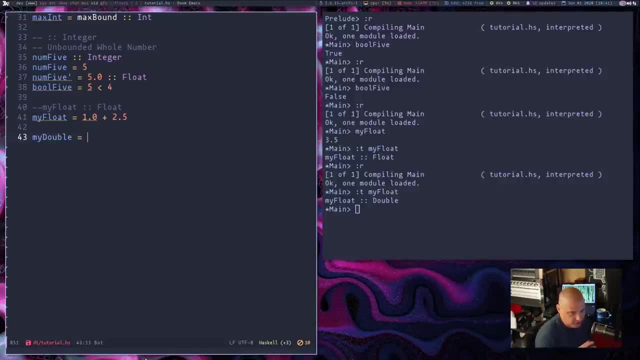 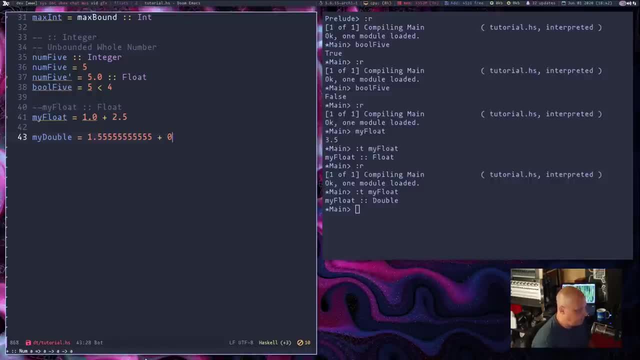 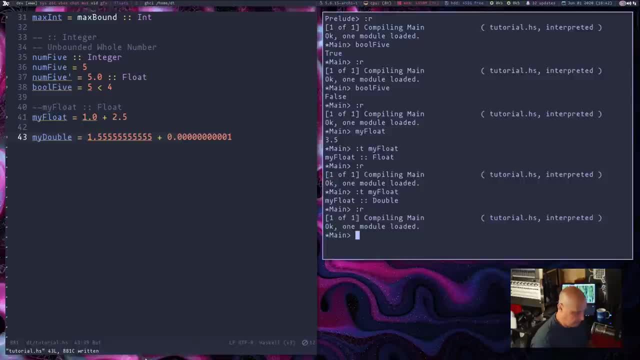 Let's write that and get back into the terminal reload and let's run my double And, as you can see, we get the correct answer returned here. The next type we should talk about is characters- Single Unicode characters denoted by single quotes. 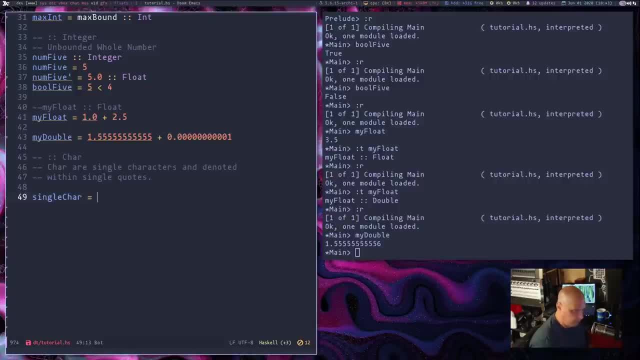 So if I did a single character equals and we'll just use the character A here and let me reload and do single character, you see it returns a, again within single quotes because that's denoting a character and strings within Haskell are just lists of characters. 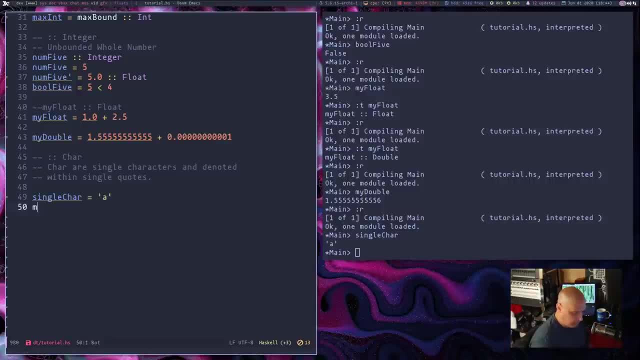 So if typically you know you set a variable for something- for example I could set a variable for My name- my name equals Derek And if I write that and get back into the terminal, reload and run my name, you see it returns Derek. 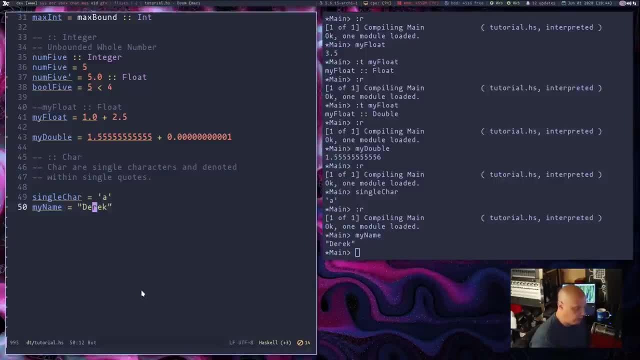 What that is. it's really just a list of single characters. So I'm going to write my name and then a single quotes- because we're just writing the same thing, basically just a different way- and then a list of characters. So a list of anything is typically is in brackets, and then it has to be separated by commas. 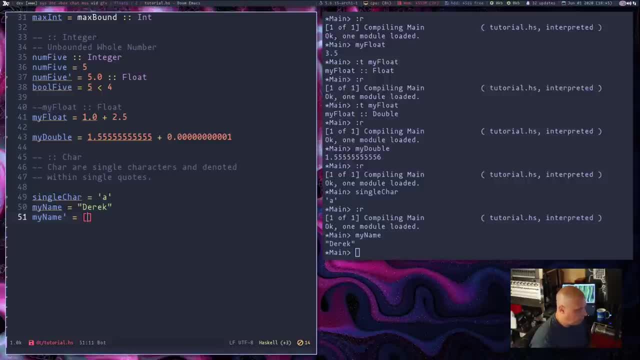 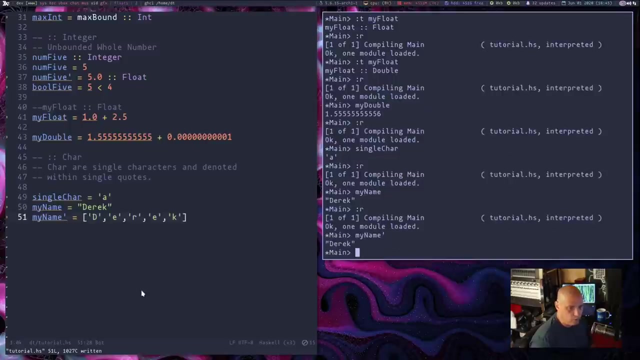 But remember, characters have to be denoted with single quotes. So this capital D actually has to be inside single quotes. and the same thing with the next character there. Let me write that and let's reload in the terminal here. And this time, if I do my name with the single quote at the end, you see it returns Derek. 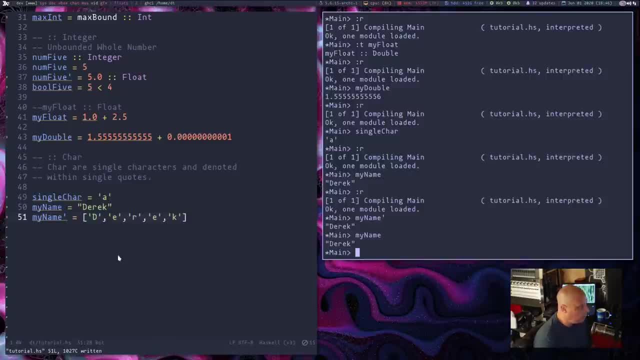 But my name, without the single quote, is also Derek, So this and this are the exact same thing. It's just two different ways to write it. And remember a string. If we had to Type my name, my name is going to be a list of characters. 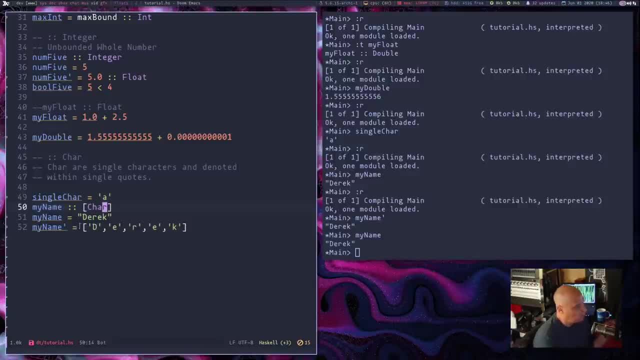 That would be the type, But again, you don't have to specify this. when you do a simple variable like my name equals, and then, in double quotes, you know a word or a sentence or something. It knows. that's a string Haskell knows. it's basically a list of characters. 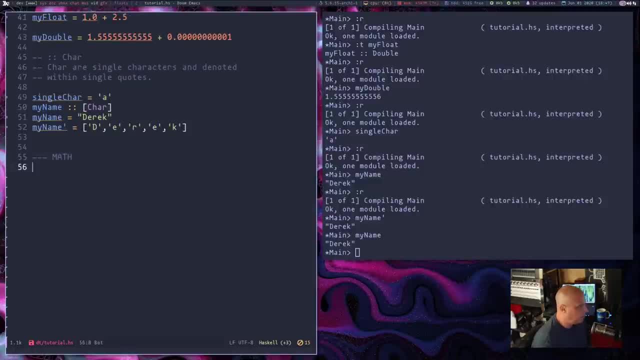 You don't have to specify it. So let's talk about some basic math operations here in Haskell. So you're going to do add num, add num. I'm going to do Three plus six. Go back to the terminal Reload. 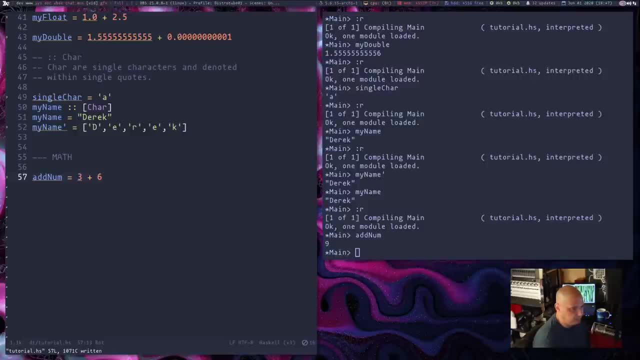 I'm going to run add num and you see I get the value nine returned. And if I wanted to, I could do the same thing with subtract, multiply, divide And you can see. it's just your standard math operations. You wanted modulus. 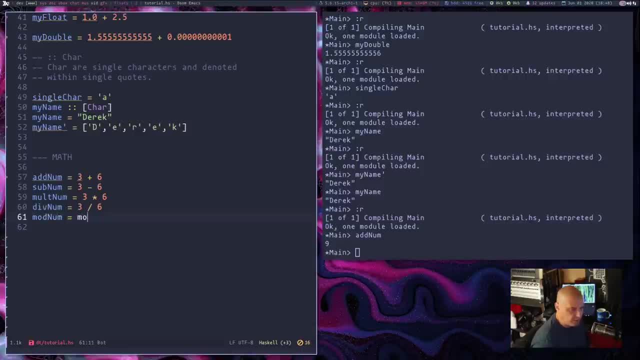 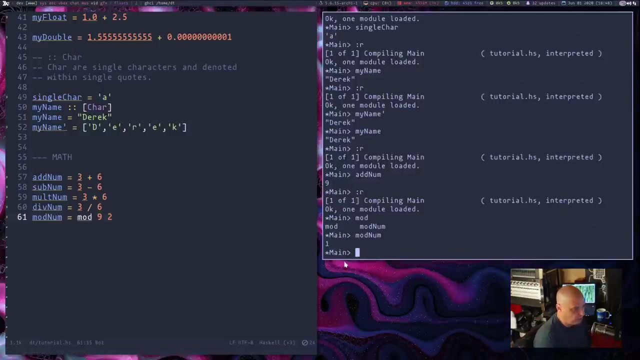 I could do mod num equals and then this command here, mod Take the modulus of, I'm going to do nine divided by two. That's right, That get to the terminal Reload. And if I ran mod num, you see I get one, because that is the modulus, the remainder of nine divided by two. 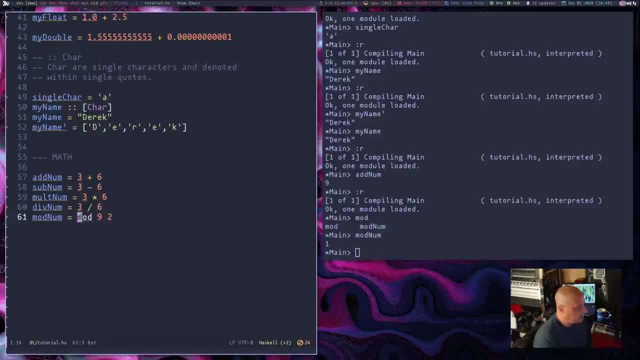 Now I could have wrote that a different way. You see mod here, this command mod. That is what we call a prefix operator. It's prefix meaning it's at the beginning right. But if I wanted to, I could have wrote this slightly differently. 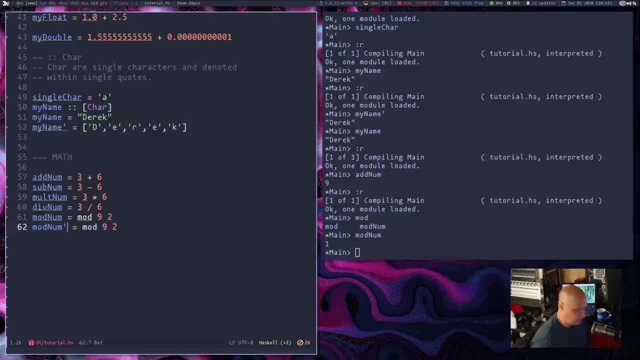 I'm going to set this to be mod num and then I'll do the single quote Behind it. I'm going to do nine And then in backticks- this is very important, You got to use backticks mod two And a lot of people like using it in this layout where, instead of using mod as a prefix operator, they like using it as a infix operator, meaning in the middle, because it makes more sense, I guess, visually, because nine divided by two, not nine, mod two. 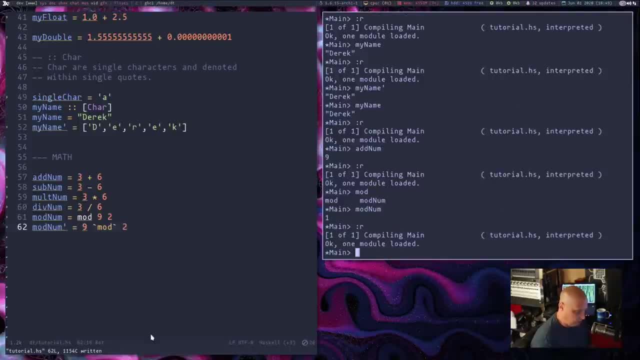 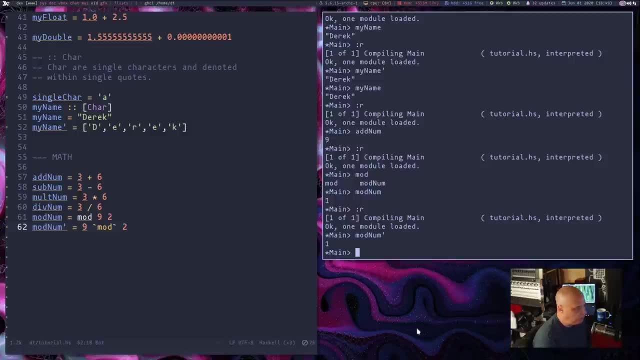 You know. for the remainder, if I go to the terminal and reload and you could see mod num with the single quote In action, here again we get the same thing. how you write it is really up to you, It seems. when I check out other people's codes and examples, most people typically use the infix version of mod. 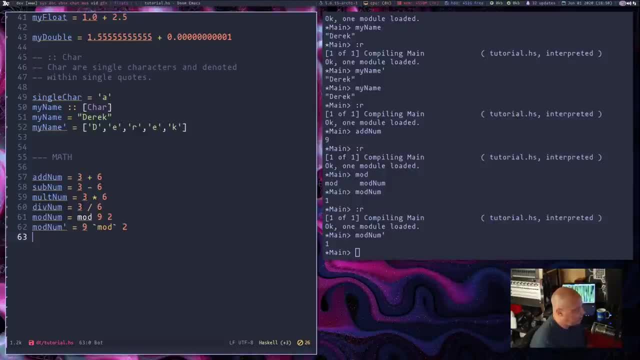 One thing to note when you are doing anything with negative numbers. negative numbers need to be wrapped in parentheses. So if I did add neg equals, and then I'm going to do, we'll do four plus, and then it doesn't really matter what I do. 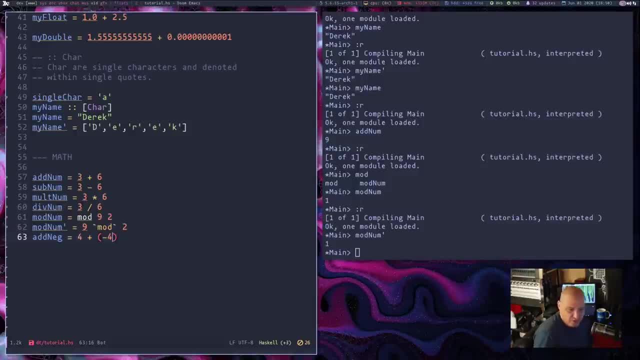 I'm going to do negative four, Even though that's just going to equal zero, But that's how you would have to write that, because if you did not have the parentheses, well, let's just try it, I'm going to write: 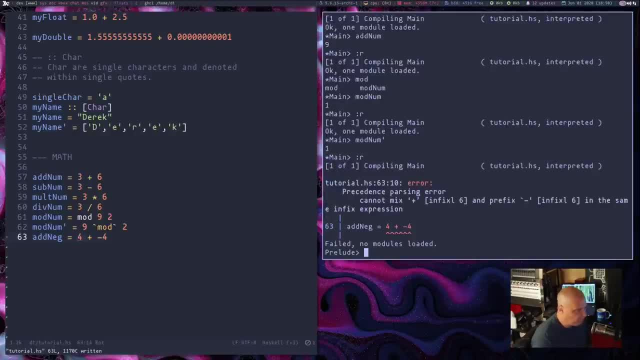 Let's go to the terminal and reload and won't even compile because it doesn't know what to do here. The compiler is confused because you got plus and then the minus. What exactly are we trying to do here? So we've got to go back and wrap that in parentheses. go back and reload this time. 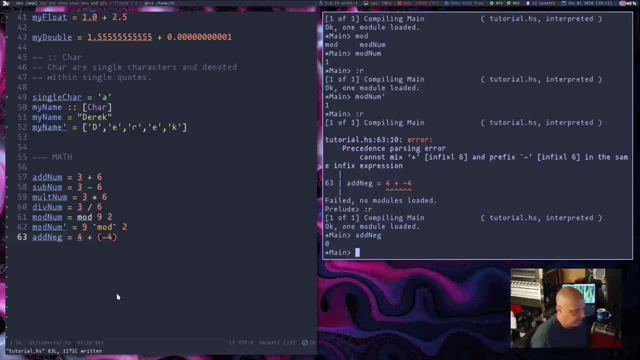 It compiles just fine. And if we ran add neg, We're good, We're good, We get zero return, which is exactly what four plus negative four would be Some other useful math functions that you could use. Of course you can use pi. 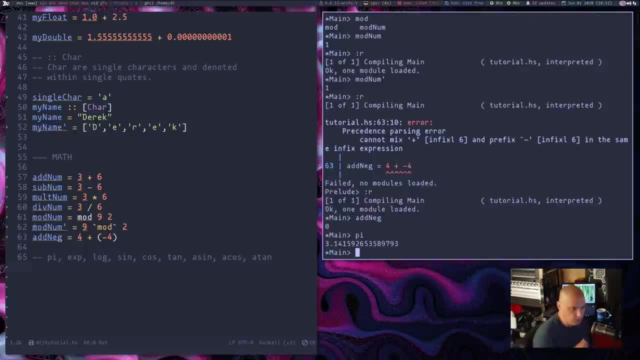 If I go back to GHCI here and I just type pi, for example, it'll tell me exactly what pi is. I think it does it out to 13 digits. I'm not exactly sure. I didn't count it. You get a lot of digits of pi though. 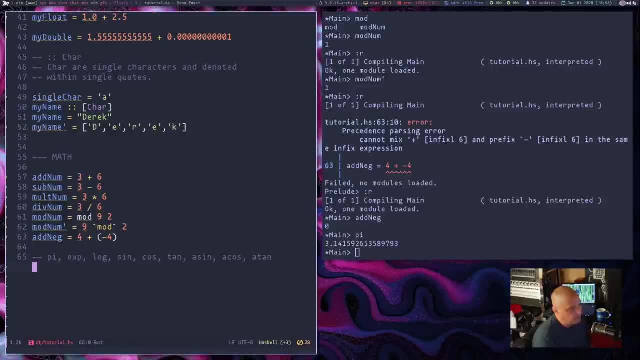 You could also take the exponential of something, the log of something, sine cosine, tangent arc. sine arc, cosine, arc tangent. You can do pretty much anything you want to do with math inside Haskell. We could also truncate a number. 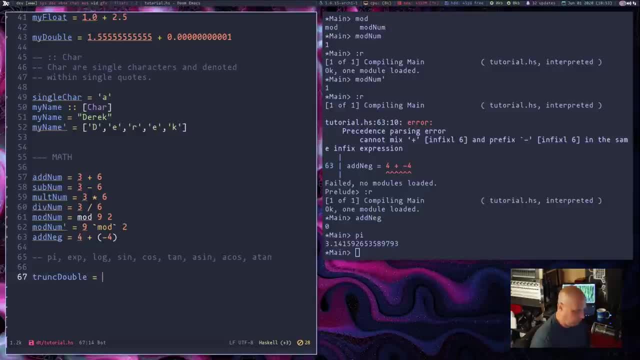 So I'm going to write this function, trunc, double equals, And then we're going to use this command, truncate, And it basically takes a long floating point number and cuts off everything after the dot. right, And you know what? Remember this, that we said earlier: my double. 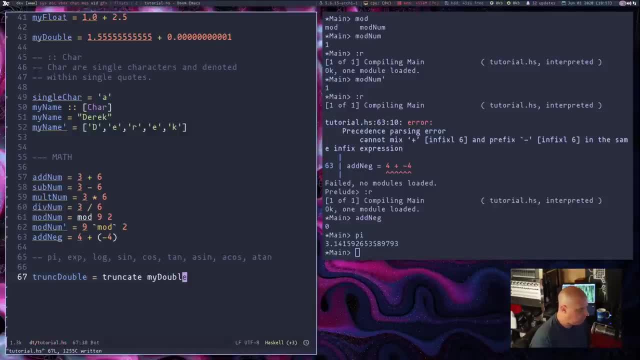 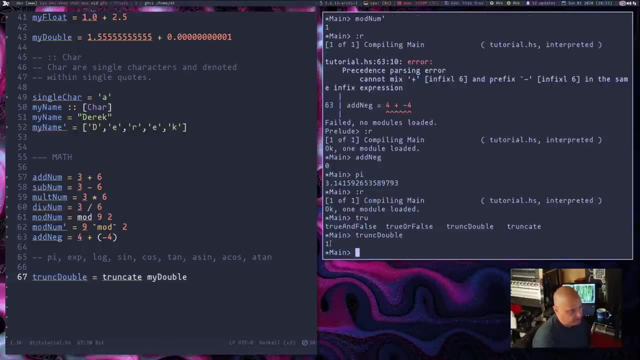 I'm going to truncate my double. Let's run that command, that trunc, double, Double command here, And you see it truncates it down to just a whole number one. And you can also round a number. take the ceiling of a number, take the floor of a number, 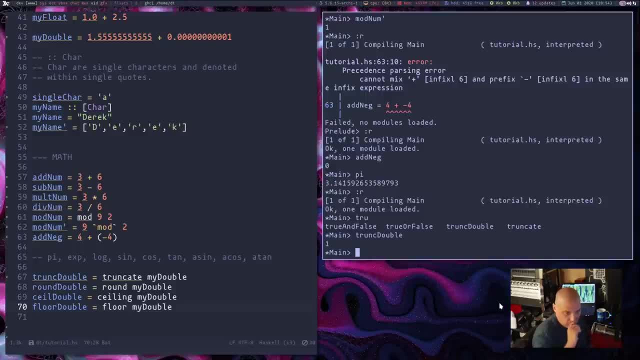 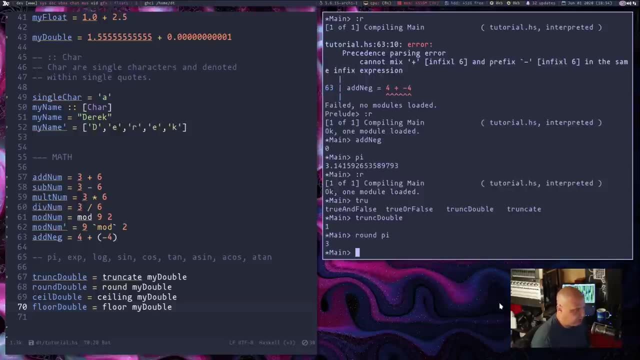 So you know, I could create those functions or I could just go over to the GHCI interactive prompt here And I could do something like: well, I could round pi, which we know it would round it down to three, because pi is 3.14.. 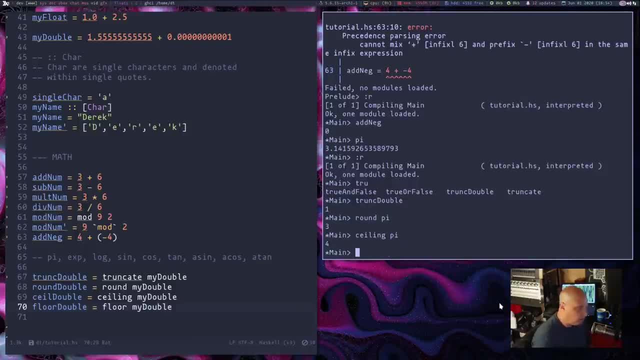 I wanted to take the ceiling of pi, Of course it would return four. Let me clear the screen here inside GHCI. To clear the screen you need to do a colon and then an exclamation point to let GHCI know you're running a built-in shell command here. 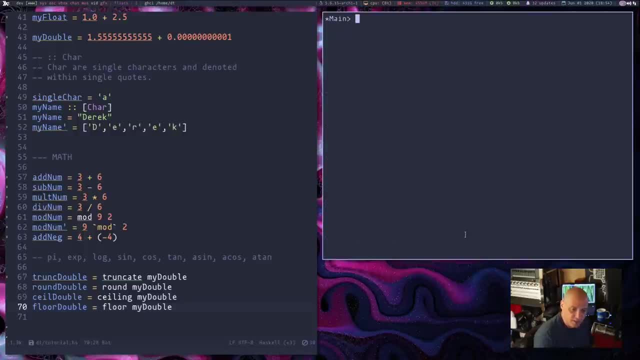 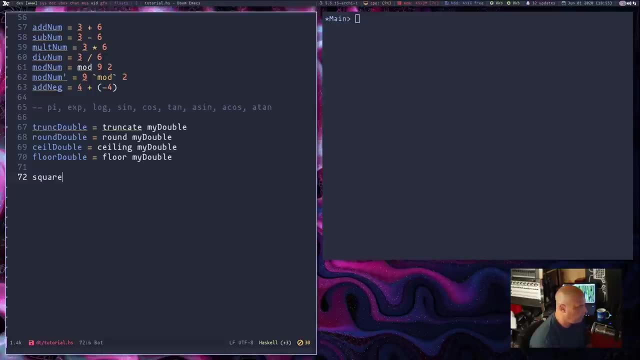 Clear And it will clear the screen. Just typing clear itself in GHCI will do nothing. It will just return an error. Let's play around with some numbers here. Let's take the square root of something I'm going to do. square five equals and this command here, sqrt. 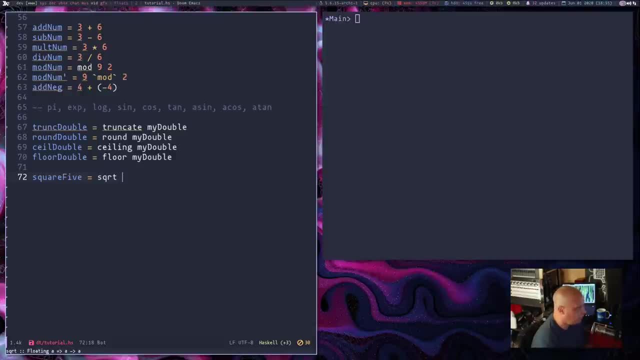 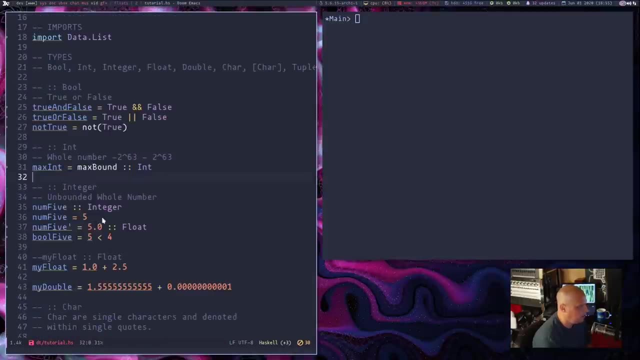 That's going to take the square root, Square root of whatever you pass along to it. You remember the variable I did earlier. Where was it? Num five equals five. Let's take the square root of five. So I'm just going to do num five. 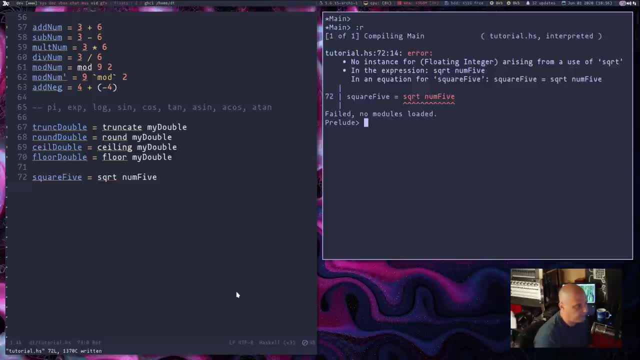 Write that and reload And it's complaining. So when I save this and did a reload, it's saying square five equals square root num five. It doesn't like that And it will actually tell you why it doesn't like that Floating integer. 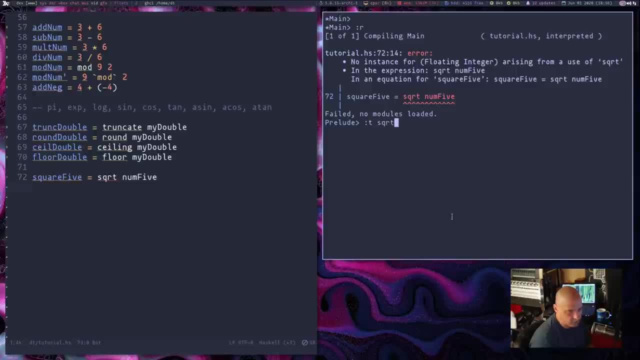 Well, let's run, type on sqrt, Square root And you see the type is it's taking a floating number, A floating of type A, And it's taking A and returning another, A type value. Basically, it's saying it's expecting a floating point number. 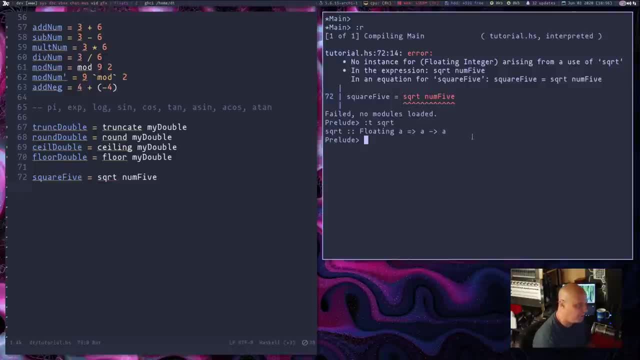 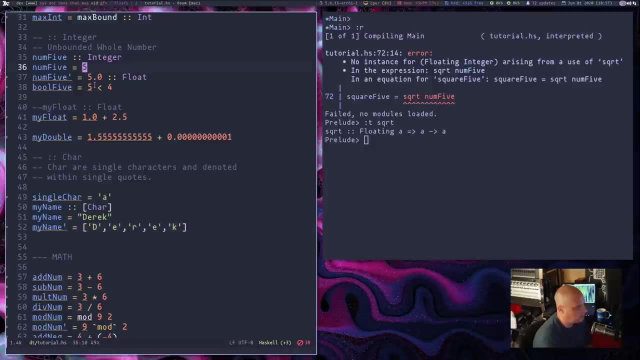 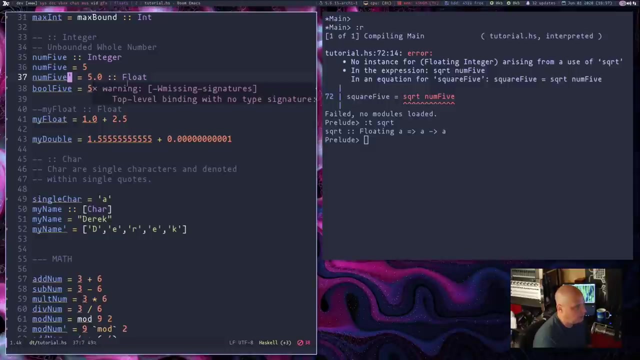 And it's going to return a floating point number when it runs the command. This is not a floating point number, though. Remember num five was just a whole number. right Now, remember this one, Num five, with a single quote. We did 5.0, and then we did the colon, colon float. 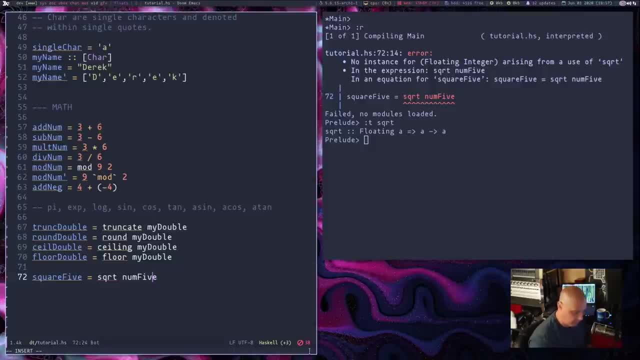 We set that as a floating point number. So if I actually go back here and do sqrt num five, single quote Write And then reload, It compiles just fine. And if I wanted to run this to make sure it actually works, let's do square five. 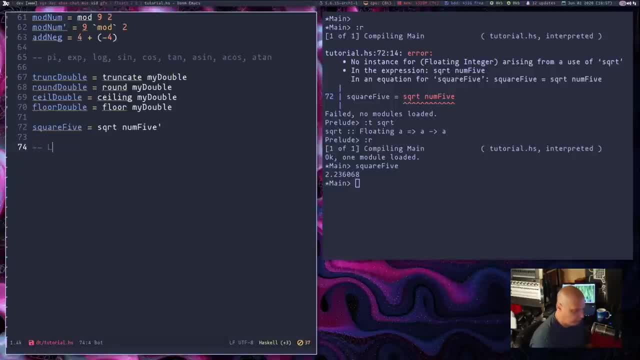 The square root of five is 2.236.. Alright, let's play around with some lists. So I'm going to make a list, I'm going to do this, I'm going to do num. list equals And a list, of course, needs to be in these square brackets. 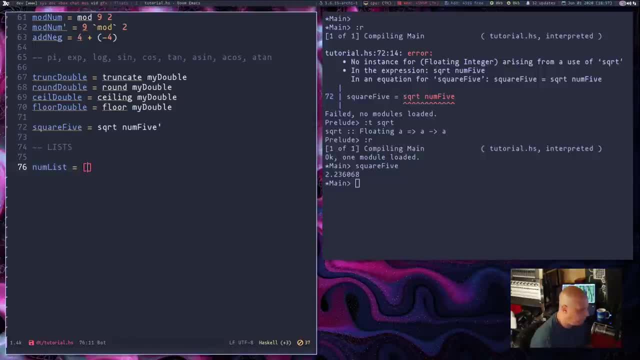 And for numerals you just need to do comma separated values. So I'm going to do one, two, three, four, five. That is a list. If I save that and go back into the terminal Reloaded And I did a num list. 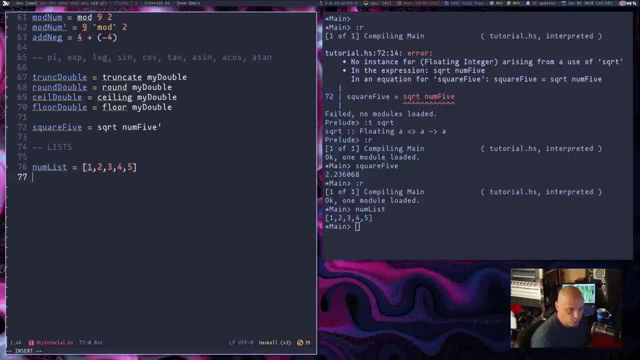 You see, I get that list returned. Now there's an easier way to write that, Especially if you're just doing consecutive numbers. You could do what is called a range, So range list. I'm going to set that to be one and then two periods: dot, dot five. 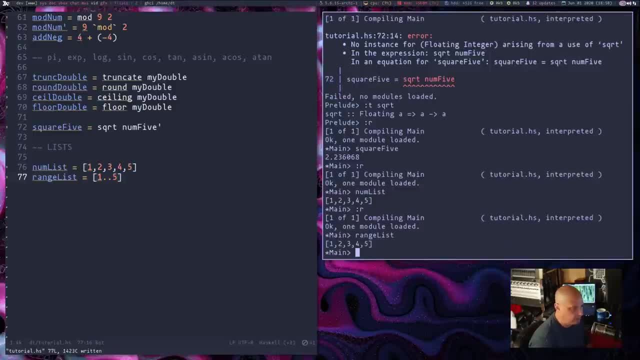 If I reload and do range list Again, I get the same thing as far as output One through five in a list, And it's just a different way to write it. It's a lot easier, though, if you're dealing with more than two or three items of consecutive items. 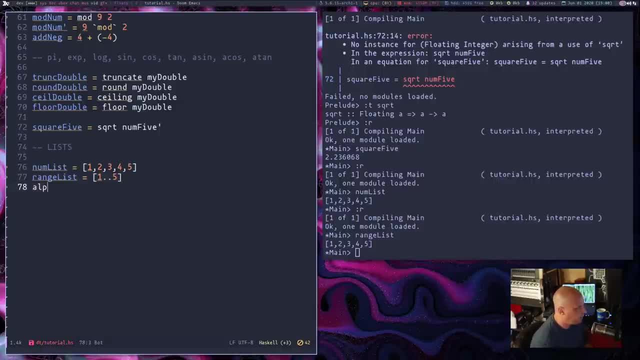 Just write a range. You can also use ranges with characters. So if I did, I'll call it alpha list for alphabet list, And again in the square brackets. Lists have to be in the brackets, But characters have to be in single quotes. 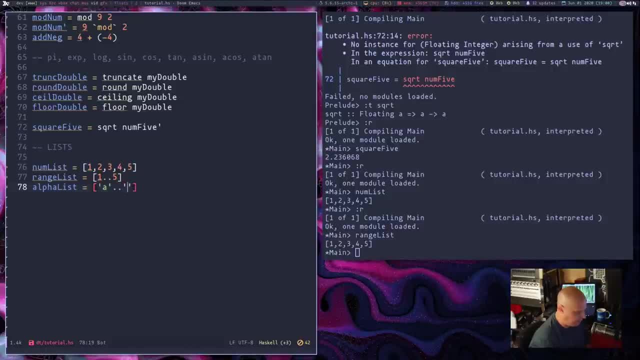 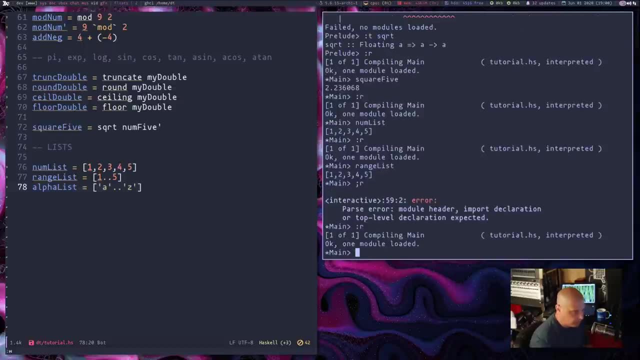 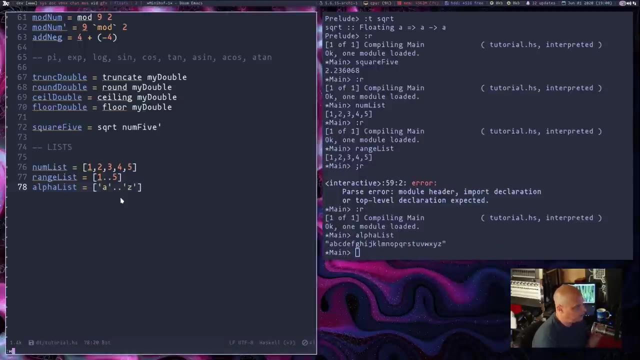 So I'm going to do A in single quotes, dot, dot And then Z in single quotes. Let me write that, Go to the terminal Reload And then do a colon. There we go. And if I do alpha list, You see I get the entire alphabet, A through Z, listed out, because I did the range here. 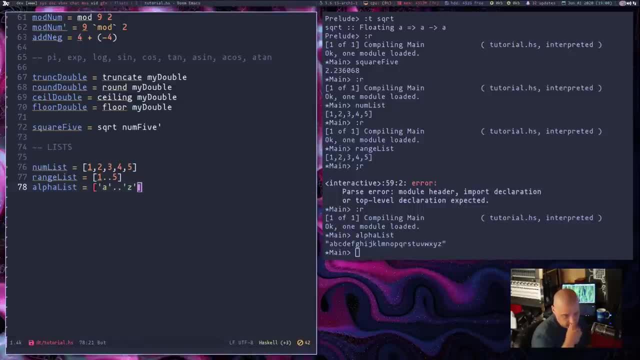 That also would have worked with uppercase. Had I did uppercase A, uppercase Z, I would have got the entire alphabet as uppercase. Now, one interesting thing you can do with ranges Is you can do something like even nums. That's what I'm going to call this. 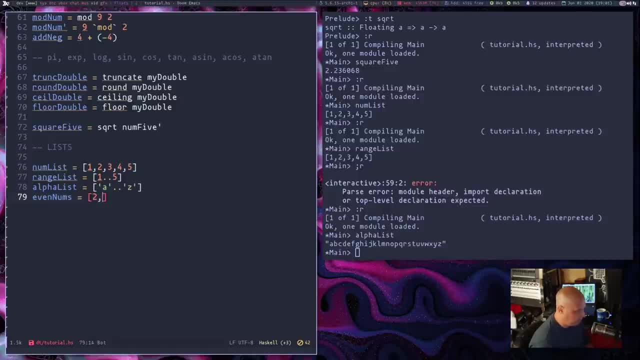 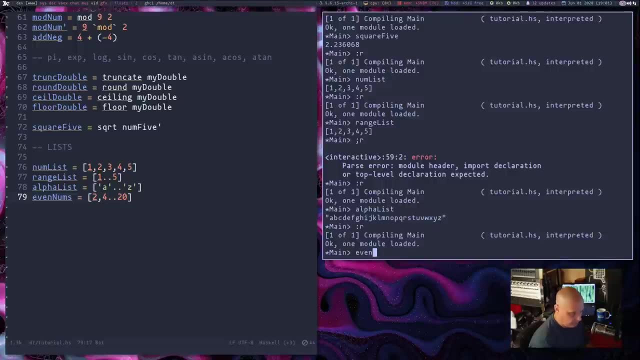 And I'm going to do a list. This time I'm going to do 2, comma 4.. And then dot, dot And then 20.. If I write that, Go to the terminal and reload And do even nums And you see I get 2,, 4,, 6,, 8,, 10, all the way to 20.. 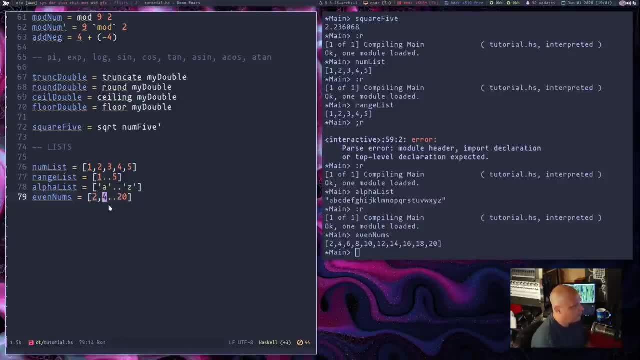 It's smart enough to know for the range. So if I did 1 comma 3. It would have taken the odd numbers actually. So if I change that and do 1 comma 3. And get back into the terminal, Reload and run even nums. 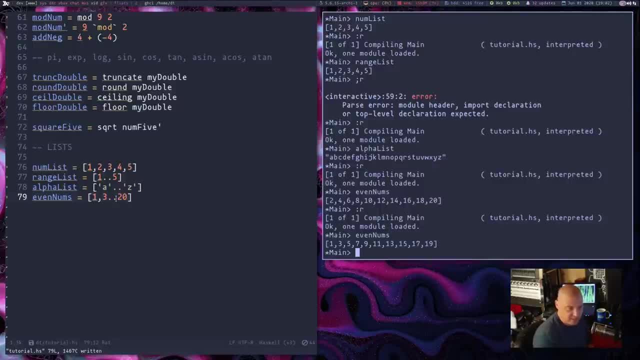 Even though it's going to be odd nums this time. You see, it actually is taking the odd values from 1 through 20.. And in case you're wondering, Yes, it works with the alphabet as well. If I did alphabet with A and then C, 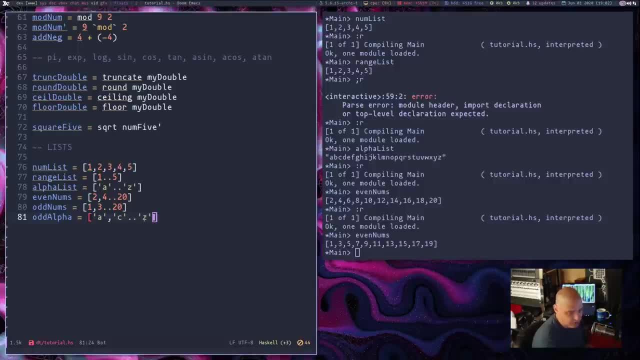 And then the dot dot for the range all the way to Z. It will skip every other character You know, starting with A All the way to Z. Let me write that And I will show you that in action. Let's reload. 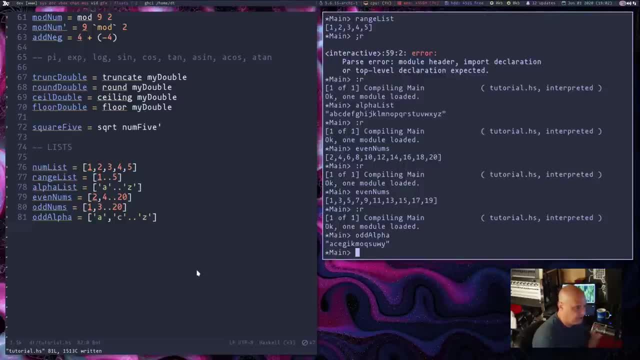 I'm going to run what I called odd alpha here And you see I get A, C, E, G. You know every other letter And you can take the sum of everything in a list. So I created this function here. Sum num list equals sum, and then 1 to 5.. 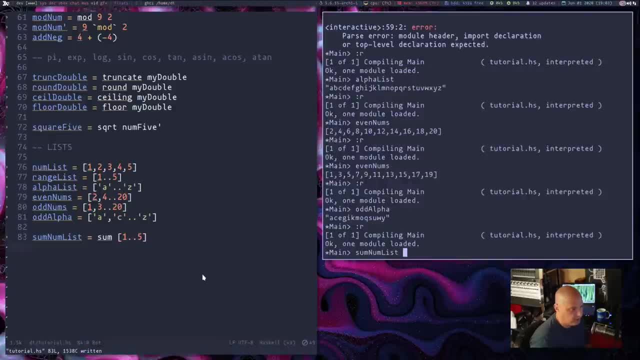 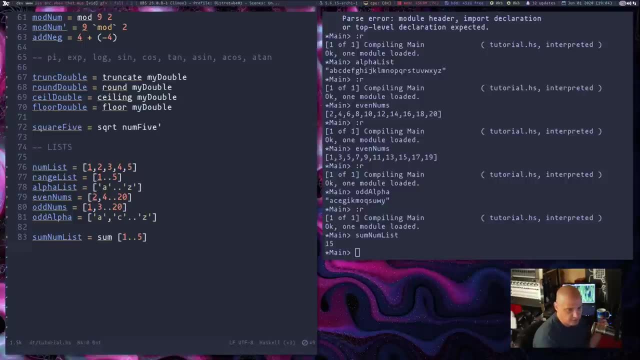 So we're going to add everything 1 to 5. If I run that in GHCI, You see we get 15.. Because that is the sum of every number 1 through 5.. Now, I actually didn't have to write it that way. 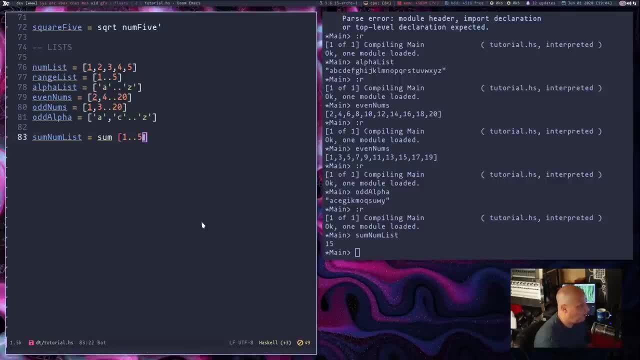 Remember I created num list up here. That is basically just 1 through 5.. So if I wanted to, Let me copy that and paste it. And I'm going to do sum num list Again with a single quote, And this time I'm going to take the sum of num list. 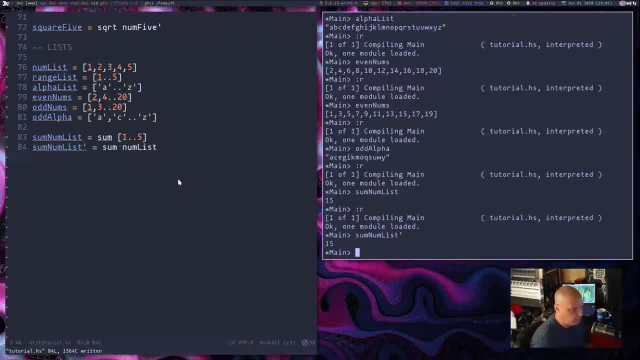 Let's reload and do sum num list With the single quote at the end, And again we get the same output: 15.. Just like you can take the sum of a list, You can take the product too. So if I did, prod num list equals product num list. 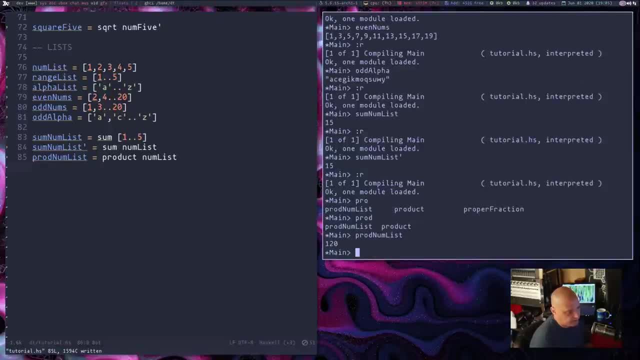 And then we run prod num list in the GHCI. Here I get 120.. Because it took every number in num list, Which is 1 through 5. And basically multiplied them against each other. Now how do you figure out if a certain value is part of a list? 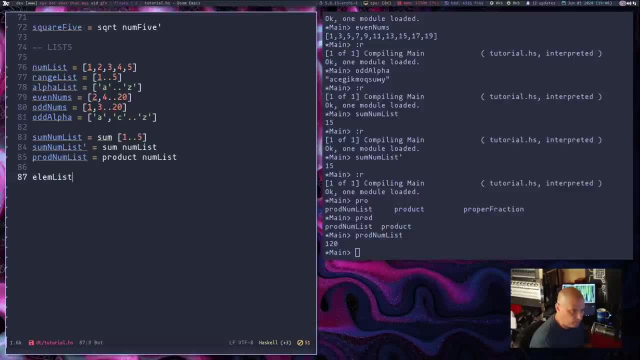 Well, you can do something like this. I'm going to call this elem list, Because it's basically going to use this command, ELEM For element. Is this element part of this list? So I'm going to do elem 5.. 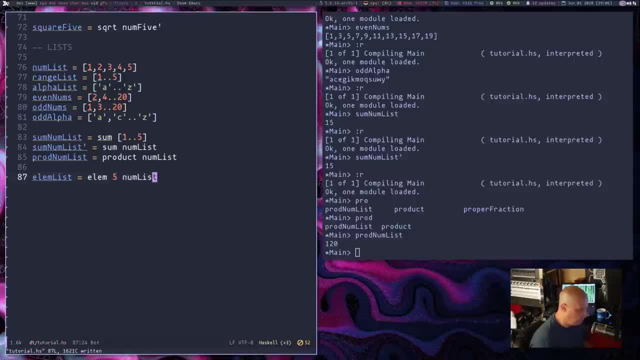 Is that part of num list? Let's write that. Go to the terminal, Reload. And if I run elem list, You see I get a boolean. True. If I would have instead asked, is elem 6 num list, I would have got a false. 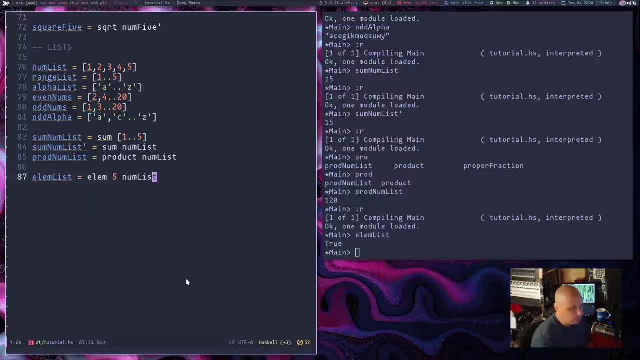 Because 6 is not a part of num list. Now elem is a prefix operator, Similar to how we used mod before, But similar to mod, You could use it as an infix if you wanted. So copy that line and paste it, And I'm going to do elem list with a single quote. 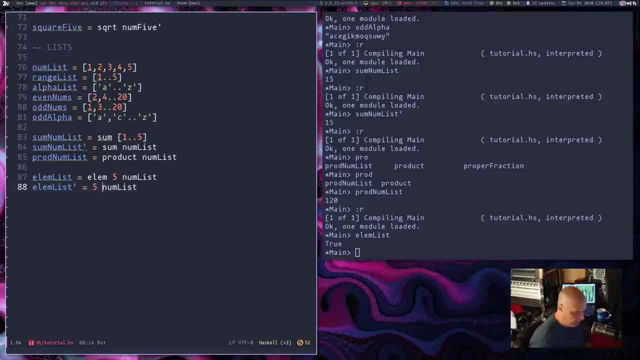 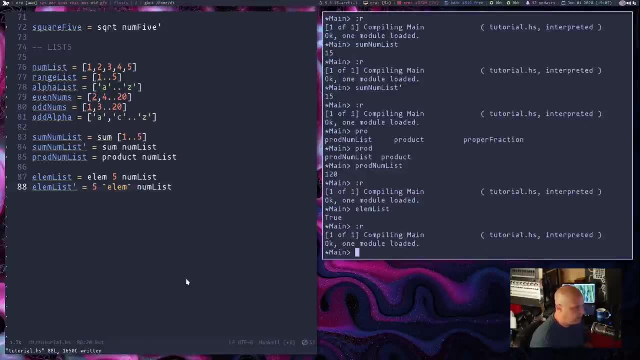 And this time I'm going to do 5.. And then in the ticks here, The back ticks, I'm going to do elem, Write that And reload GHCI here And run elem list single quote. And again we get true, returned. 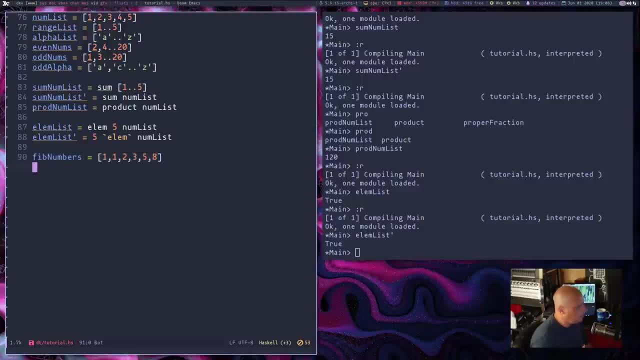 So some other things you can do Is you can create a list. You know I created this list here Called fib numbers. It's the first 6 numbers of the Fibonacci series. Now, if I wanted to, I could create more fibs. 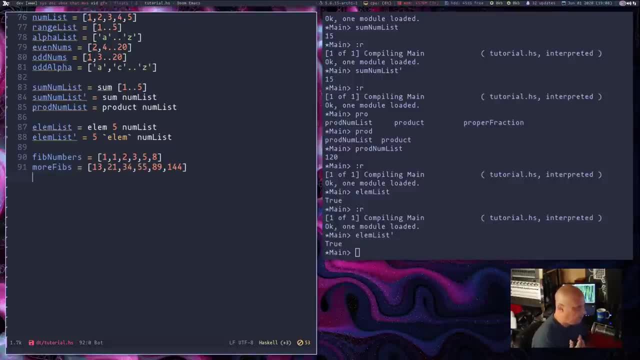 And that list is the next 6 numbers In the Fibonacci sequence. And if I wanted to combine those lists, I could do. combine fibs equals fib numbers, space plus plus More fibs. Let me write that Let's go ahead and recompile. 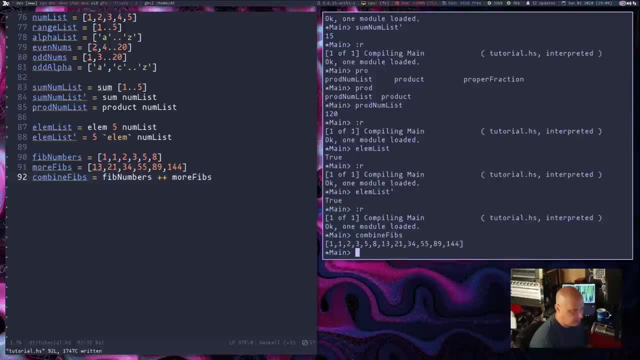 Everything looks good And let's run, combine fibs And you see The output is the combined Fib numbers list And more fibs list And it's the Fibonacci sequence all the way up until 144.. Now sometimes you have these massively long lists. 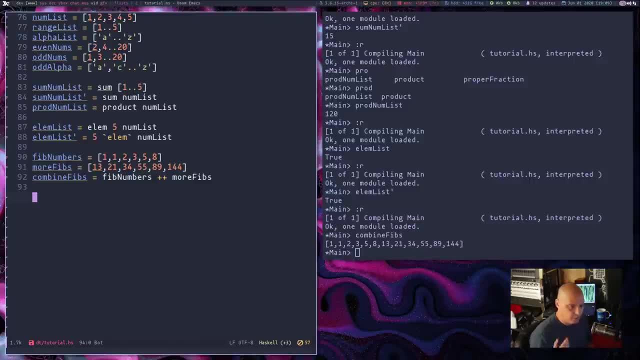 And you want to pick out the largest value of a list Or the smallest value of a list, So you could do that with these commands here: Maximum and minimum. So you can see what's going on here, I created this. Max fib equals the maximum of combined fibs. 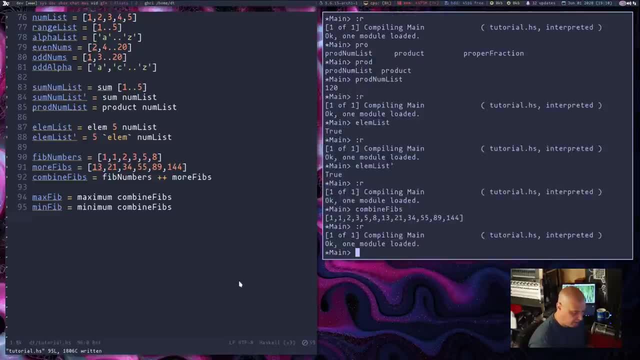 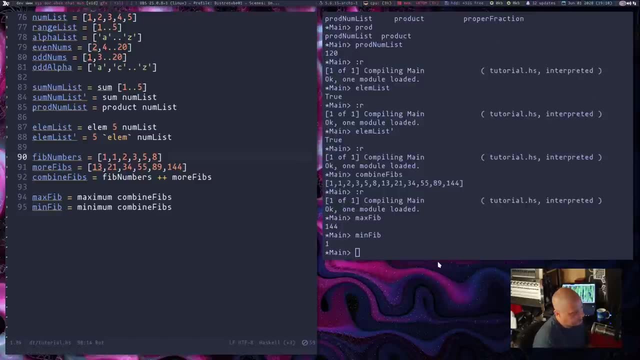 Let's reload this Into GHCI: If I do Max fib, It returns 144.. If I do Min fib, It returns 1.. And now that I'm looking at this I notice I didn't actually start my Fibonacci series. 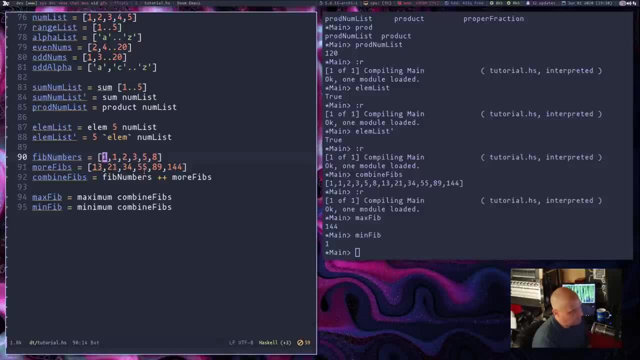 With a 0. Because it really should start 0, 1, 1.. Oh well, My bad, I'm not going to do a retake, though. We're just going to leave it in. Now, what if you wanted to create a list of lists? 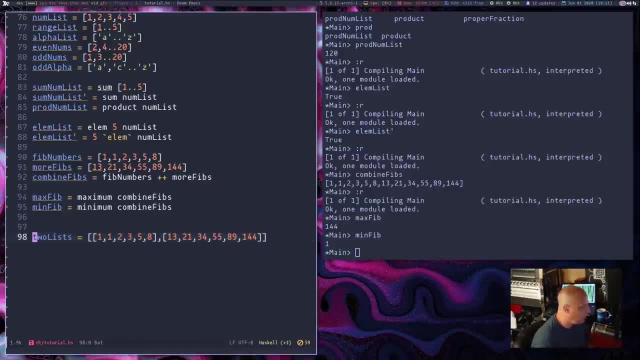 Well, you can do that. So you know, I could do something like: Two lists here Equals A list, So brackets, And then within it You have two other lists, Which is This: 1 through 8 of the Fibonacci series. 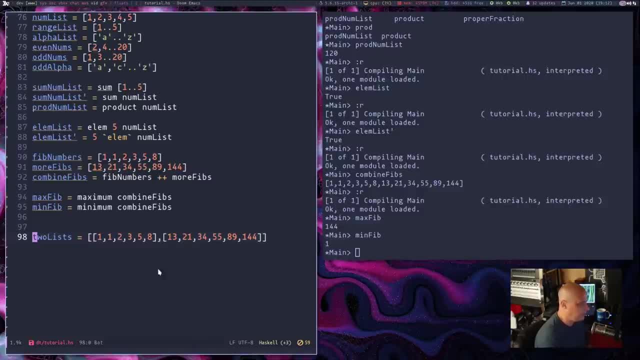 And then 13 through 144. Of the Fibonacci series. You see how that's two lists Within a list. Of course, The better way to write that would be Just make a list Including fib numbers And more fibs. 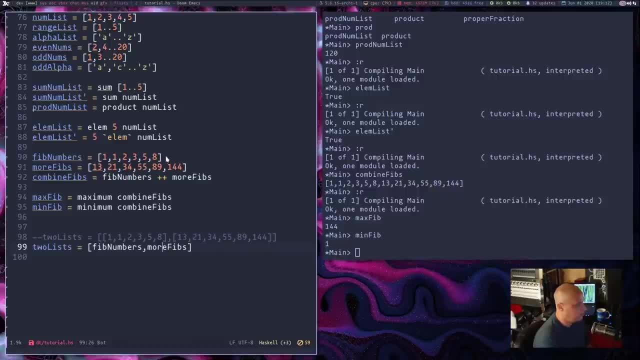 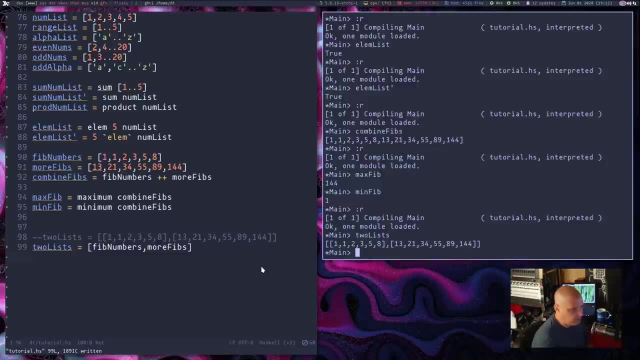 Because that's actually what those two lists were, See fib numbers, More fibs. Let me save. And if we reload In GHCI- And I actually run two lists, You see, One interesting thing you can do with lists Is this command here: 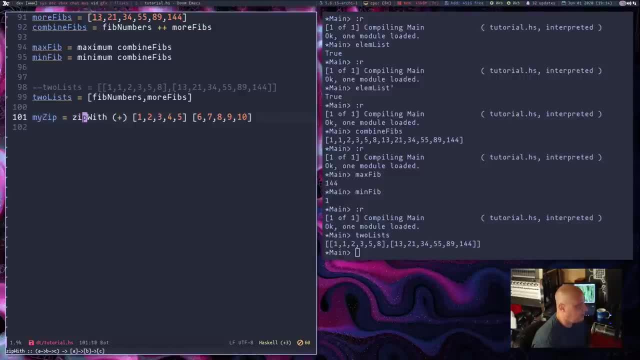 Is zip width, And what this does Is basically saying: Take this action, This function, Which is plus- And that's what I want you to do- To these two lists. So it's going to take 1 in the first list. 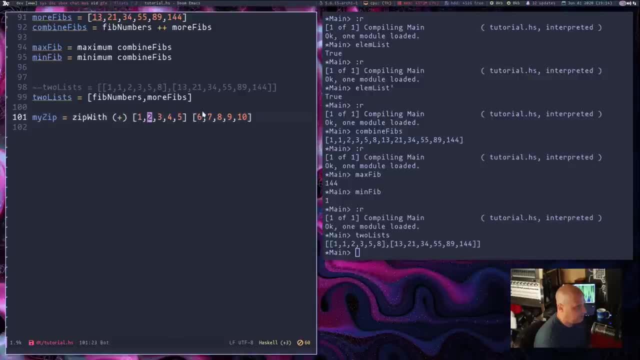 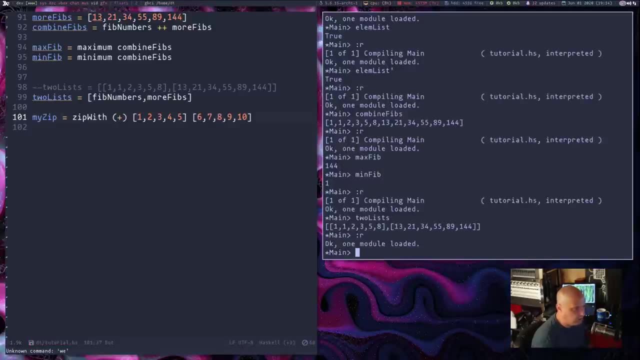 And add it to 6.. Then it's going to take 2 in the first list And add it to 7.. 3 to 8. Etc. So let me save And Let's reload. here I'm going to run my zip. 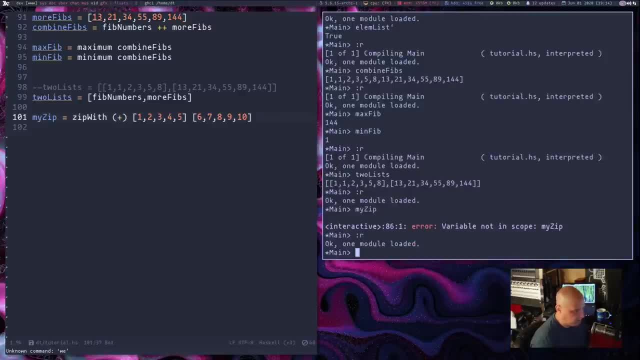 And it says variable, not in scope. Did I not reload this right? I didn't save the file correctly. Let me reload And then run my zip And you see I get 7,, 9,, 11,, 13,, 15.. 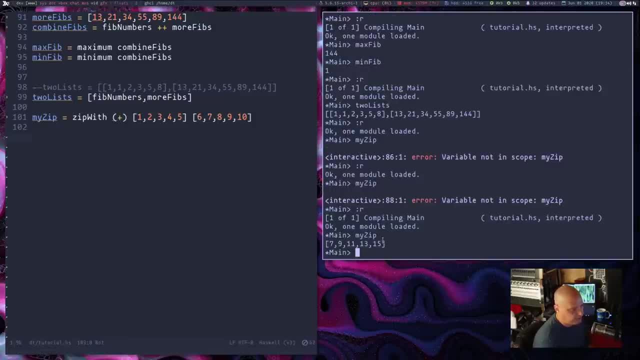 That's the values When each of the pairs are added And, of course, If we use some lists That we had already created, Maybe the fib numbers list And the more fibs list. You want to see that in action With zip width. 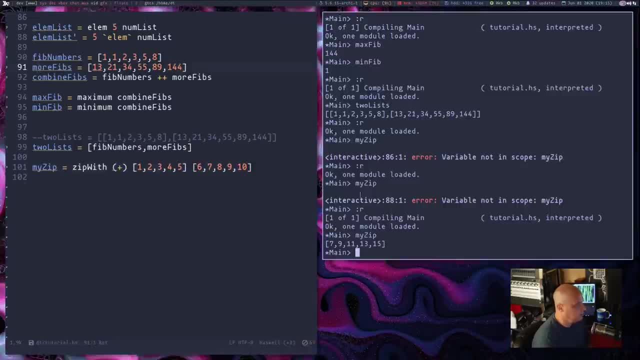 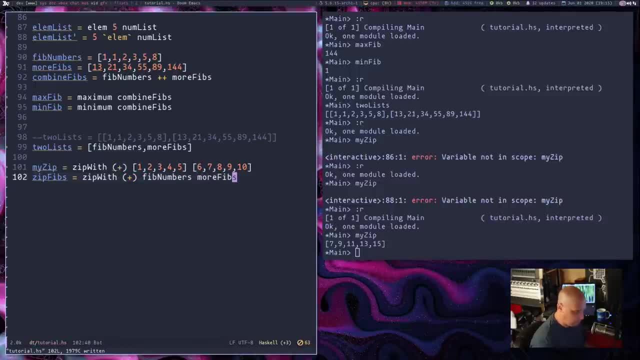 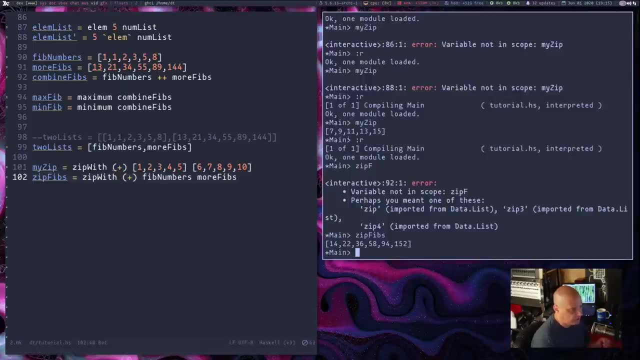 And then We'll do the plus, And then the two lists Are actually going to be Fib numbers, Space And then More fibs. Let's write that And then Recompile Recompiles, just fine. 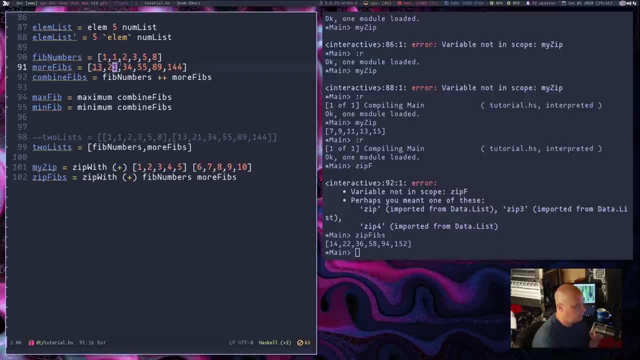 If I run zip fibs, You see I get 14,, 22,, 36,, 58. Which is 1 plus 13.. 1 plus 21.. 2 plus 34. Etc. Now You can create infinite lists. 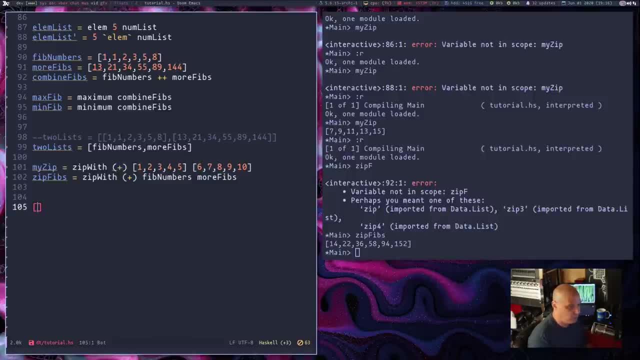 Within Haskell And school's lazy right. It's actually not going to try to evaluate this infinite list unless it needs to. So it's perfectly safe if I wanted to create some variable and have it an infinite list, For example, if I did one comma two and then do two periods again, except this time don't give it. 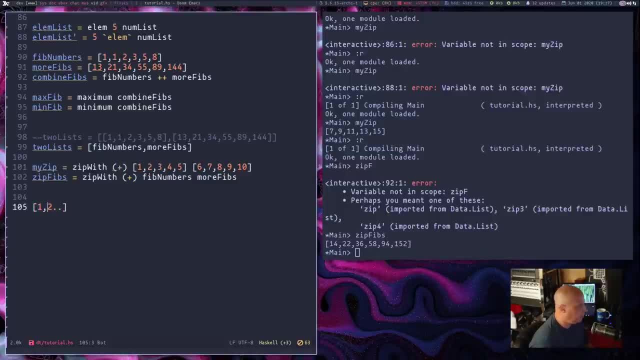 an ending number, just leave it infinite. So that's an example of an infinite list. If I wanted to, of course, I could do something like: inf. odds equals, and then in the brackets, one comma three. you can see we're going to skip every other number, We're just going to take every odd number. 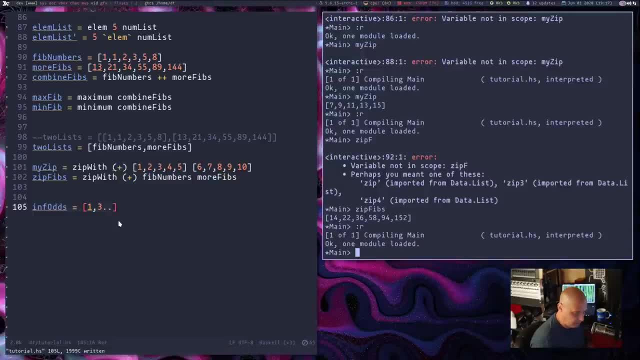 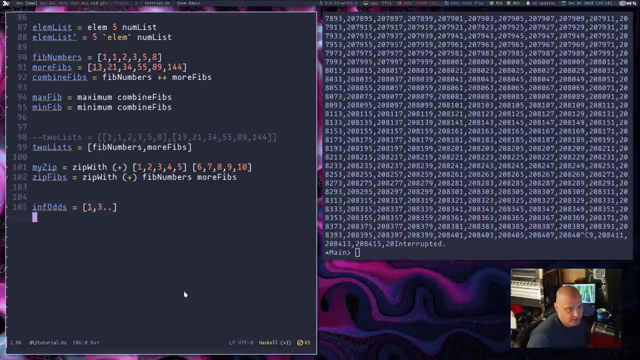 forever, right? So let's get back into GHCI recompile. And if I actually ran this, remember it's to infinity. So I do need to cancel it with a control C because it's going to try to run until the computer completely locks up. So there we go. All right, let me stop that. Now we're. 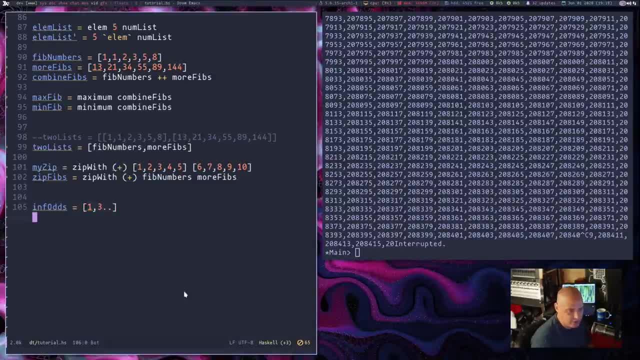 setting these infinite lists. It's useful is you set these infinite lists but then later you tell it exactly where to cut off the infinite list. For example, I'm going to create this function here- take odds equals- and I'm going to run the command take, Take. basically is we're presenting it with a list. 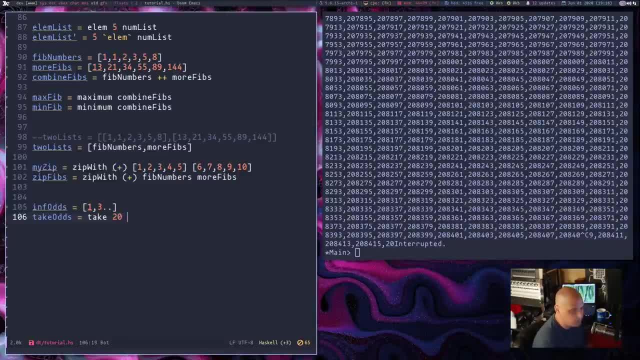 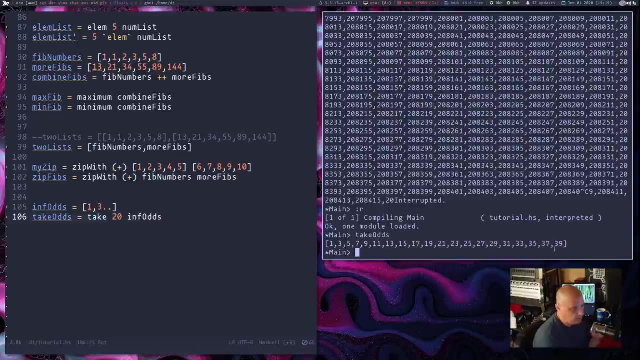 and we're saying: take this many members of that list, In this case 20.. I want the first 20 of infinite odds, So inf odds. write that, let's recompile. And if I run, take odds this time I get every odd number up to 39, because that's the first 20 odd. 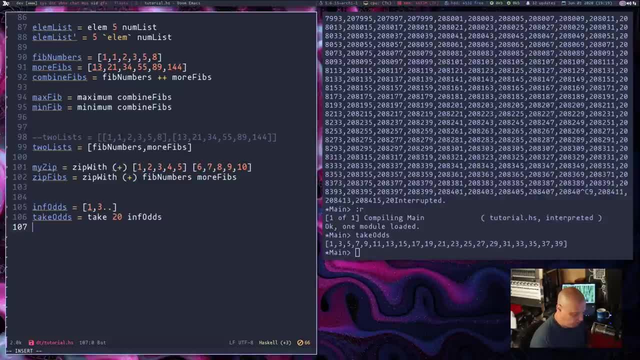 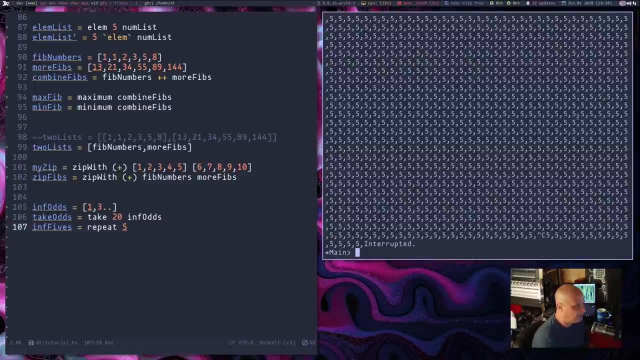 numbers. If we wanted an infinite amount of a particular numeral, I could do inf fives, equals and then this command repeat and then the numeral five and that will just spit out fives forever. So if I recompile and do an inf fives, you can see it's just going to spit out fives. 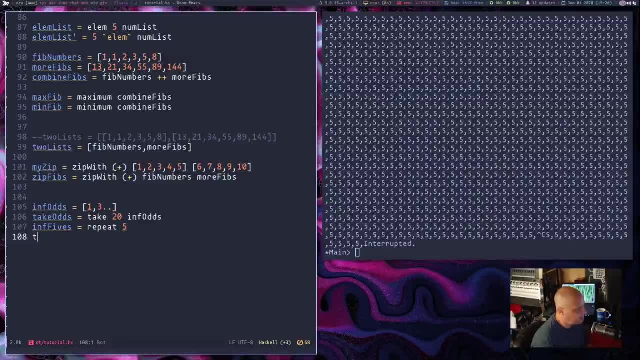 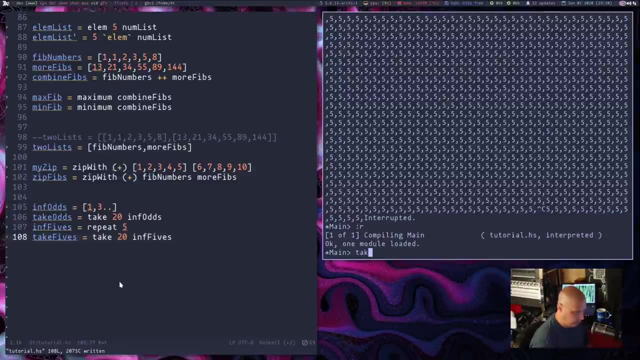 until we tell it to stop at some point. So let's tell it to stop. I'm going to create: take fives. This time I want to take 20 and then inf fives. So remember, this is going to repeat forever, Infinite number of repeats. but we're saying: just take 20 of them, Let's recompile and 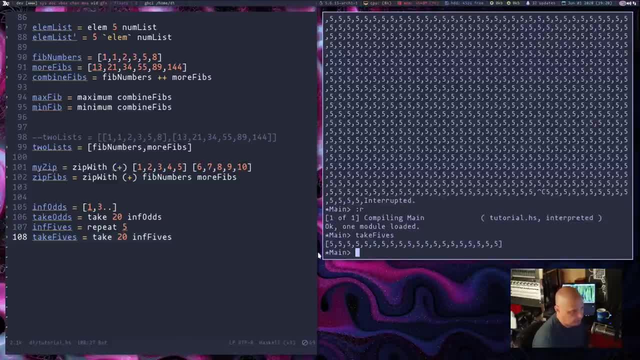 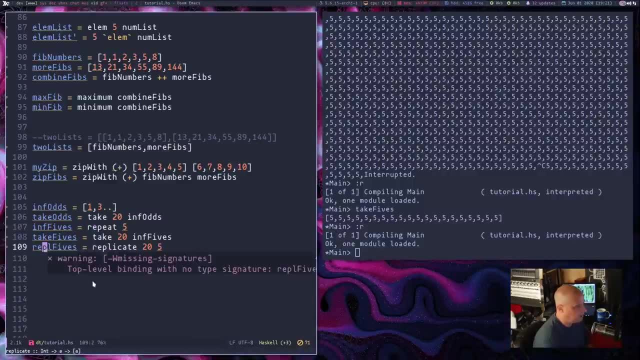 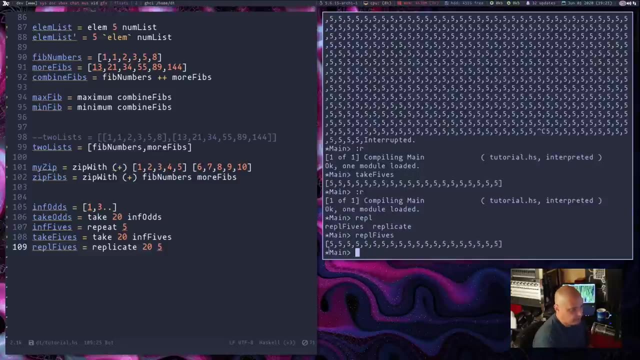 do a take fives And this time I get just a list of 20 fives Similar to take. you also have the command replicate, So I created this repl. fives is replicate 20 times the numeral five And if you want to see this in action, you can see. 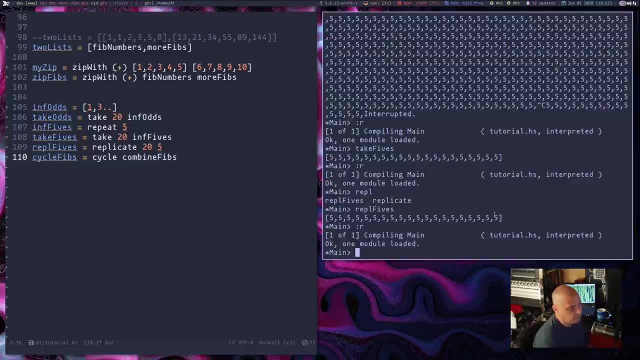 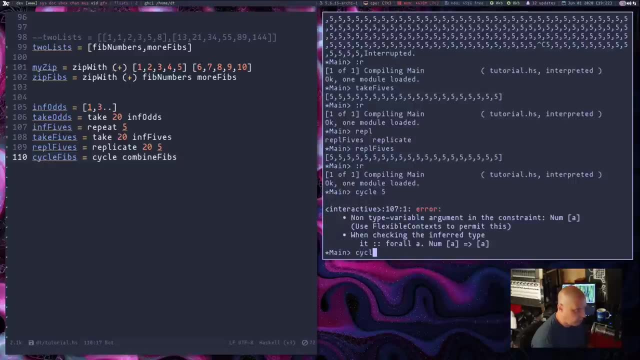 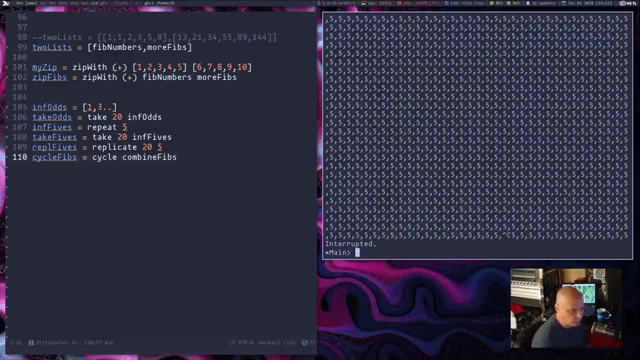 It's another list containing 20 fives. Another interesting command is cycle. So if inside GHCI if I just did cycle five or return to error, I need to cycle and it needs to be a part of a list. So in brackets five, I get fives forever. Let me control C to kill that. I created this. 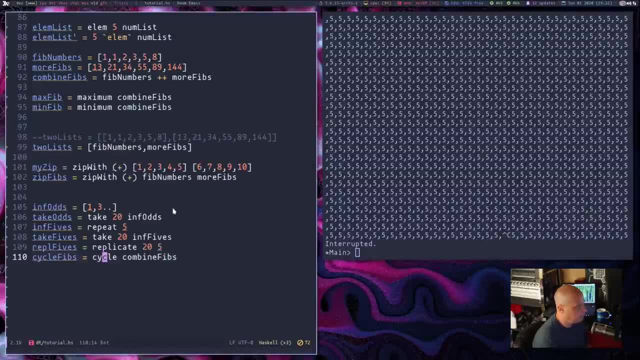 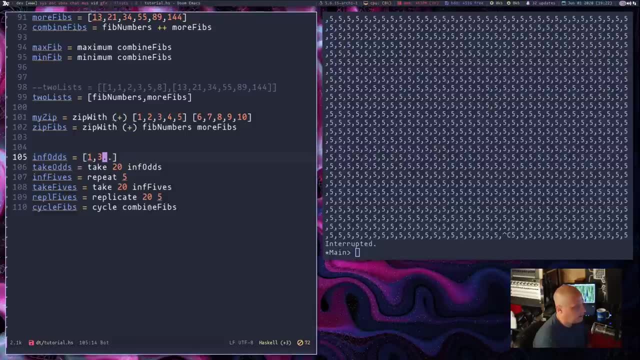 over here, though. Cycle fibs equals cycle combined fibs. You remember our combined fibs list, which is every Fibonacci sequence, number one through 144.. We're going to say, take that and cycle it forever. So basically, just one through 144 in the Fibonacci sequence. 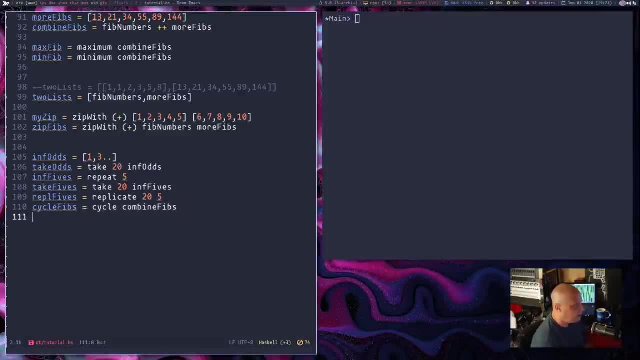 just cycled over and, over and over again. Why don't we do a combination of take and cycle? I'm going to do take, cycle equals, and let's take the first 50 values of and then, in parentheses, cycle, and we'll give it a list. I'm going to do a list of one, two, three, four, five, six, seven. eight, nine and then 10,, 11,, 12,, 13,, 14,, 15,, 16,, 17,, 18,, 19,, 20,, 21,, 22,, 23,, 24,, 25,, 26,, 27,, 28,, 29,, 30,, 30,, 31,. 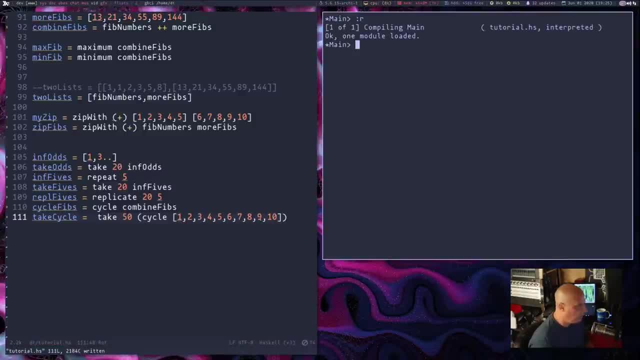 32.. Let's write that and let's recompile, And if I do a take, if I can spell take cycle, what it does is it cycles one through 10, over and over again, but it only takes the first 50 values. 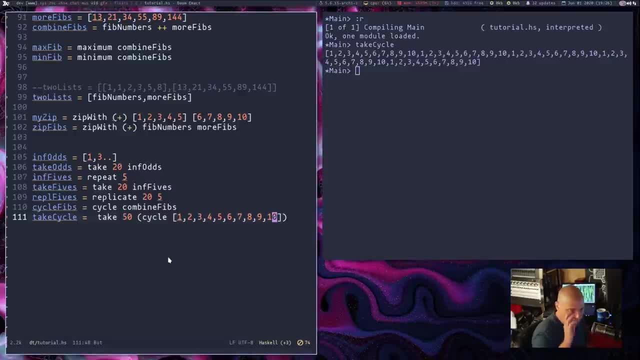 So really it only runs that list five times. One interesting note about the syntax of Haskell is: you know you run a command take and then you run another command inside of it. you know with the parentheses That's kind of standard syntax. you see in a lot of programming. 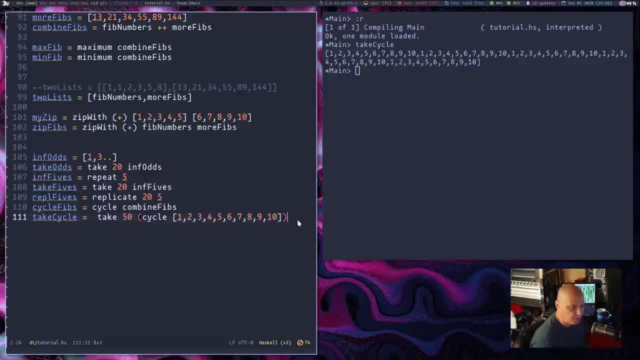 languages. but Haskell does something really unique. Instead of doing the parentheses, we could get rid of those parentheses around cycle in the list. Just put a dollar symbol. A dollar symbol means take 50 and then in parentheses everything else. That's after it. 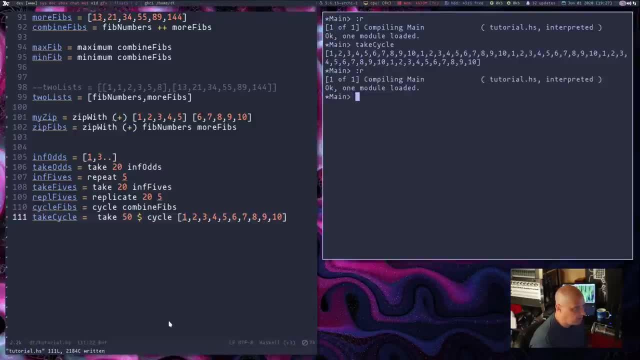 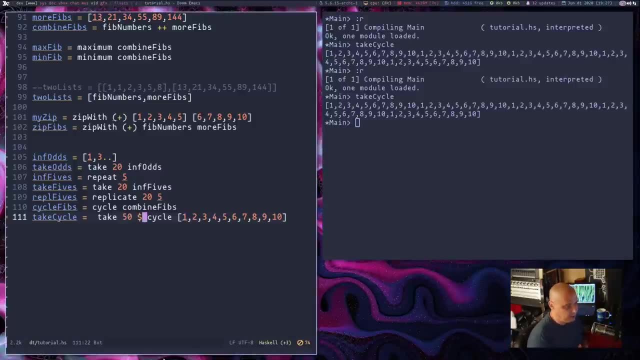 That's exactly what that means. So if I write that and go back and recompile, it recompiles just fine. Take cycle Again, it works exactly the same. It's one of the confusing things, especially new people to Haskell. When you open up a Haskell program, there's all these dollar signs everywhere and 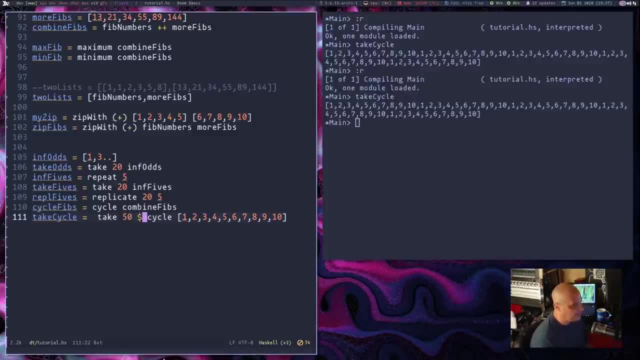 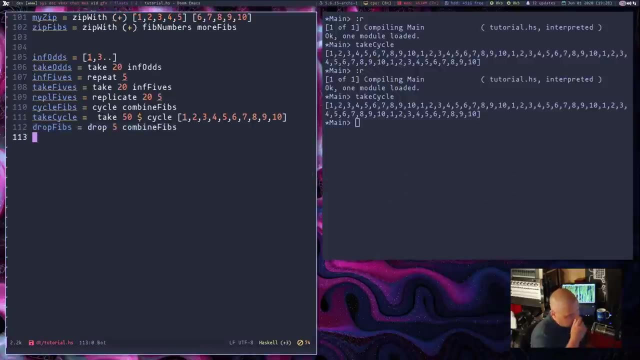 nobody knows what they mean. Well, it's basically the same thing as a parentheses. It's just an easier and, quite frankly, a cleaner way of writing things. If you've ever used a language that has a lot of nested parentheses, it gets confusing fast. I'm looking at ULISP. Similar to take there is. 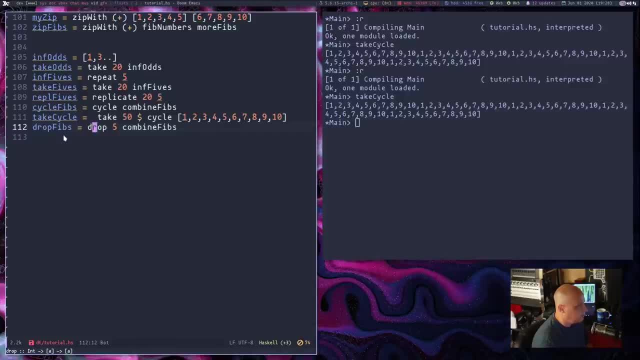 also a command called drop. So I created drop fibs here and it's going to run the command drop five. So drop The first five of this list. combined fibs. Remember the combined fib list. recompile and run drop fibs. 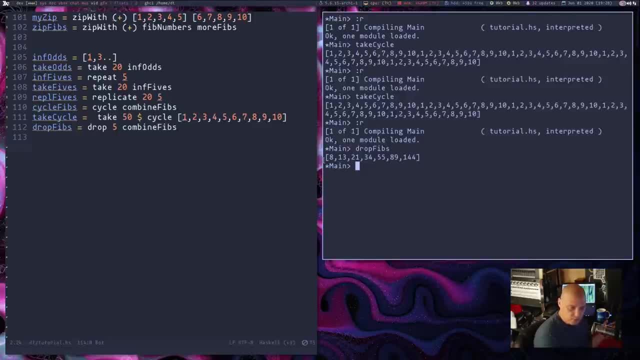 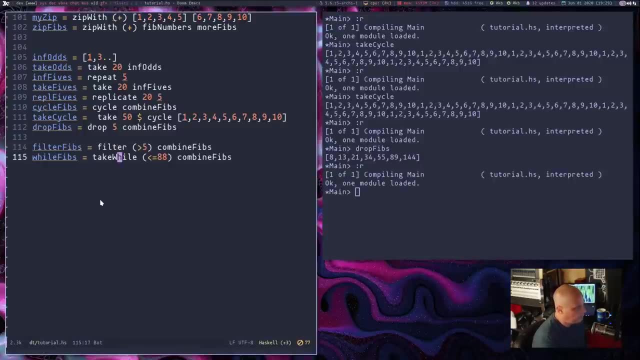 And you see, we get the combined Fibonacci sequence list from before, except it dropped the first five members of that list. A couple of interesting commands. It's also filter and take wall. So if I do filter and then in parentheses, greater than five and then combined fibs, it's going to take. 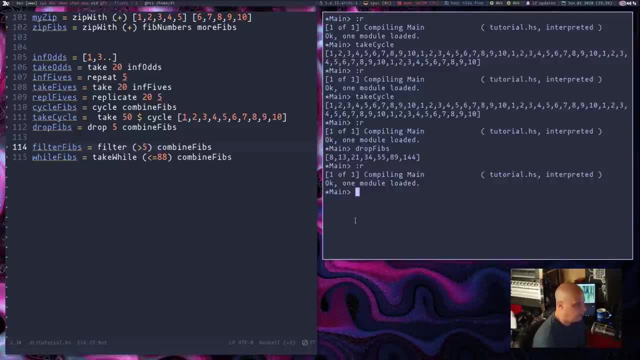 the combined fib list and filter out everything except the The ones that are greater than five, and you see it returns the combined fib list itself, Only the ones that had a value greater than five. Then I created this here called wall fibs, and that is take while anything that is less than or equal to 88 and combined fibs. 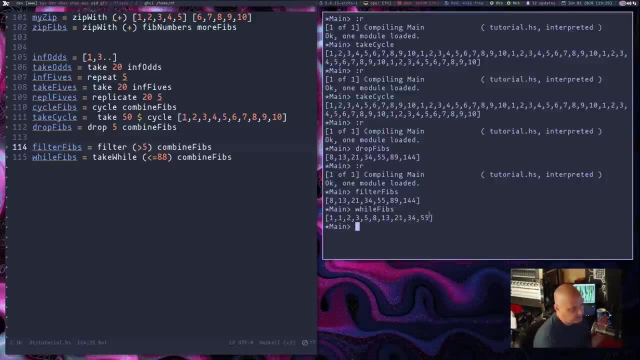 And if I run that, you see I get the combined fibs list up until the characters get greater than or equal to 88. Now I'm going to create this here, I'm going to call it map list and I'm going to show you. 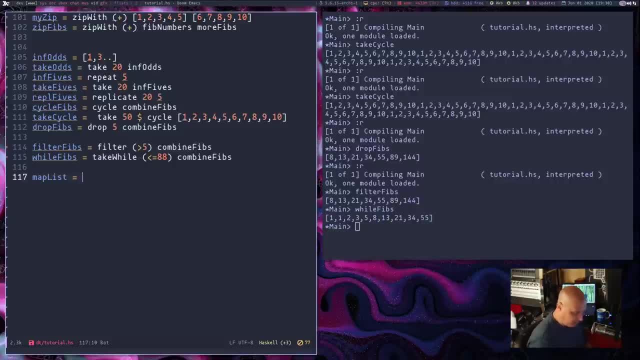 One of the most often used commands- probably in Haskell, You see it everywhere- And that's the map command. map is basically saying: take this and do it to every member of a list. So I'm going to do map and then, in parentheses, I'm going to do times two and then let's create a list here for it to do all of this on. 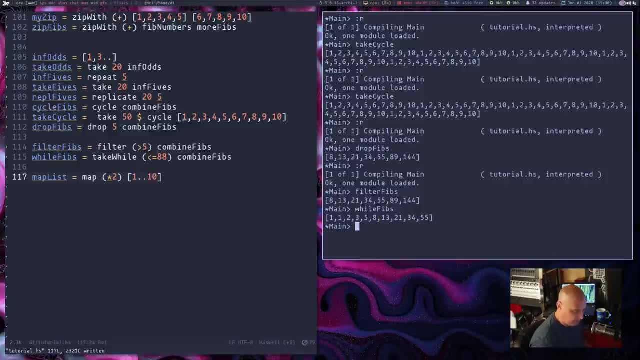 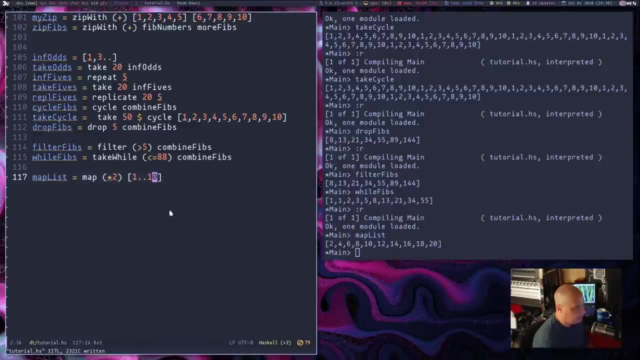 So I'm going to do one through ten and let me save that and recompile. And if I run map list you see it takes one through ten and it runs times two on Each member of that list. Now how do you sort an unordered list? 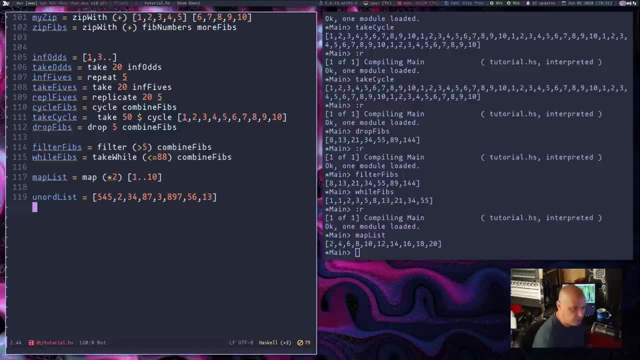 Well, let's create an unordered list here. So I created this list of a bunch of numerals. They're completely out of order. Well, let's sort them. So I'm going to create sort list equals and then run this command: sort. 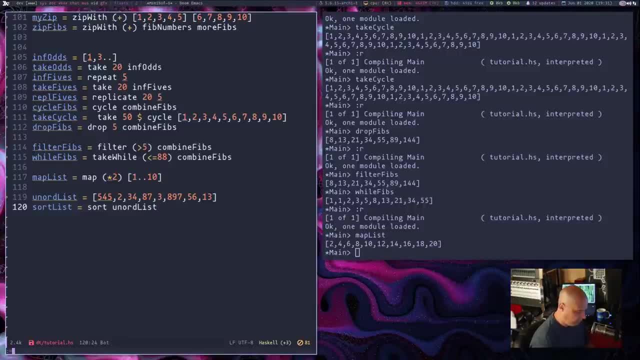 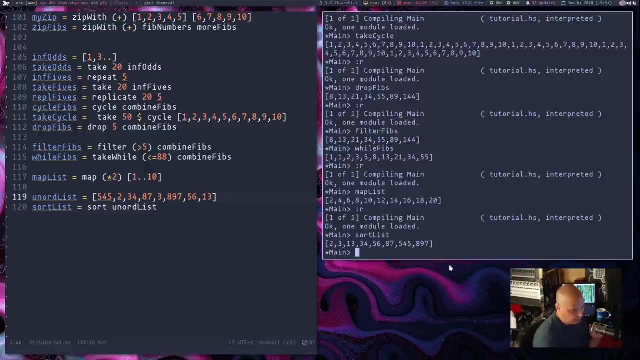 And what are we sorting? where we're going to sort, of course, the unordered list here. Save that And if I do sort list here, you see it takes the unordered list and it sorts them in the correct order. Let me do a colon exclamation point clear again to clear the screen. 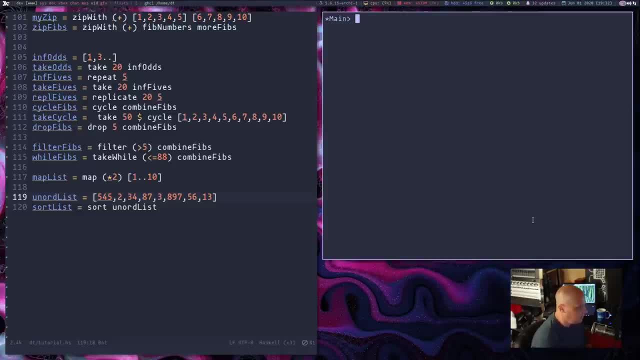 Let me do a colon exclamation point clear again to clear the screen. Let me do a colon exclamation point clear again to clear the screen here. I won't bother writing these as functions in the tutorial dot hs, I'll just do these interactively here in GHCI. 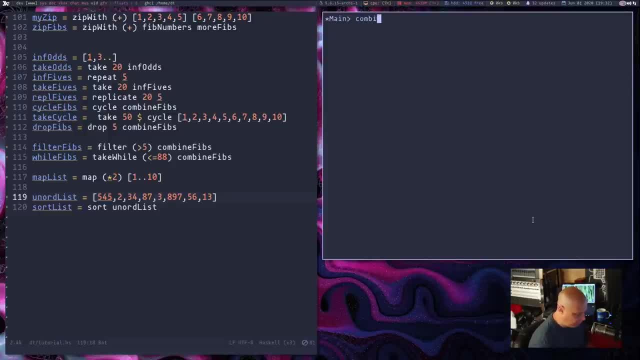 Let's talk about head, tail, last, and a knit. So you remember, combine fibs, that list. Well, what? if we do head combined fibs, It takes the very first value in that list, And if we do a tail combined fibs, it takes every member of that list but the first value. 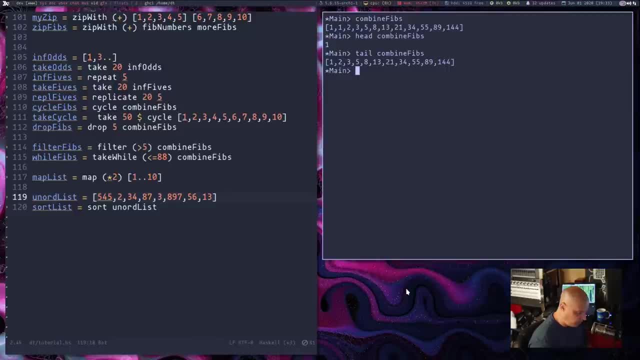 So remember head, tail last and a knit: Remember: head is the first value, tail is everything but the first value. Similarly, we also have last, you know that command, And if I do it on combined fibs, I get the very last value, which is 144.. 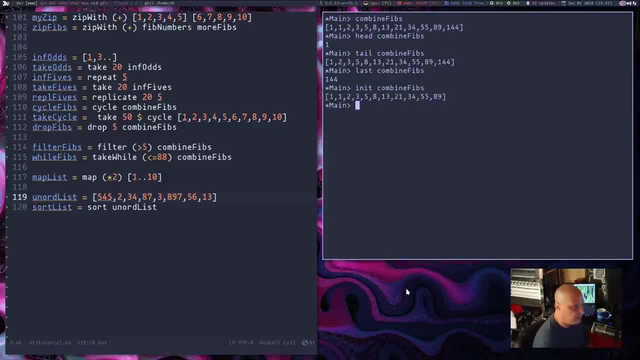 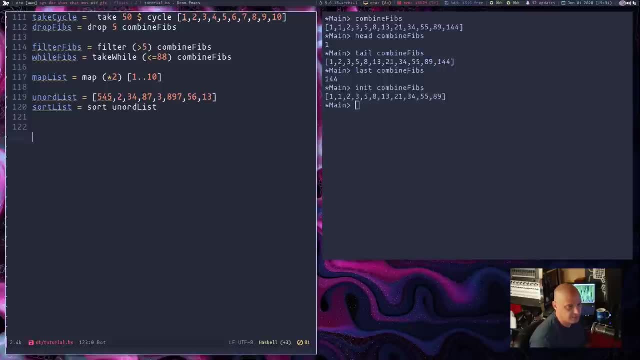 And we have a knit which is every member of that list except the last. So remember head, tail, last a knit. The next commands I want to talk about are fold R and fold L. So I'm going to create this here. I'm going to do: 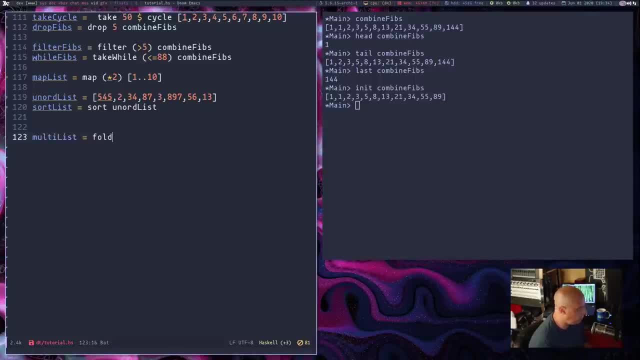 Multi list equals and I'm going to use the fold R command and it needs to do something And I'm going to tell it to do a multiplication here and then I'm going to do one and then a list. inside the list I'm going to do two, three, four, five. 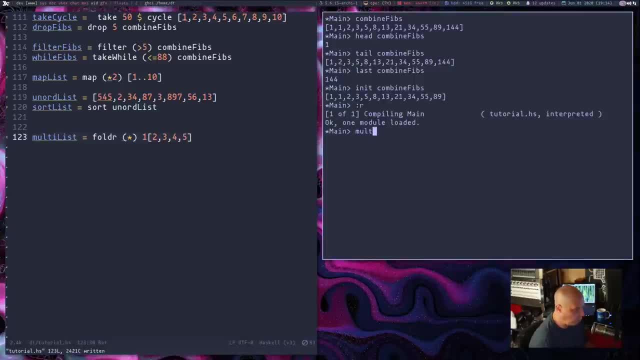 If I save that recompile and I run multi list, we get 120 returned. Exactly what is fold R doing? Well, fold R is basically taking some function F and then some value E, and it's doing it to the members of that list. 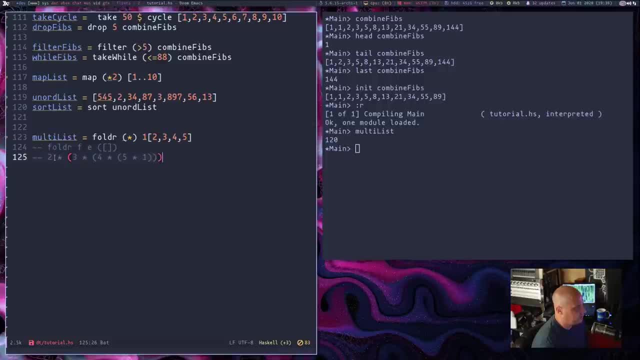 And here I've rewritten it basically what multi list is doing. It's taking two times, and then in parentheses three times, and then in parentheses four times, and then in parentheses five times and then one, because one was the value outside of the list here. 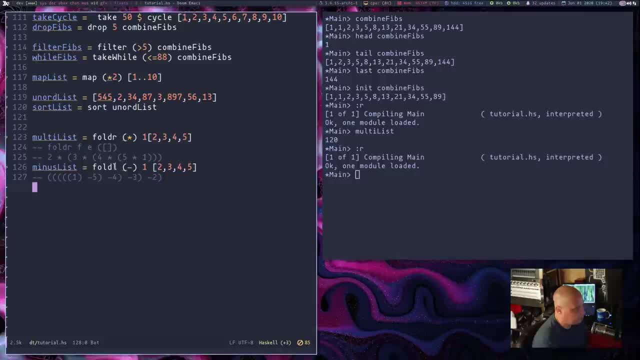 And here is something created with fold L, And the difference between Fold L and fold R does make a difference in this case, because we're doing subtraction, So what order we're starting in of the list, what direction we're going, does make a difference. 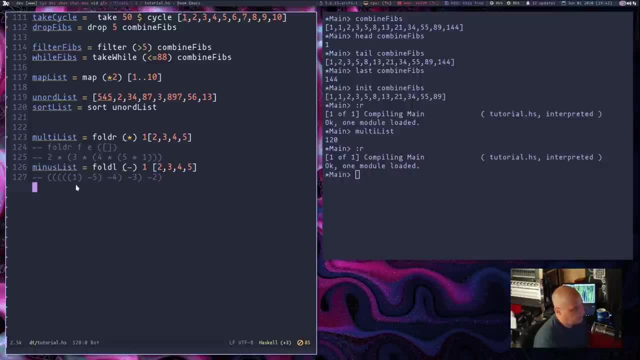 Basically, what this is- the same as writing- is a whole bunch of parentheses- one- and then closing parentheses minus five, closing parentheses minus four, closing parentheses minus three, And again we're minusing, starting with one, five, four, three, two. 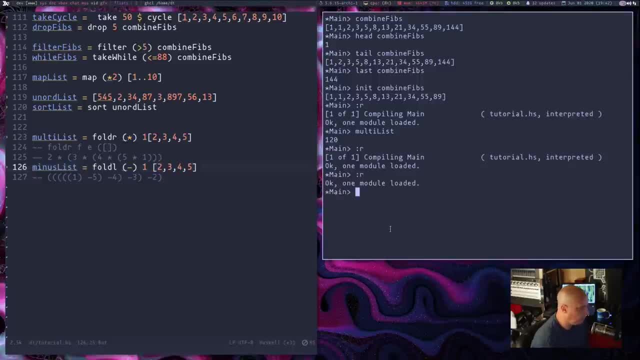 I hope that makes sense. If I actually reload here And if I run minus list here, I get minus 13, which is exactly what I would have expected on that. And one of the favorite things people love to do with programing is writing the same thing multiple ways. 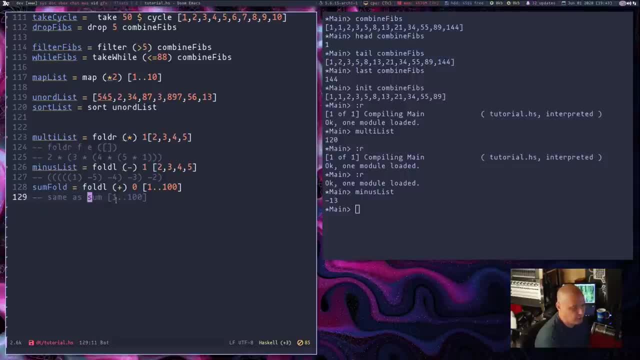 Here is an example of doing the same thing as taking the sum of everything one through 100.. Well, you could do that with fold L, fold L plus zero, and then a list one through 100.. Let's recompile and do some fold. 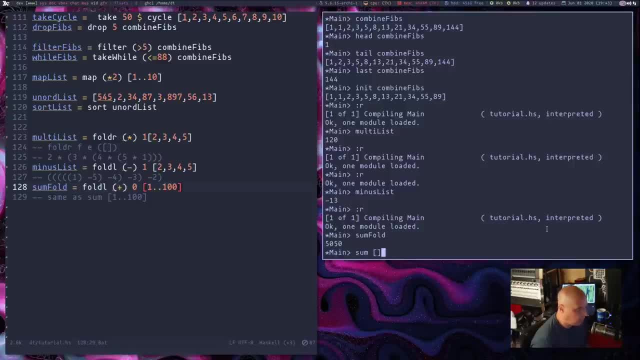 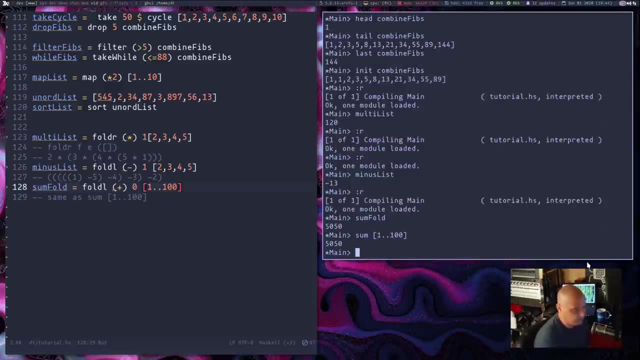 I get 50.. 50. And if I just ran a sum on one to 100, just to verify that that is the same value. So just two different ways of writing the same thing there. Obviously the same way of doing. it is just using some. 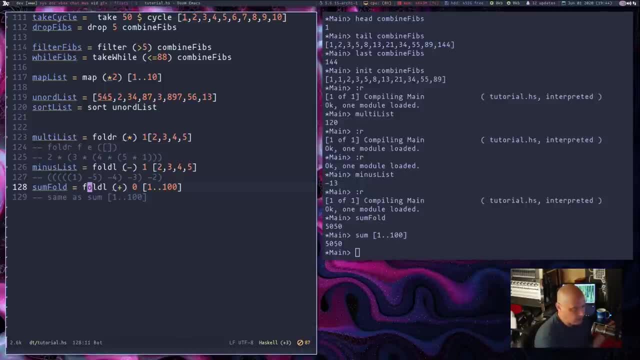 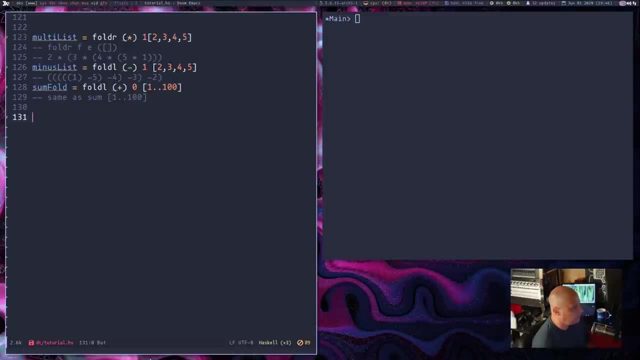 This was just showing you that it's possible to do it with fold L as well. Now let's talk about how you add something to a an existing list and Haskell And to do this. typically you prepend a list Rather than adding. 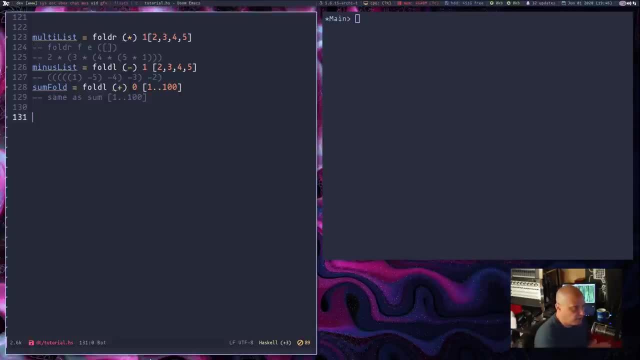 Something to the end of a list, because some lists can be quite large And if Haskell has to basically evaluate the entire list, you know, to add something to it that can take some time. It's much easier to just add something as the first element of a list. 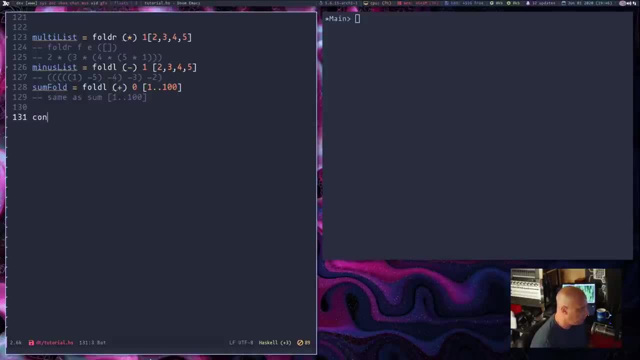 And you use what is called cons to do this. So if I create this variable here, cons list, and what I'm going to do is I'm going to do one and then colon and then an empty list. I'm basically saying, take this empty. 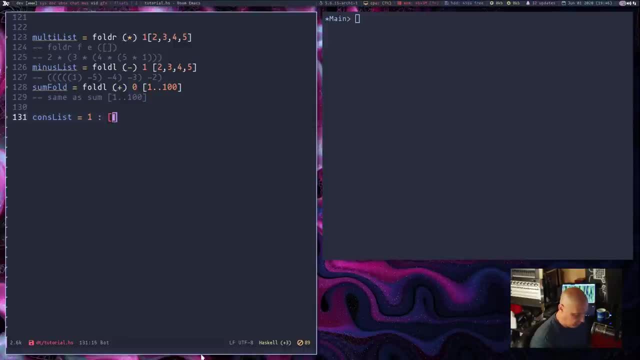 And then at the beginning of that empty list, I want you to add a one to it. That's right, Recompile. Let's run cons list and you can see one is the only value. but I could keep prepending stuff here if I wanted to. 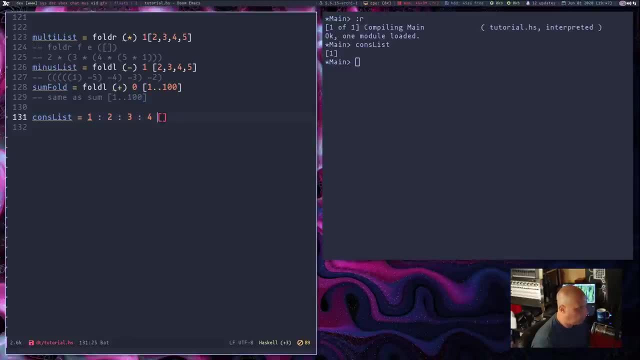 I could do two colon three, colon four, colon five, And then of course you have to do a colon before the empty list. Let me write that and let's recompile, And this time, when I run cons list, I get a list containing: 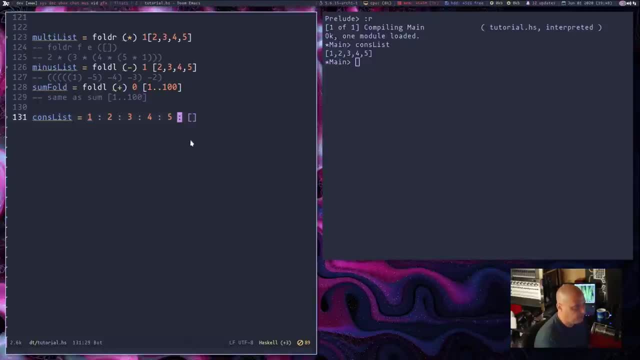 One, two, three, four, five, because it repended one through five to the empty list. Well, we could have done that with any list. You remember the combined fibs list from earlier. Well, we could have done a sixty six colon combined fibs. 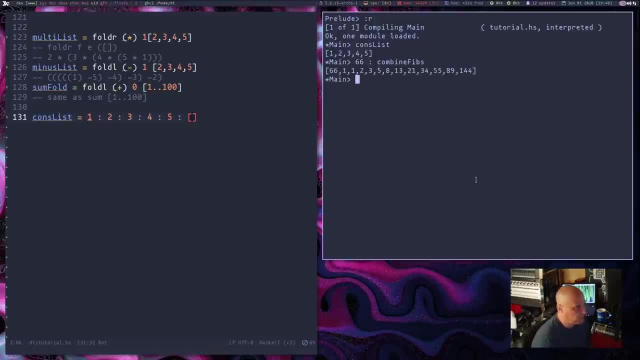 This is saying: take the combined fibs list and prepend it with the number sixty six And you see there's sixty six at the beginning of the fib sequence. By the way, creating a fib sequence, wouldn't it be great if Haskell could figure out a range? 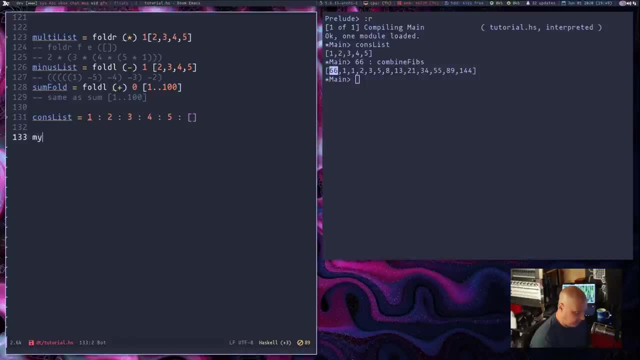 As far as the fib sequence, it can't, but it would be nice if we could do something like my fibs equals. And then we did a list of like zero, one, one, two, three and then the dot dot. 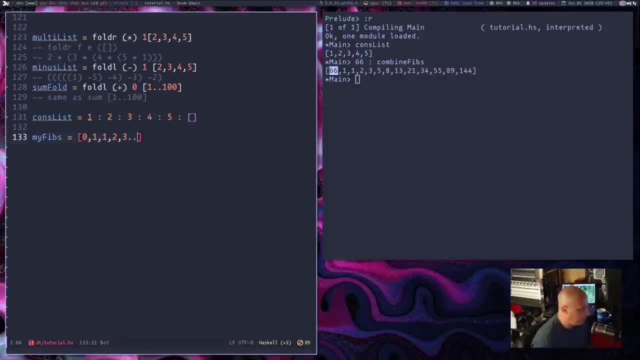 And it would figure out what we're doing. Well, that's not the way ranges work. Ranges only take the two comma separated values at the beginning and then the dot, dot. So there's no real way to make a fib list. It just doesn't work well. 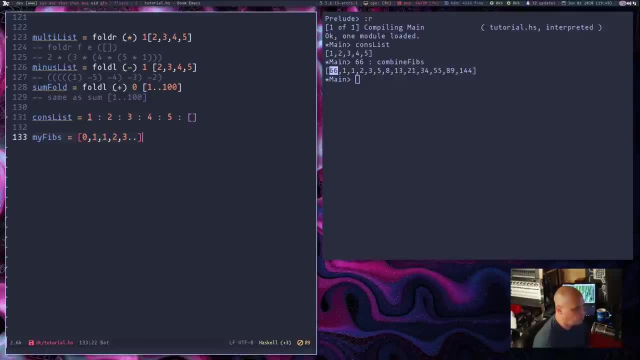 We've learned enough, though. I mean With tail zip with and with the cons operator here. prepending lists, we could actually create a function that creates a Fibonacci sequence for us, So I'm going to write this right here: Fibs for infinite. Fibonacci equals zero colon, one colon. 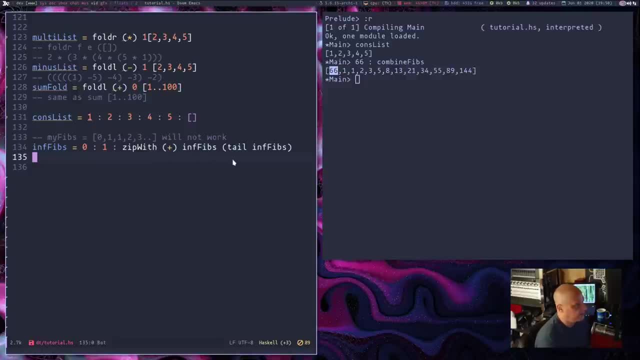 Then zip with plus infinite fibs again and then in parentheses tell infinite fibs. Now I don't want to explain too much of this because I want some of you guys to actually think about that. Pause the video, if you need to, and see if you can figure out exactly what is going on with that. 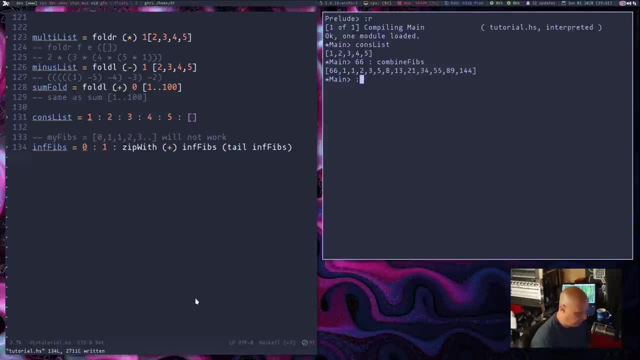 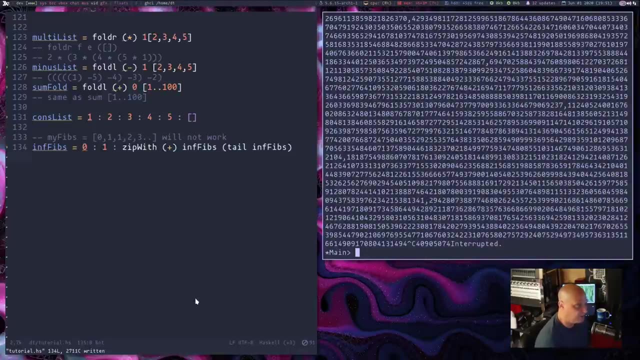 But while you do that, I'm going to go ahead and write this and I will recompile and I will run Fibs just to show you that it will actually calculate Fibonacci sequence numbers into infinity. A better way to have done that would be something like: take 30 of those numbers of the Fibs. 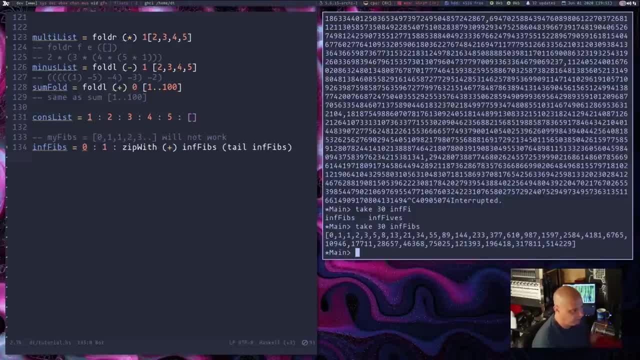 And you see, I get the first 30 Fibonacci numbers. They get quite big Very quickly. So now that you've had a minute to think about it, I will give you some clues as to what's going on with this zero and one. 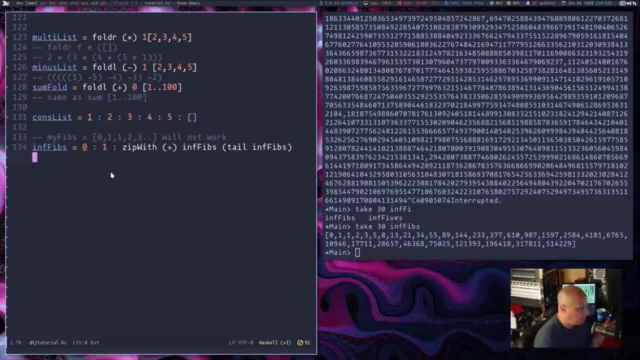 We're basically taking a list and we're starting with zero and one, and then we're doing a zip with plus on two different lists. What are the two different lists? Well, the tail of Fibs, which is just one, and then Fibs itself, which is zero and one. 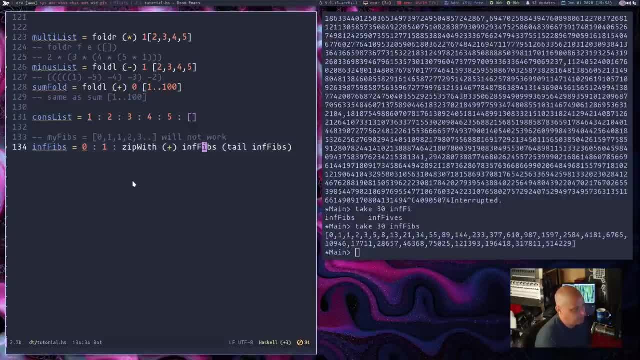 You may need to actually diagram that on paper or type it out or something to figure out what it's doing. So I will do that Right now. so it's basically taking this list of zero and one, and then another list which is just the tail of the list, which is when we're starting out- just one. 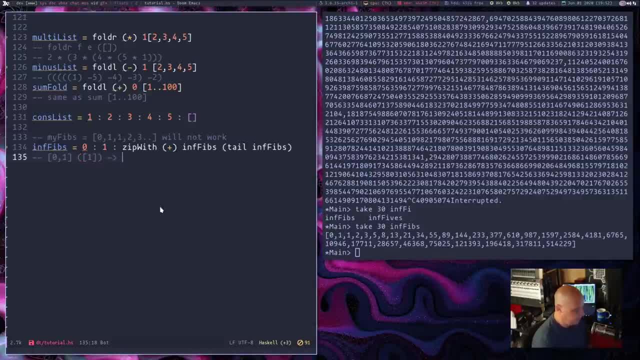 And then, once it does the zip with on the two lists, what are we ending up with? Well, at that point we would have one and Two in the list, but then we keep telling it to keep preventing zero and one, zero, one, one and two. 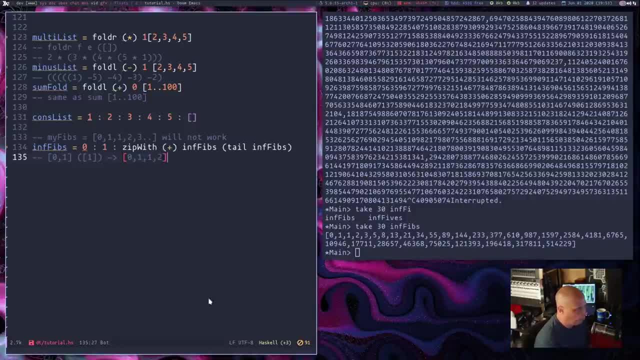 Actually become the list And then, because it's going to keep repeating, then we take the tail of that new list, which the tail of the new list is one, one and two. Then, once it adds those up again, we get a new list. 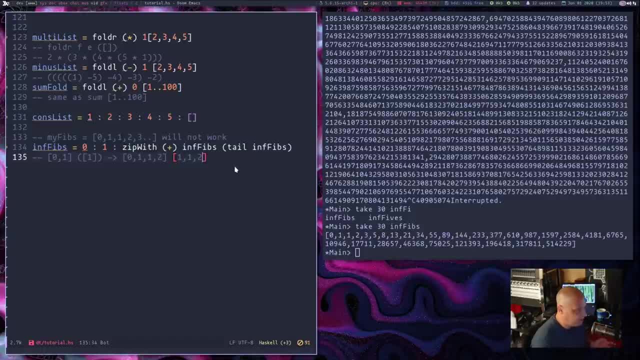 The new list is going to be, I think, zero: one, one, two, three. We're going to tell it. well, actually, the new list is going to be one, two, three, but we're going to tell it to prepend zero and one again, on, and on, and on. 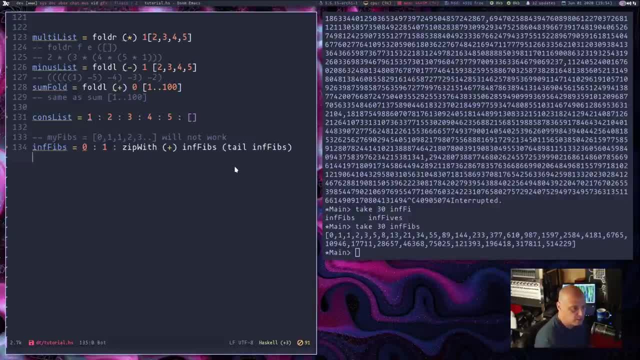 It's kind of how that works again. I will let you guys Study that a little more. Really neat Haskell one liner. there is one to share with your friends, So let's play around with creating some more functions. This is a functional programing language. 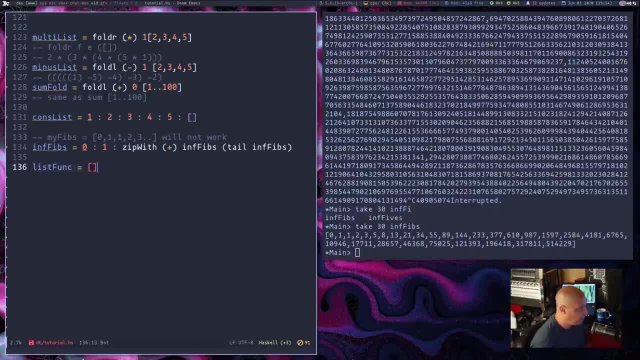 I'm going to call this list funk And what I'm going to do is, inside parentheses, we're going to do a X times Y and I'm going to do a pipe symbol which basically says: for X times Y, the X value. 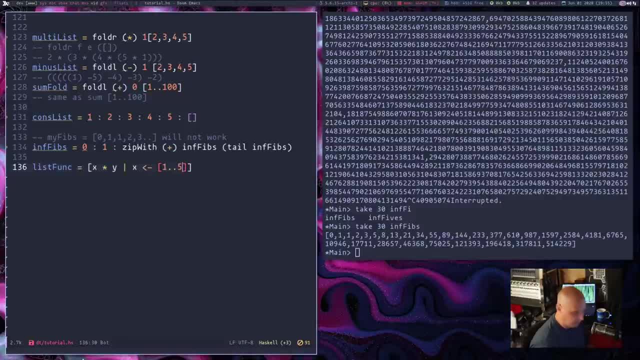 I want to pull that from this list one through five. I'll create a range, I'm going to do a comma And I'm basically going to say why we're going to pull that from a list. Why don't we do that also from a list one through five? 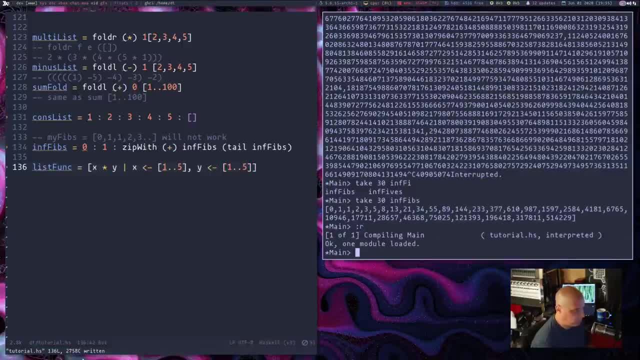 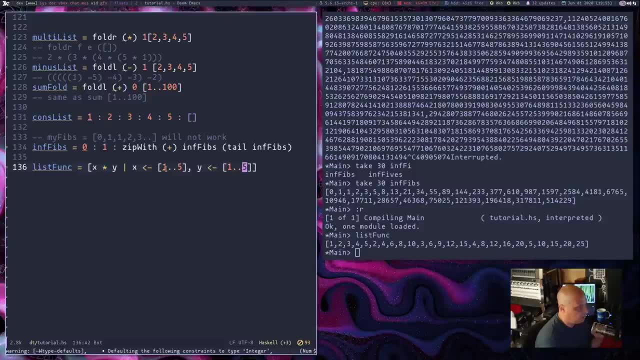 And if I write that and go back to the terminal and recompile, recompiles just fine. So let's see it in action List: funk. And what it does is it takes one through five and times that by one through five. So one times one, one times two, one times three. 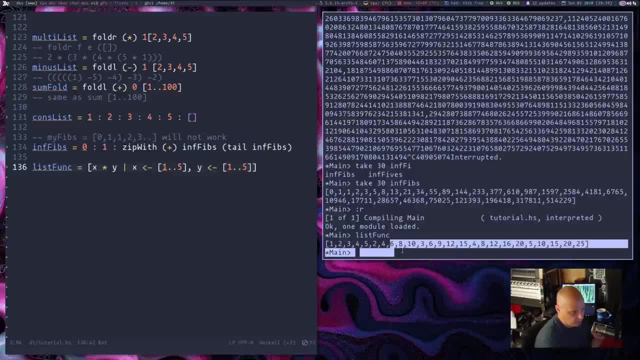 One times, for, one times five, Two times one, Two, Three, four, five, and then it takes three times one, two, three, four, five, four times one, two, three, four, five, etc. etc. Now I'm going to copy that function and let's create a new function list, func, and I'll do. 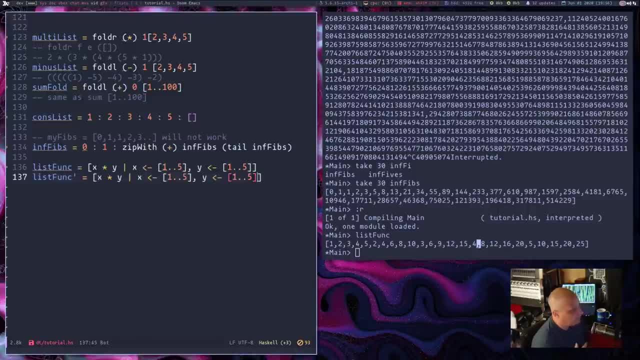 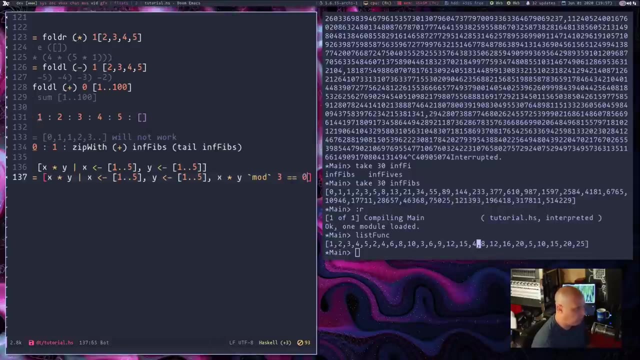 the single quotes because I just want to do a minor modification. So let's do x times y, where x is pulled from a list one through five and y is pulled from a list one through five, and where x times y, and we'll take the modulus of three equals zero. So we're basically taking the same thing. we 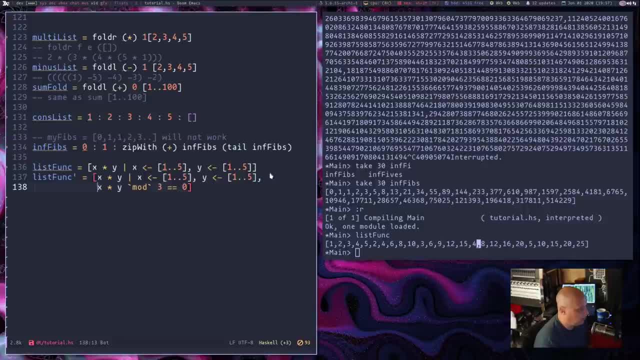 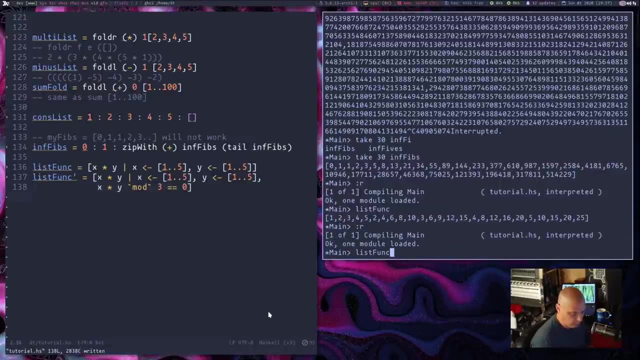 did before, except this time, and let me do a line break here so you can read it This time: the results, the only ones we want, are the ones where, when we divide the result by three, the modulus is zero. So let me write: get back into the terminal recompile and I will do: list func- single quote. 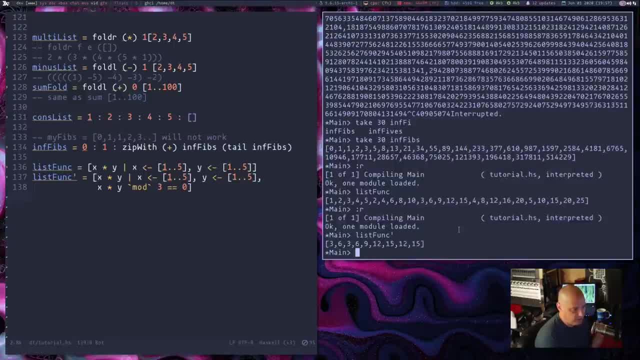 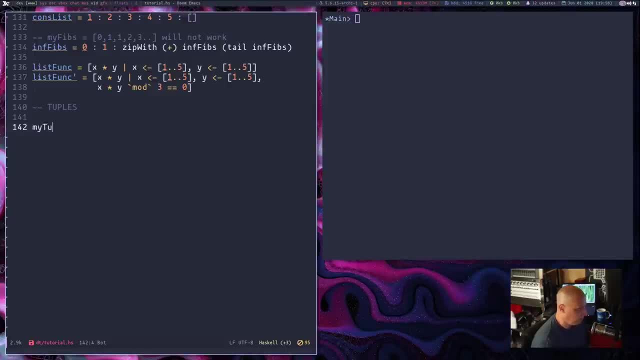 and it takes that list from before, basically, but it only returns the ones where it's divisible by three. and let's talk briefly about tuples. So I'm going to create a tuple here, I'm going to do my tuple equals, and then these need to be in parentheses and these are basically lists of items that are. 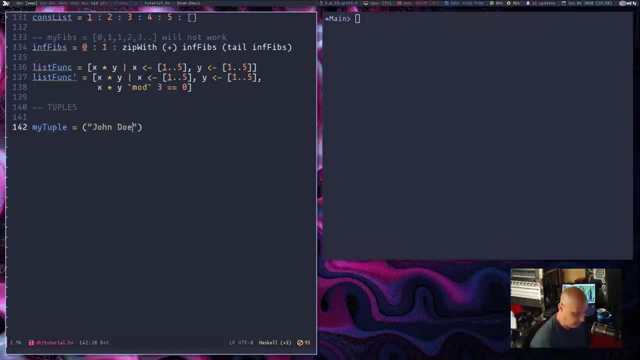 not alike. So for example, I could do a string- how about john doe? and then colon and then comma one. So basically we're going to do this tuple that contains names and numbers. We can pretend like the number is an id number. Maybe this is for business, right? I write that. 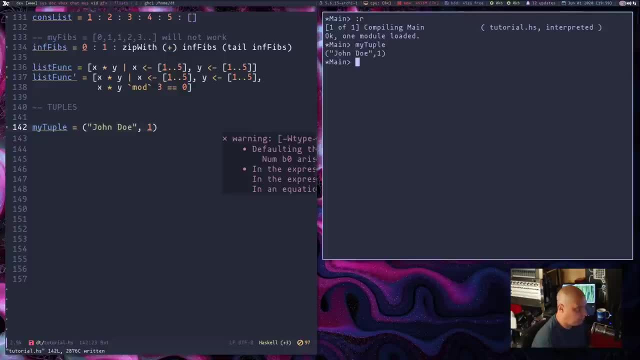 go to the terminal recompile and I do my tuple. Of course it just returns john doe and one. If I just wanted to pull the name out of the tuple, I could go get name and the command we want to run on it is fst for first, Basically saying, pull the first thing out of this tuple. The tuple is my tuple. 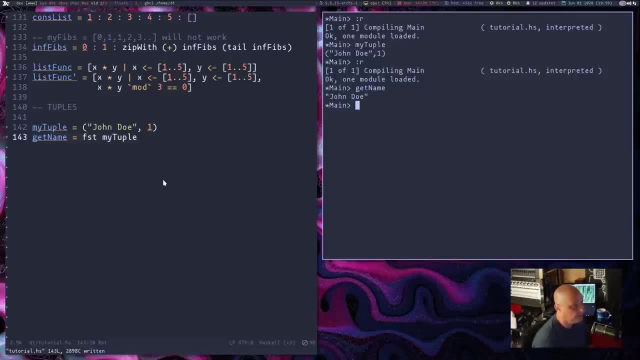 If I recompile and recompile, You see I get john doe, and I could do the same thing as far as getting the number. So I will do get id. We'll pretend like it's an id number and instead of first, let's do second: snd Write. 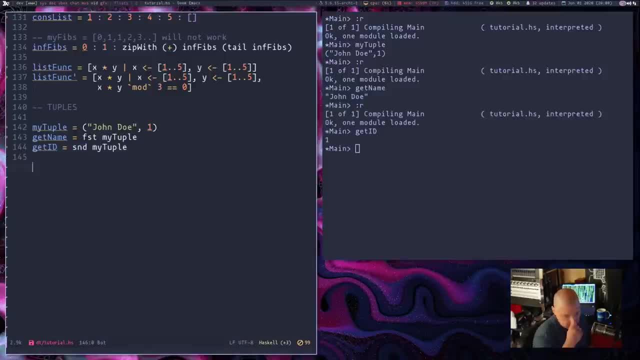 recompile and get id and it returns one. Now let's create a list of all of our employees names and a list of all our employees id numbers. I create this list of names: john doe, jane doe, mary jane and ben dover. 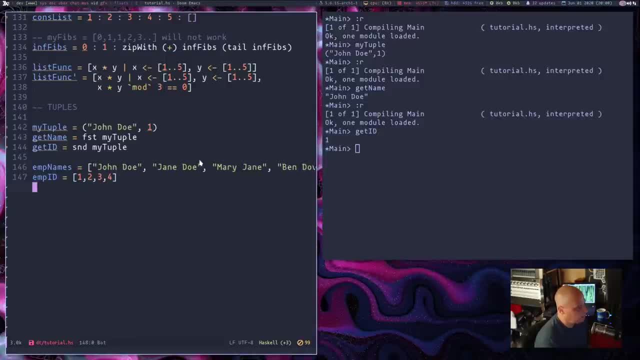 It's cut off here- And then employee id numbers, for each of these is one, two, three, four- And how we could create a tuple out of this. Basically, combine the two lists into a tuple is I'm going to create. I'll call it imp list and it's going to basically be a zip of imp names and imp id. 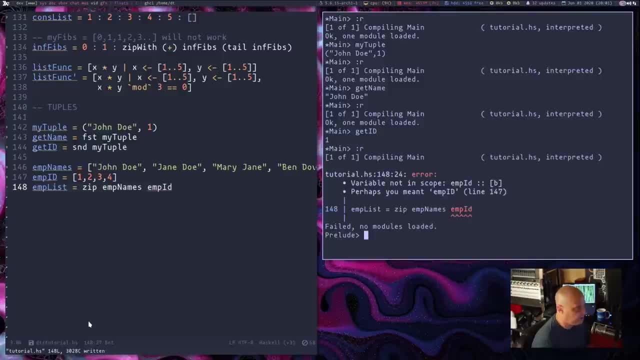 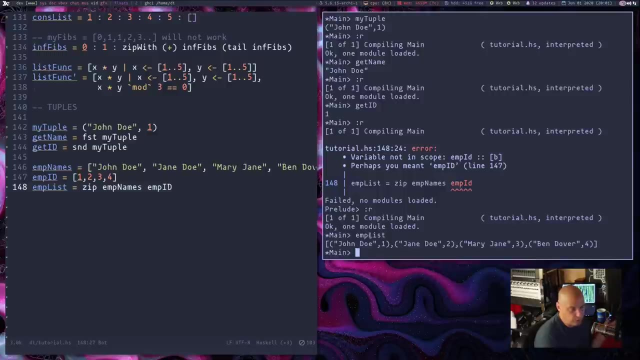 Let's write that. Let's recompile and ghci. I misspelled imp id because I had capitalized it. I'm going to capitalize both the i and the d when I created that variable. Let's reload It. compiles. just fine that time. And let's run imp list And you see, we get the tuple return, The new tuple. 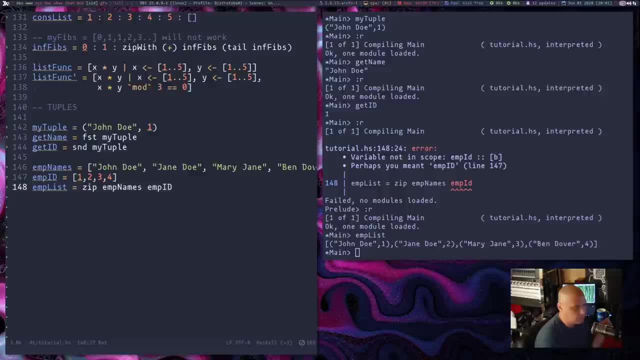 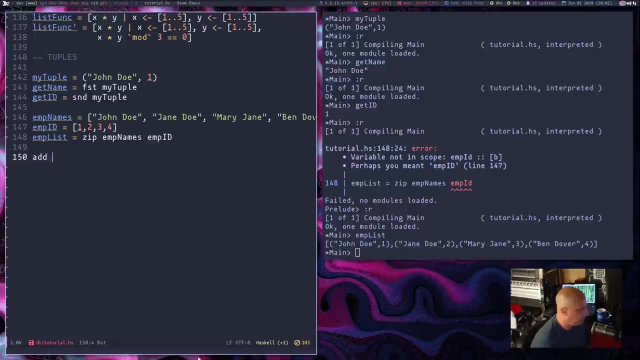 John doe one, jane doe two, mary jane three and ben dover four. Now I mentioned we could combine functions earlier. Well, let's see this in action. If I created this function- add a and b- So the function is going to be called add and then it's going to take two different values, a and b. 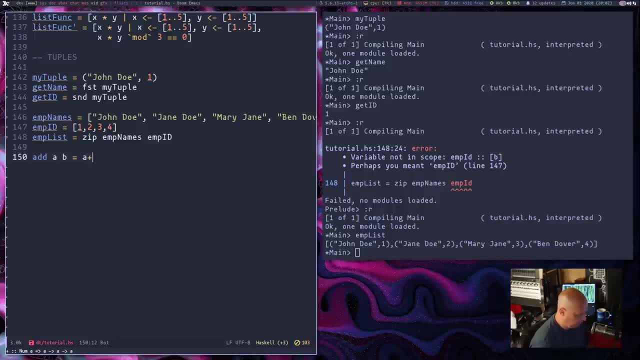 And it's going to equal a plus b. Pretty simple function, right, And we'll create another function. Let's call this multiply. It's not very original, but multiply, Let's do multiply. a and b equals a times b, And now that we've created those two very simple functions, we could combine those. 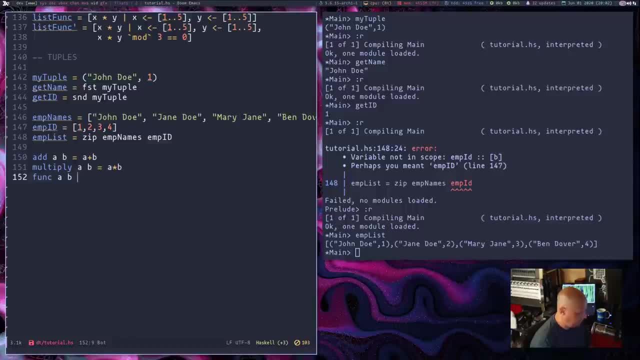 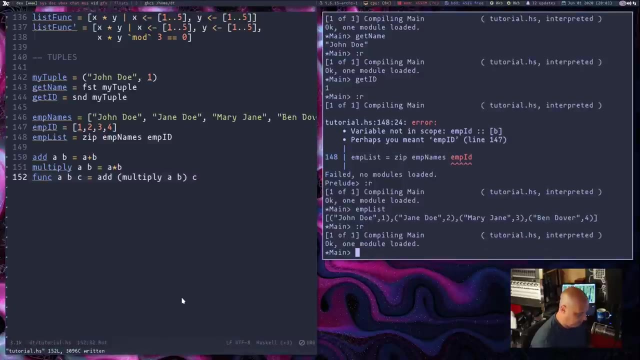 within another function. I could do func: a, b, c equals add and then in parentheses multiply a and b and then outside the parentheses c. You guys see what that's going to do. I'm going to write that and let's see if this compiles. See if I made any mistakes now And then if I run func. 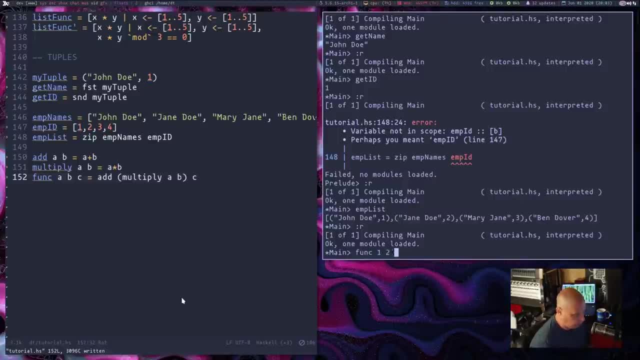 and then give it three numbers. I'll give it one, two and three. What it's going to do, it's going to multiply a and b. So it's going to multiply one and two first, which is two, And then it's going to. 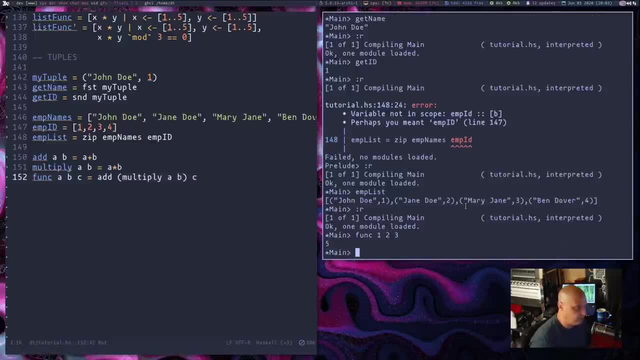 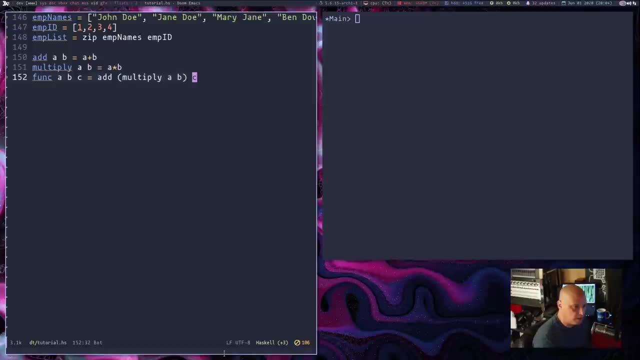 add two to c, which is three, So I should get five returned, And that's exactly what I get returned. I think the last thing we want to do is actually show you guys how to compile your tutorial dot hs, or whatever you named it, into an actual compiled 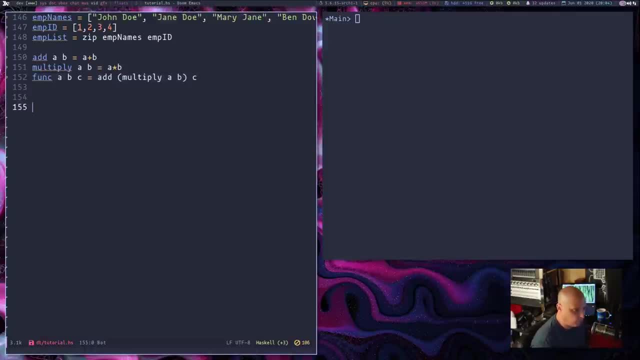 Haskell program and run that. It needs to have somewhere in it main equals. It's got to have a main function. What I'm going to do is I'm going to create this variable here. I'm going to say hello equals. Let's do your typical hello world. I'm going to do hello comma world. 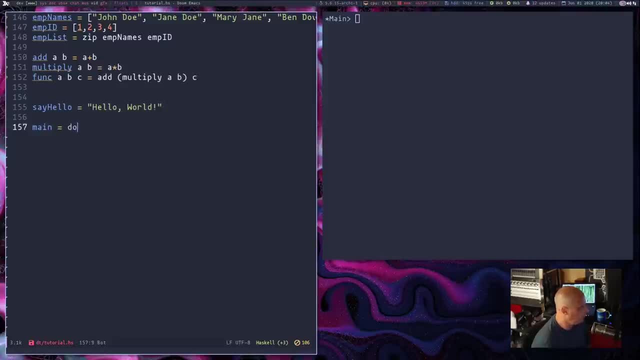 Exclamation point. And then on the next line, I'm going to do main equals do, And I'm going to hit enter And I'm going to print say hello, Let's write that. And if I go back to the GHCI and 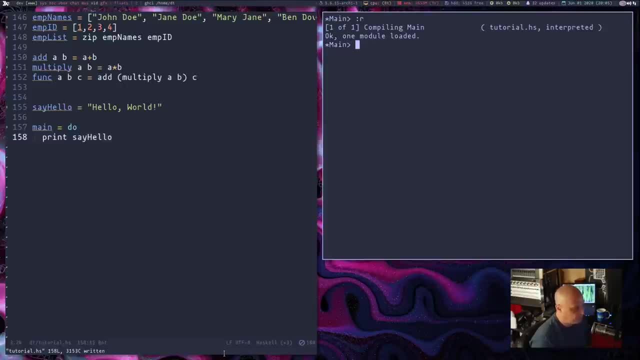 compile. If you actually compiled this into an actual program- Say you compiled your tutorial dot hs into an actual binary called tutorial- When you executed tutorial it's going to run the main And it's going to actually print out hello world. But here in GHCI I actually have to type main to. 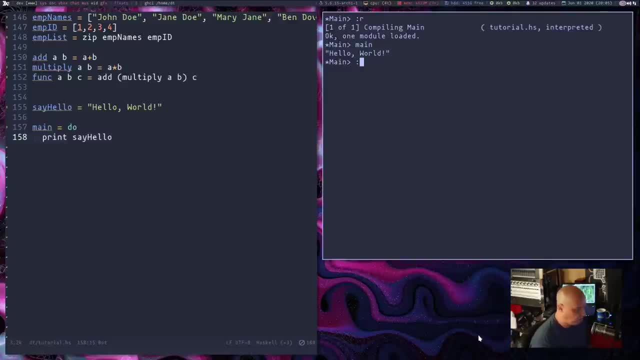 get this to work And it says: hello world. If you actually did want to see this compiled, I could do a colon q to get out of GHCI And to compile it you just need to do GHC, which is the Haskell compiler, And then what? 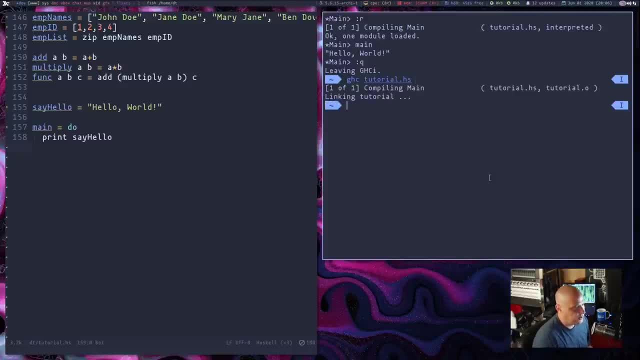 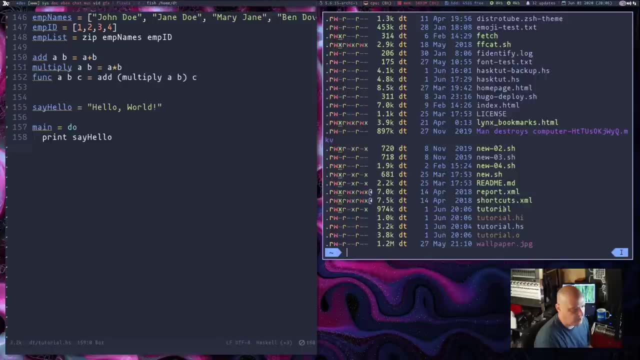 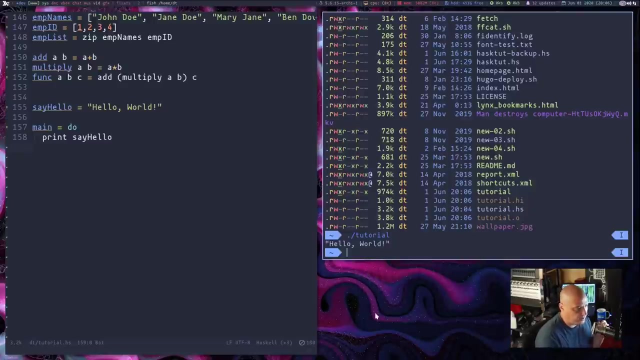 are we compiling? We're going to compile tutorial dot hs And you see, it just compiled it. If I do, it ls here in my home directory I still have the tutorial dot hs, But now I also have this executable binary called tutorial. I run tutorial. You see, I get printed out here in the command line. 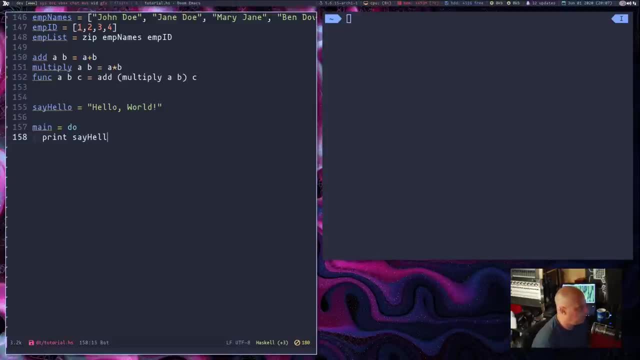 and I'm going to do hello world. Now, for most people, a simple hello world program, that's a little too simple. For your first program you may want to branch out a little bit. So instead I'm going to change main equals, do I'm going to do? put string line, So put capital s t, r, capital l? n, And then it's. 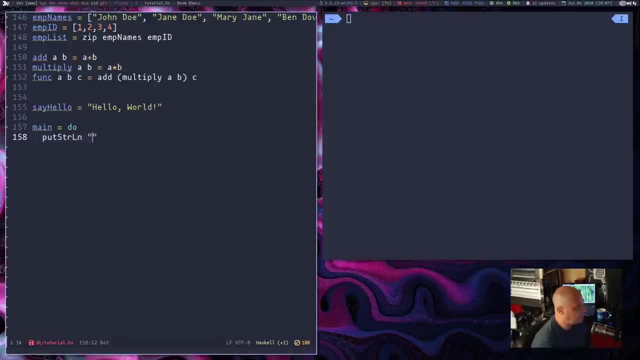 basically the same thing as printing a string here And then adding a new line after it And I'm going to put enter your name, colon space, And then on the next line I'm going to do name And then I'm going to do the less than sign and then a dash. It's basically saying I want you to get line and I 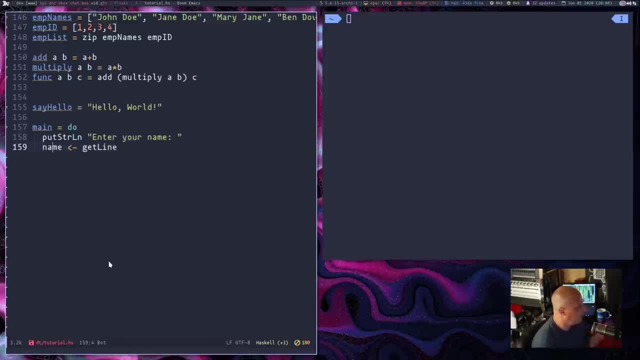 want you to send it to this variable here name. Now, what get line does? it takes whatever you enter into standard input And it's going to put that into this variable here name because we asked you to enter your name when you type your name. That's where get line realizes: OK, that's input. What am I? 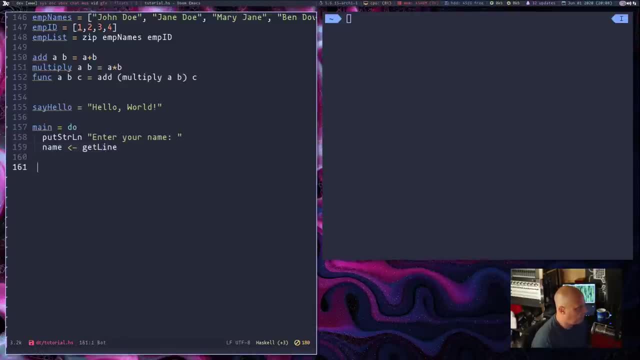 doing with that. I'm going to put it right here in name, And then the last thing we want to do is another Put string line, And then I'm going to wrap it in parentheses here, because we're going to do a few things here. I'm 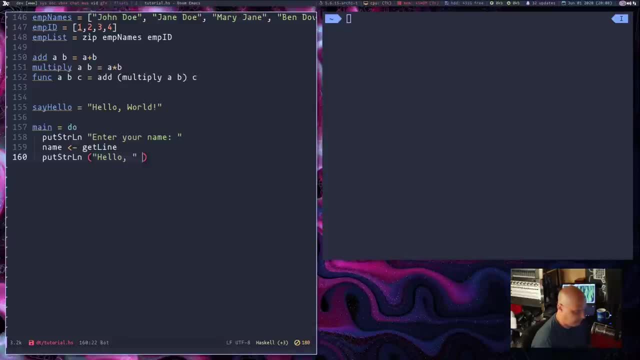 going to do a hello comma space and then outside the quotation marks I'm going to do space plus plus and then name from whatever you entered from get line, Put it in name, and then plus plus and then inside double quotes, an exclamation point. Let's write that. You know what we need to. 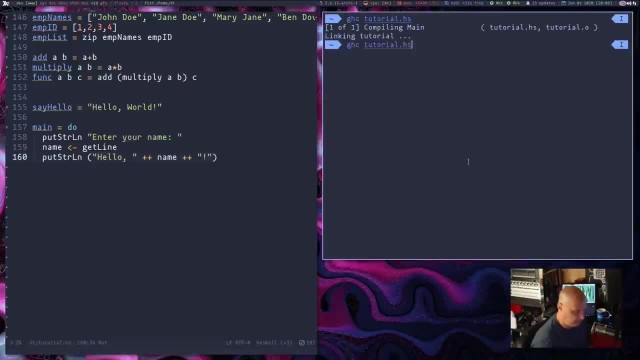 recompile, though. Let's recompile tutorial dot h s, and this time, when we were on tutorial, It asks: enter your name. So I'm going to enter my name, Derek, And it's going to take Derek, and it's going to return hello comma and then my name that I entered, Derek, plus the exclamation at the end. 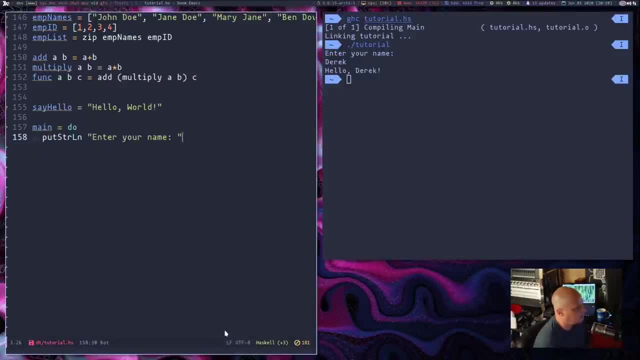 And just one more example of a good starter program. I'm going to basically just delete all the main and let's create a new function. I'm going to call it non uppercase and we should type it. It's basically going to take a string. Remember, a string is a list of characters. 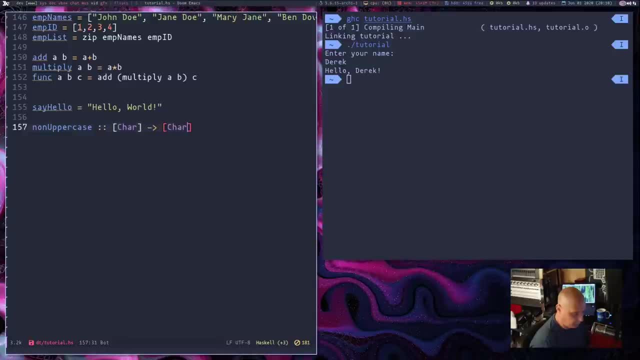 And what it's going to return. Well, it should return another string Again, another list of characters. Now that we've got that typed, Let's go ahead and do a non uppercase and then space, and then some value. I'll just call this s equals, And then what we're going to do is see the pipe. 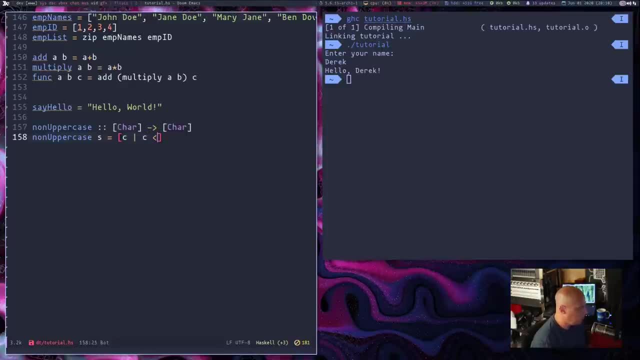 symbol. So it's going to take a character and it's going to pull this character from s, whatever it is. we enter as s. S is a string, by the way, So I'm going to do an s for a string. Let's see for a character here. Let's run e l e m for is it an element of? So is the character an. 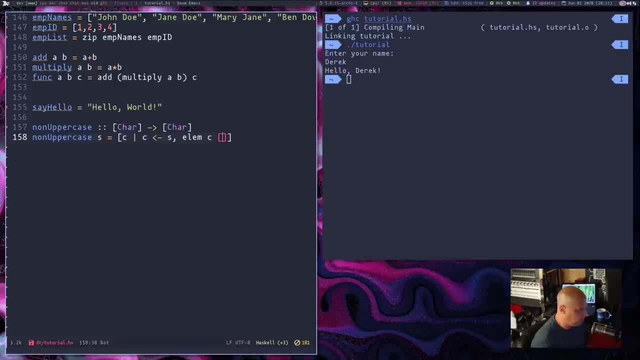 element of, And let's just do the whole alphabet. I think that makes sense. So I'm going to do, of course, a in single quotes, because a character has to be in single quotes, and then z. So you guys see what this is going to do: Non uppercase. and then on s, which will be a string, I'll pass a string. 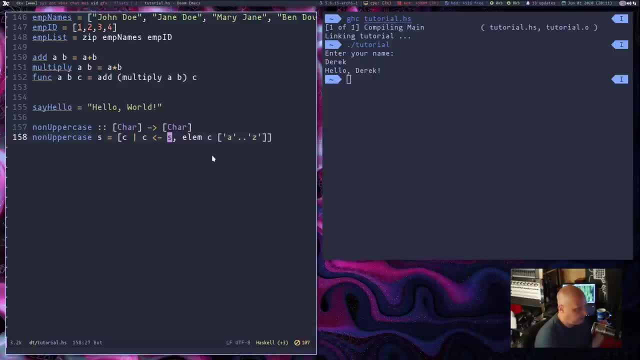 along to it. I'm going to take a character from the string and it's going to see if it belongs to a through z, the alphabet. And you're going to think, well, of course everything belongs a through z, But remember, this is just lowercase a through z. That's why I called it. 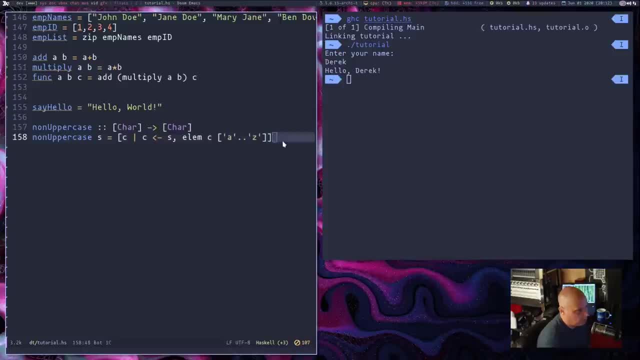 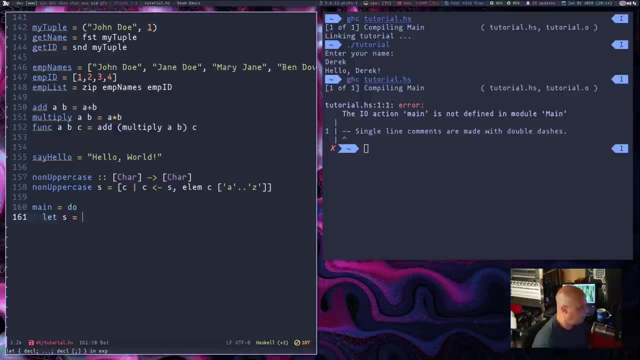 non uppercase. Any capital letters obviously are going to have a problem here. Let's do our main equals do. And then on the next line, I'm going to say let s, which is our string, And we're going to run our function from earlier that we created non uppercase. I'm going to run non uppercase on this. 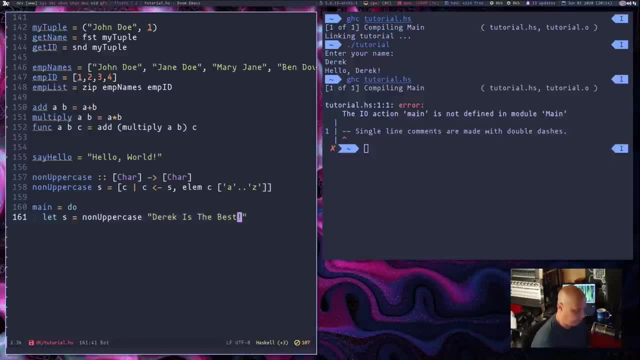 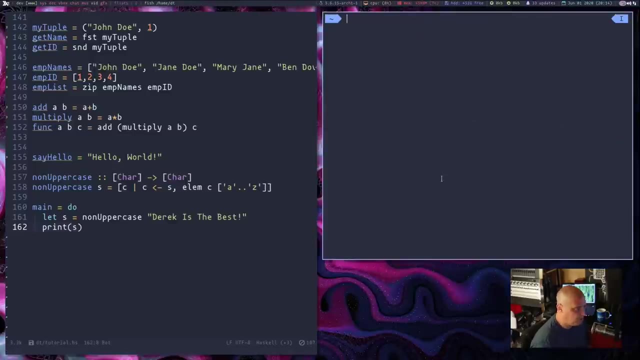 one, Derek is the best exclamation point. And then on the next line, I'm simply going to do a print s. So we're going to print that string, But it should pull out all the uppercase characters, because they are not an element of the a through z list, because it's all lowercase. Let me get into. 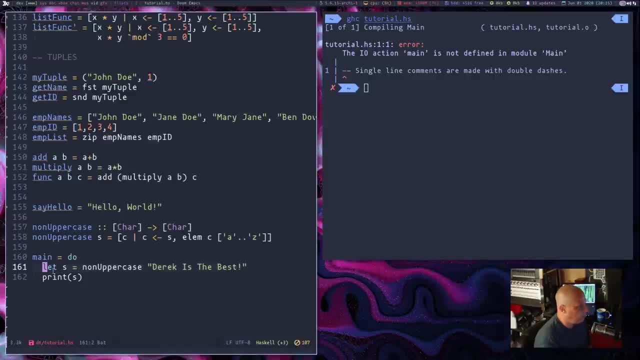 the terminal here I'm going to recompile. You know, what I think it's complaining about is my spacing. I just went with the spacing that Emacs kind of suggested. But these two lines after main equals do need to be changed. So I'm going to do a print s And then on the next line I'm simply going to. 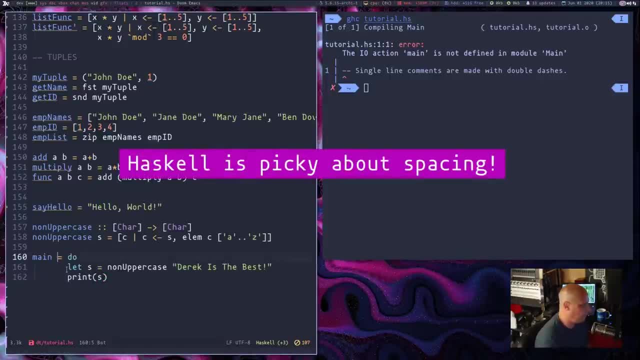 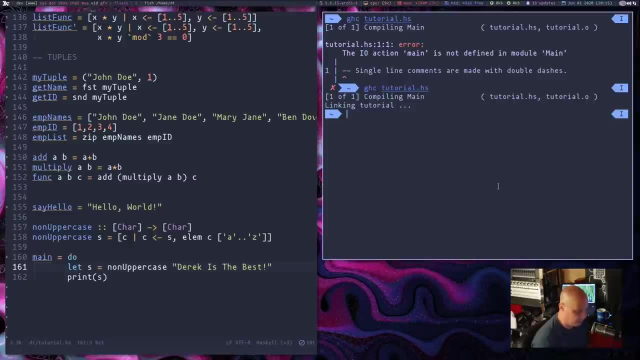 be on the other side of the equals sign. If I let them be over here, it was going to cause some errors. So now let me save that and see if it compiles correctly. And of course it does. And now let's run tutorial. And I don't know what that's supposed to be, But it took out everything. 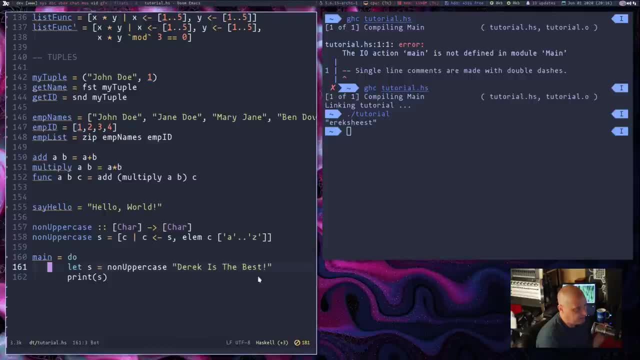 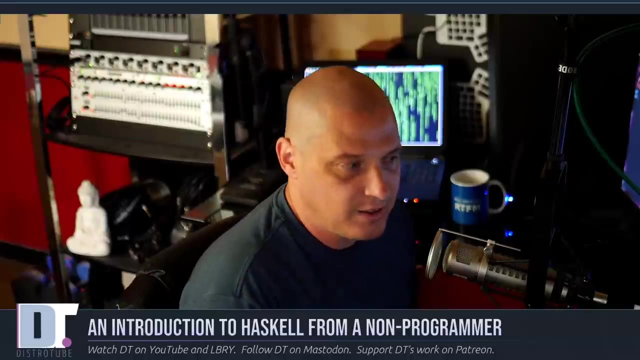 that wasn't a lowercase a through z, So the capital D, I, T and B are all gone. Also the blank spaces, the empty spaces are gone, And the exclamation point also didn't make it. So I think that's a good stopping point for this introduction to Haskell from me, the non-programmer. I just know. 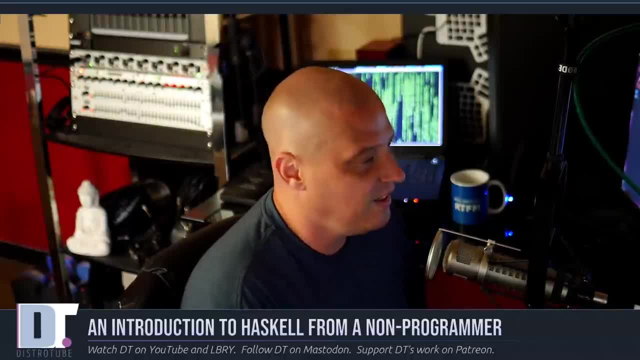 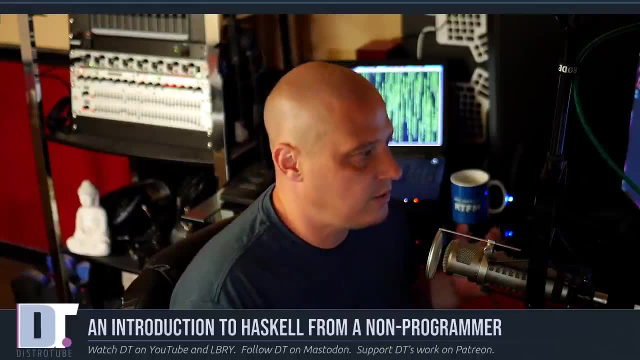 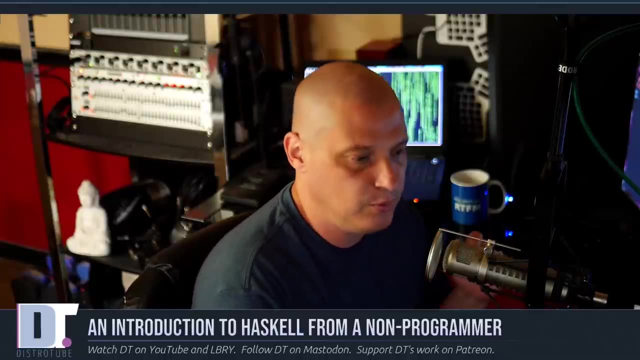 enough Haskell to hack on my Exmonad config a little bit, And today this really was very basic basic math functions, how to work with lists and tuples and a little bit about you know how the data types work with Haskell. I hope you guys found this stuff useful. If you'd like me to, 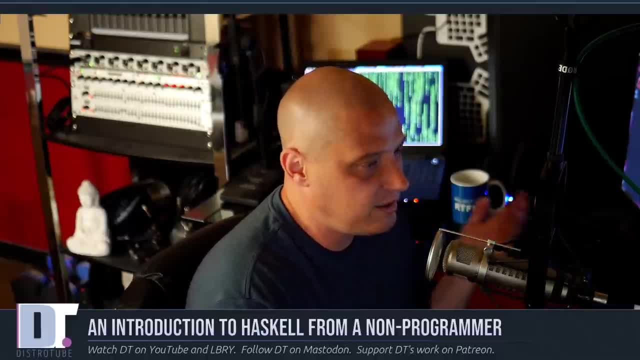 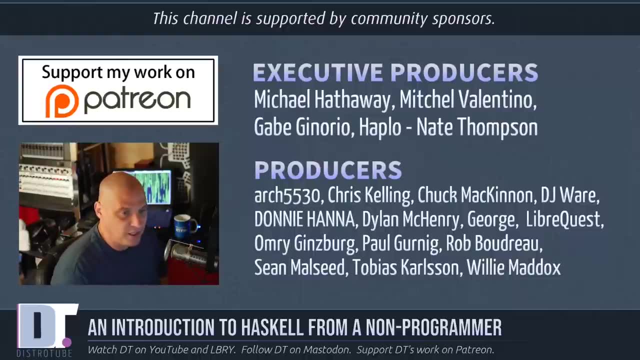 do more stuff involving Haskell in the future, I certainly don't mind. I'm going to do a little bit. I find Haskell interesting. I actually like working with Haskell. Before I go, I need to thank a few special people. I need to thank the producers of the show: Michael Mitchell, Gabe. 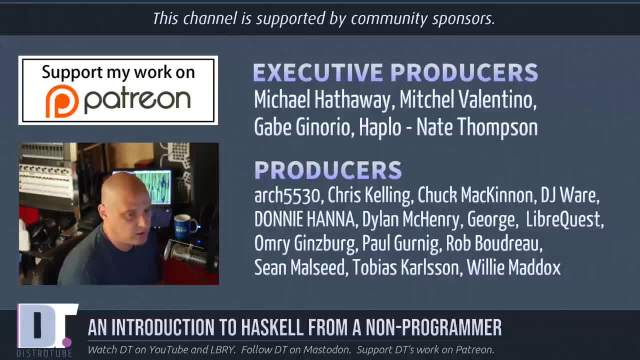 Haplo Nate Arch5530,. Chris, Chuck, DJ, Donnie, Dylan, George, Haplo LibraCuts: Omri, Paul, Rob, Sean, Tobias and Willie. They are the producers of the show. They're my highest tiered patrons. 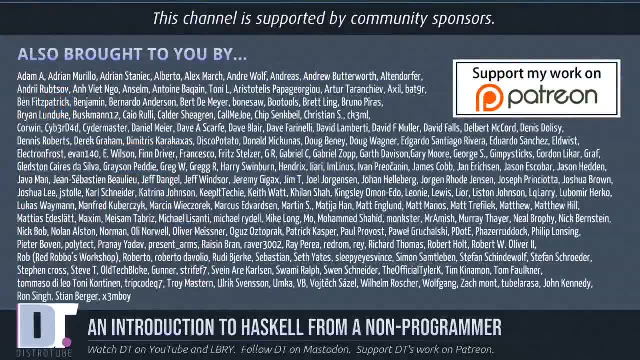 over on Patreon. The show is also supported by all of these ladies and gentlemen. These are all my supporters over on Patreon, each and every one of these ladies and gentlemen. I want to thank those guys. If you guys would like to support my work, consider doing so. You'll find DistroTube over on. Patreon: All right guys, Peace. 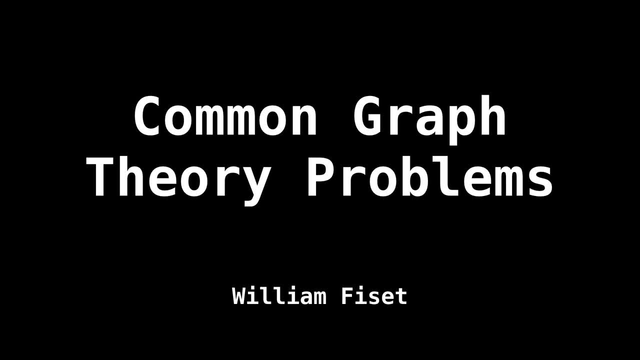 Hello and welcome back. My name is William And today I'm going to talk about common problems in graph theory. A lot of problems you will encounter can often be reduced to a famous or well known problem, or some variant thereof, So it's important to be able to familiarize ourselves. 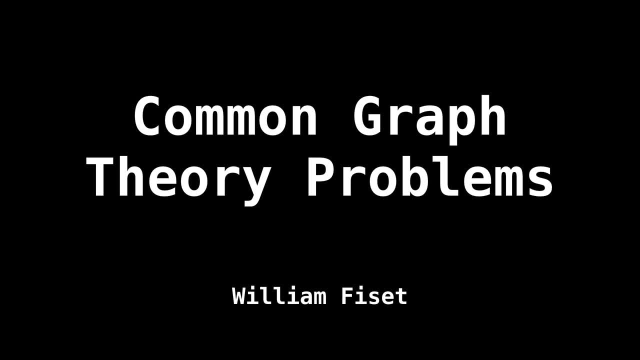 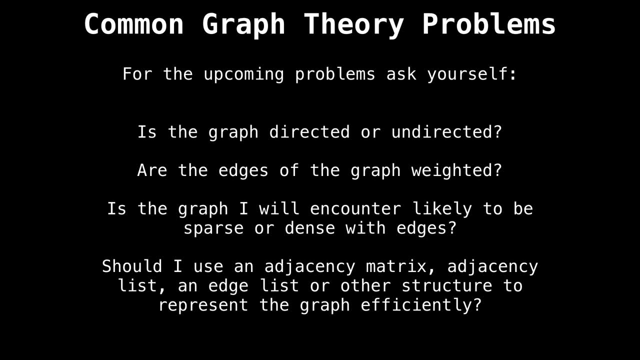 with common graph theory problems and their solutions. Just before getting started, following off from what we learned in the last video about representing graphs, I want you to think about how you would store and represent the graphs and the upcoming problems I'm going to describe In particular. is the graph in the problem I'm describing directed or undirected?